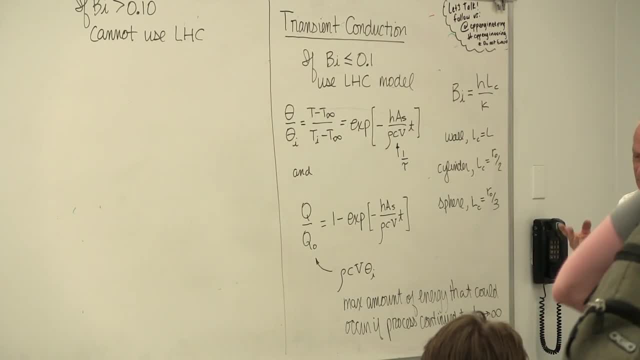 So if you use that model, and that model then says that the temperature in a body at any particular time is not a function of geometry, the spatial coordinate, The temperature is not a function of X or R, it's only a function of time. So we use that, we derive the little simple. 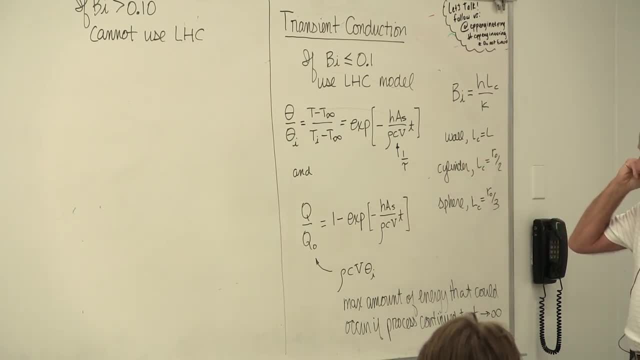 differential equation. we integrated it with the initial condition. we end up with this equation right here in your notes: Theta is T minus T. infinity. Theta I is initial temperature minus T. infinity Rho CV over. HAS was defined as something called the time constant units or seconds if it's in SI Rho CV over. 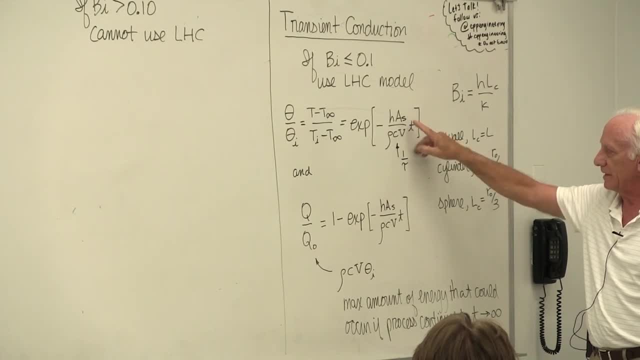 HAS, V is the volume, AS is the surface area. Very simple equation: Exponential decay function. Then you can integrate that with respect to time and find out how much energy has been transferred to or from that particular body. When you're done with that calculation you have Q over Q naught 1. 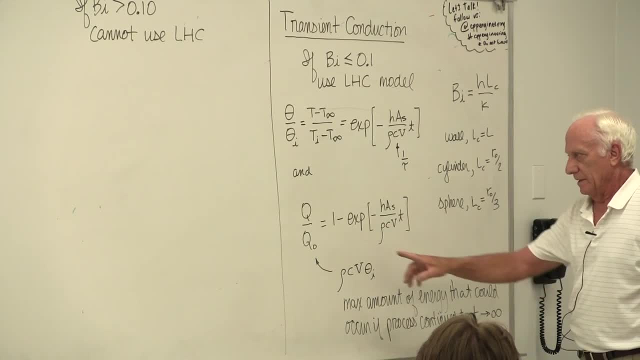 minus exponential, minus T over tau. This Q naught is rho, CV, theta I. Here's what it is: Rho times V, density times minus the mass. This is just mass C times change in temperature. What temperature? T initial minus T, infinity. So that term Q naught one way to interpret. it is the maximum. 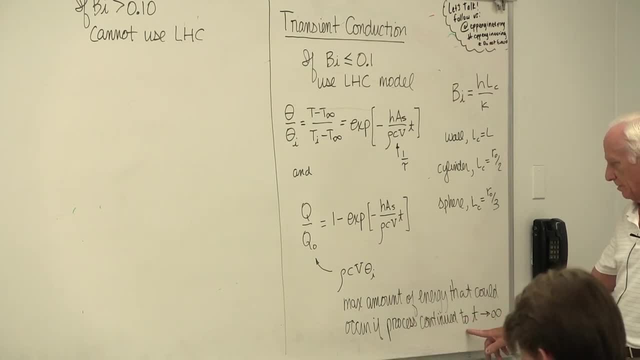 amount of energy that could occur if the process continued all the way out to T, approaching infinity: The maximum amount of energy. So it's a ratio: The actual amount of energy divided by the maximum amount of energy. All right, so there we are, for the simple model. 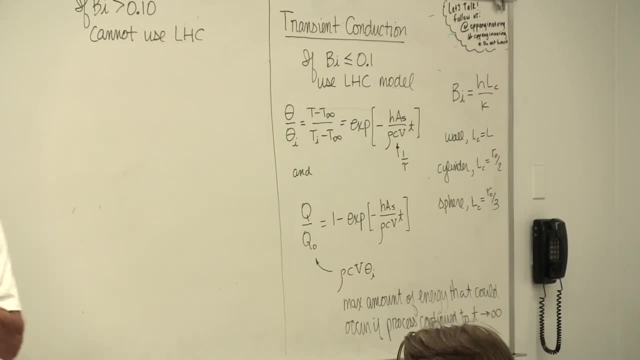 Now the next question is: what's the number of thermos that is less than or equal to T? Good question, We've got T. Let's go back and see what the number is. So let's take a look at that. 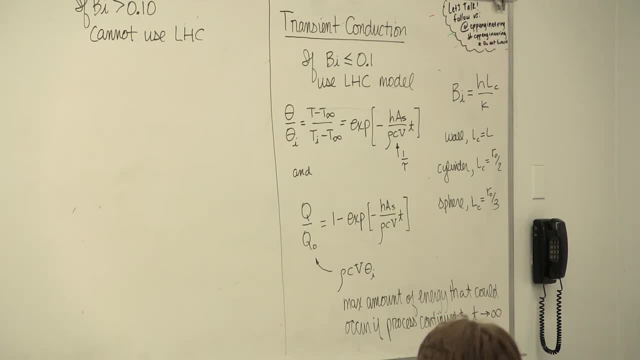 So that's the number. So it says we're going to run this over the temperature and we have a lumped heat capacity. Of course, the next question is whether a number comes out to be greater than 1 T. We can't use that anymore, So now we have to go back to chapter 2 and start from. 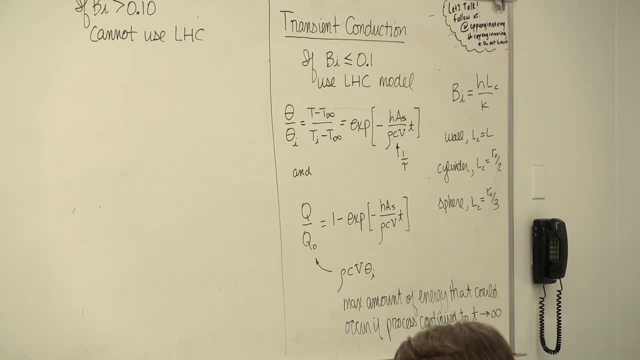 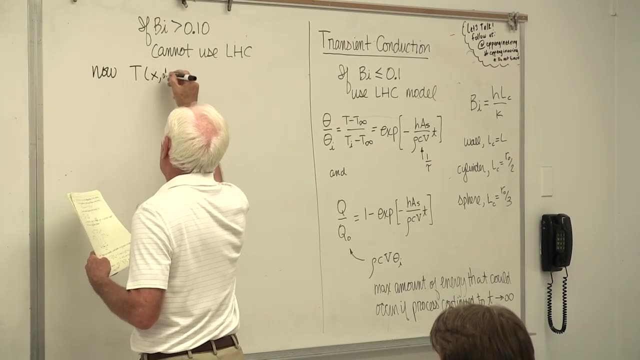 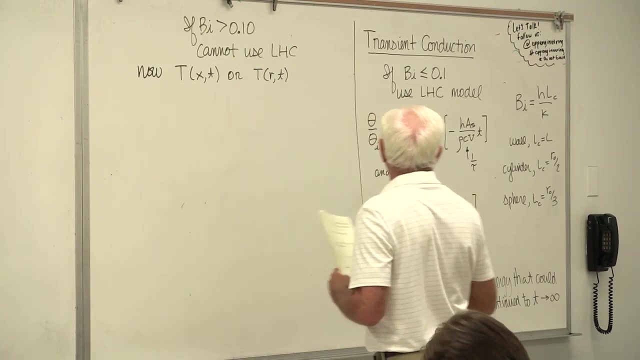 there. Now the temperature is going to be a function of X, So what does that give us over T? As a result, we have a function of X and a function of E and time, Or maybe radius and time if it's a long cylinder. 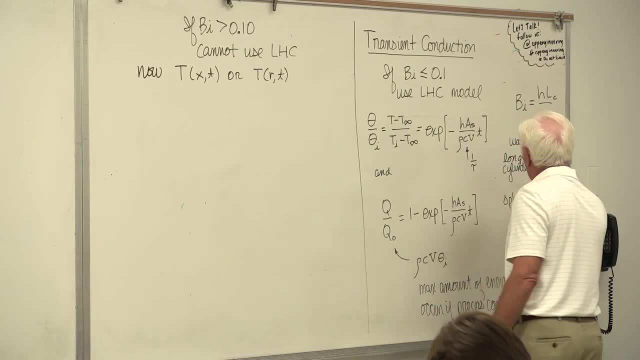 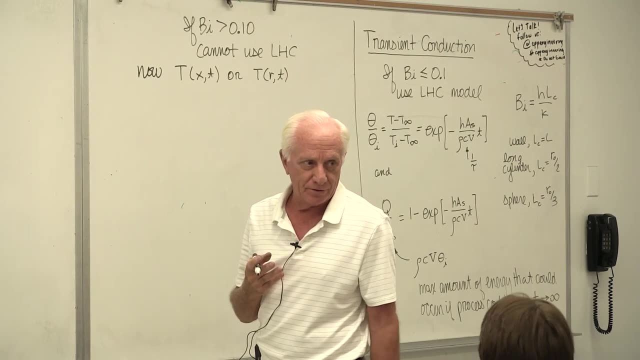 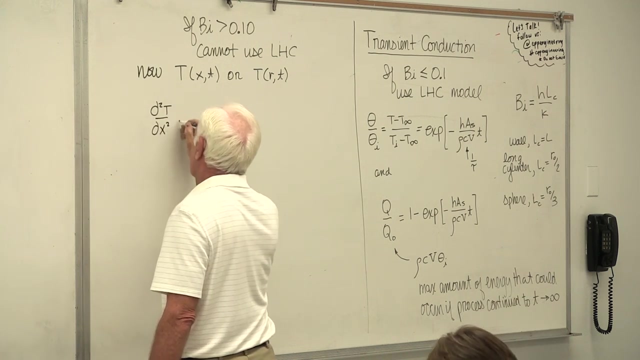 By the way, this is a long cylinder. A long cylinder or a sphere? Now we have to go back to the governing partial differential equation, chapter 2, which is the second partial of P with respect to x squared. This is for a wall. 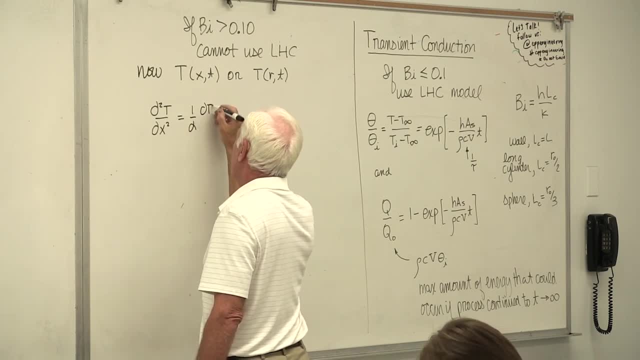 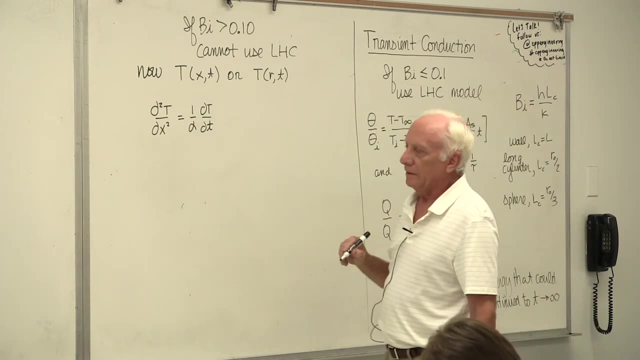 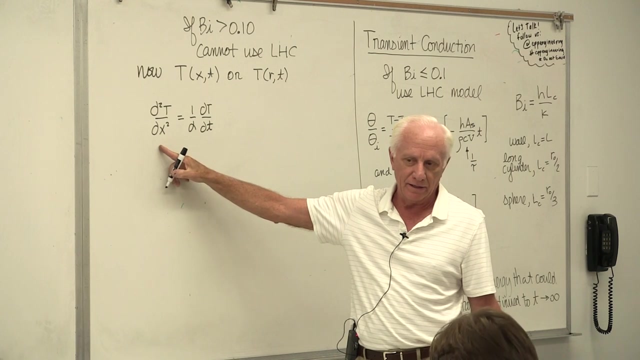 It's equal to 1 over alpha dT, d time In words. left hand side is the net conduction heat transfer that occurs in the x direction. The net conduction heat transfer in the x direction, The right hand side, is the time rate of change of. 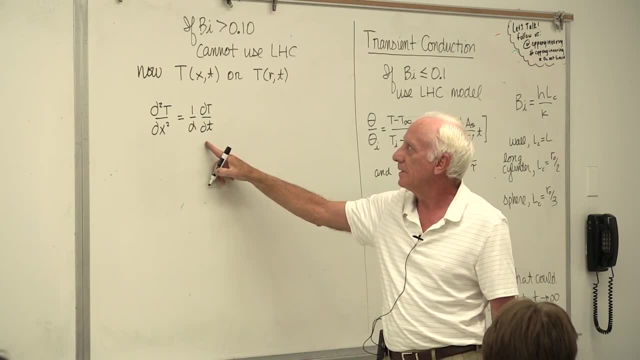 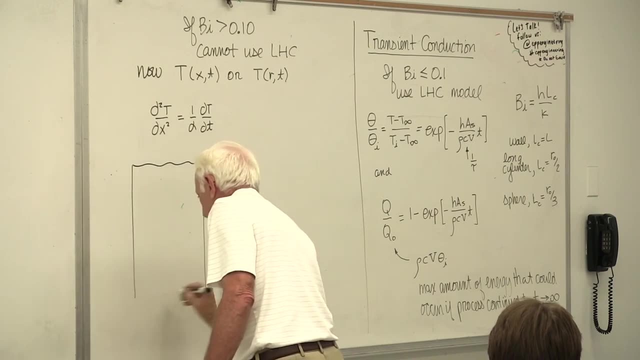 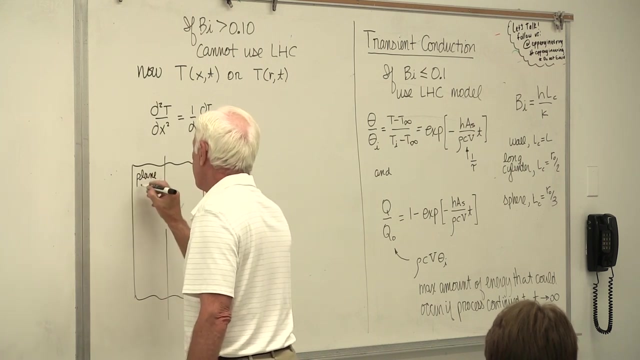 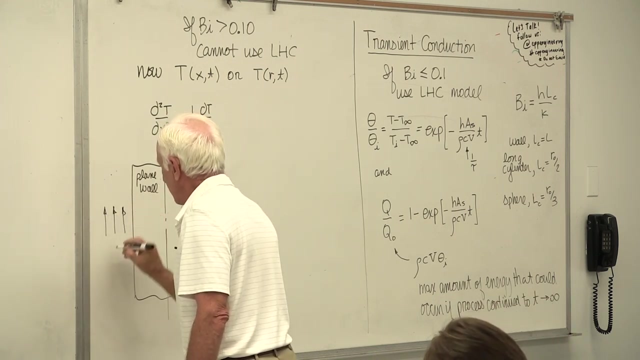 energy stored in the object. The picture that goes along with this- and we had it on the board last time, but I'll reproduce it here- Here's: this is a plane wall. There is a fluid blowing over the outside of the plane wall. 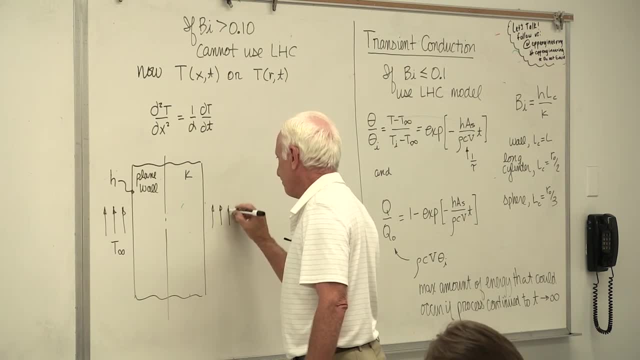 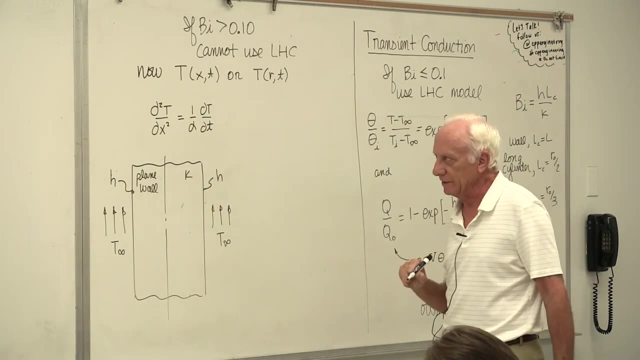 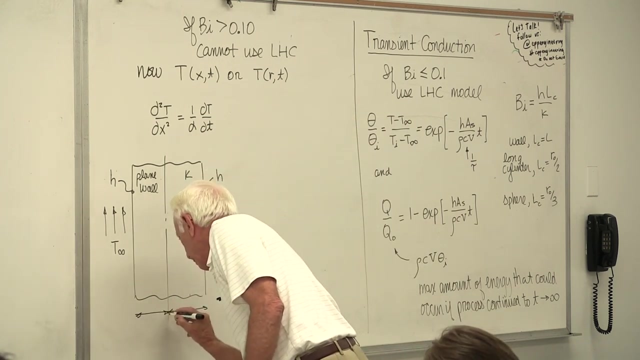 Temperature T. infinity Convection coefficient is H on both sides of the wall. It's symmetrical, the same conditions. The wall has a thickness of 2 times L. We measure x from the center of the wall, so the center of the wall is x equals 0.. 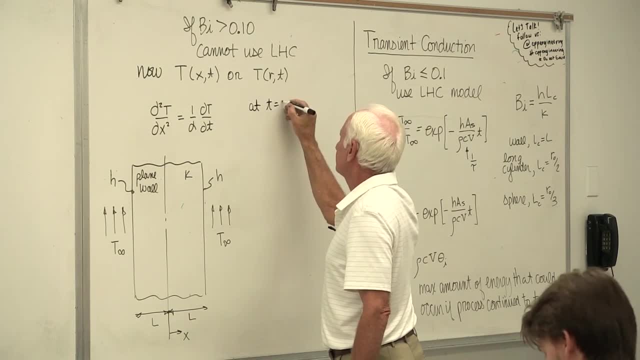 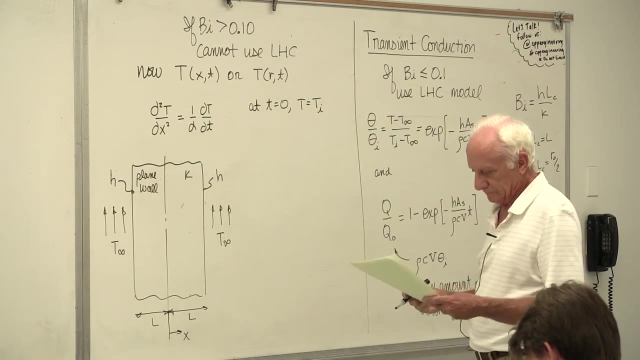 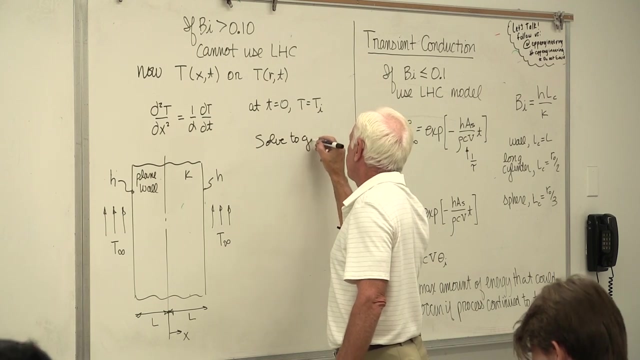 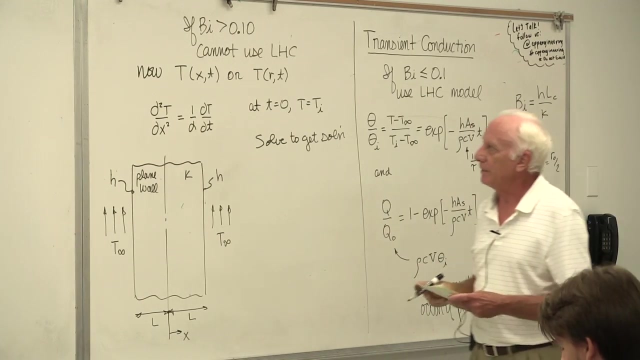 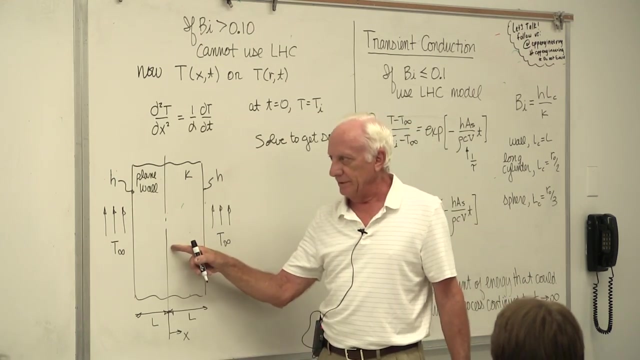 The initial condition, T i. We solve that partial difference equation with the initial condition and the boundary conditions. The boundary conditions are- let's take the easy one first At x equals 0,. dT dx is 0.. The slope of the temperature curve at the middle is 0.. 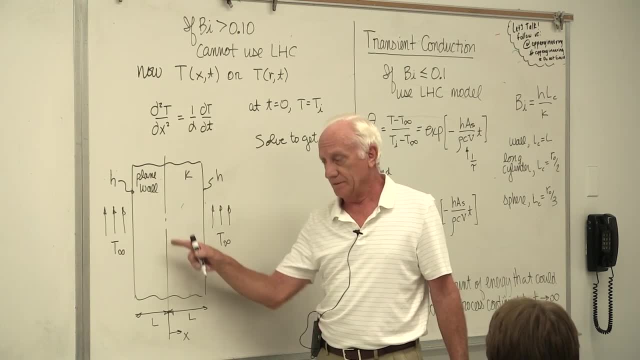 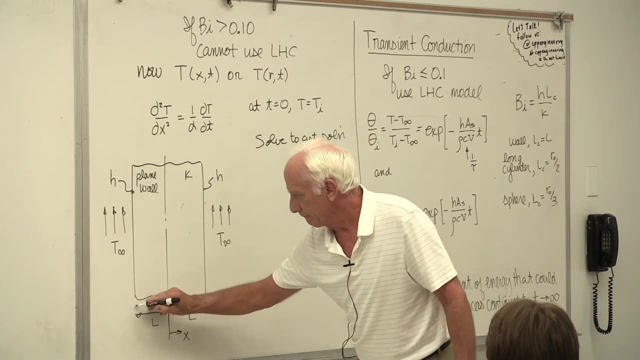 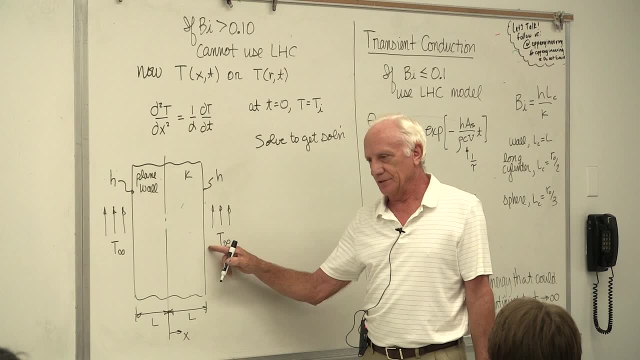 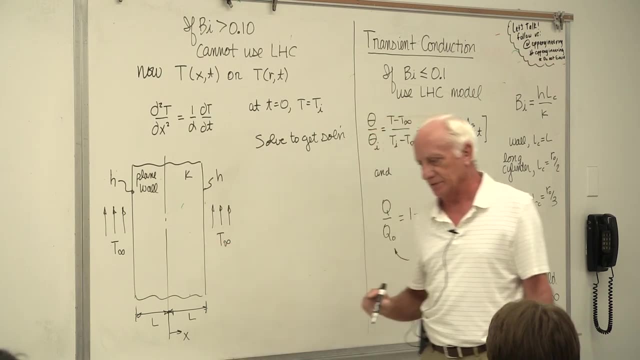 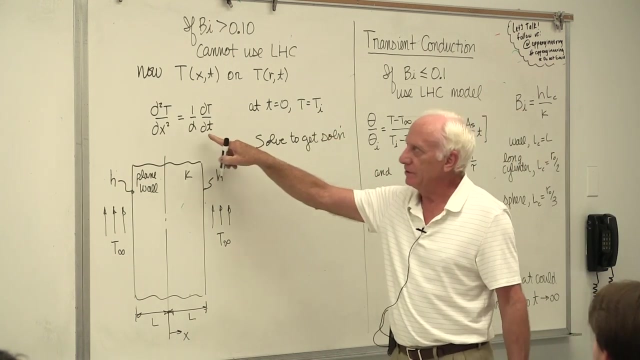 x equals L. conduction into the surface equals convection out of the surface. Conduction into the surface control volume equals convection out of the surface control volume. Chapter 1.. Okay, So you use this, one initial condition, two boundary conditions. 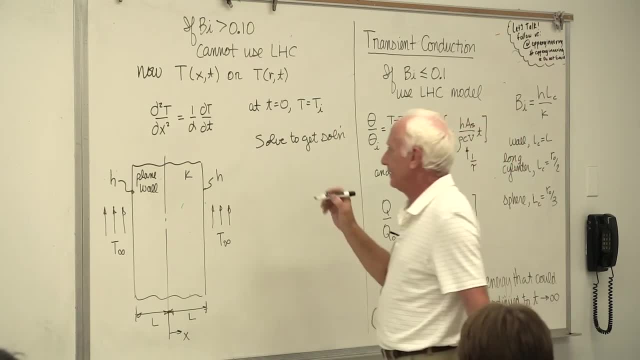 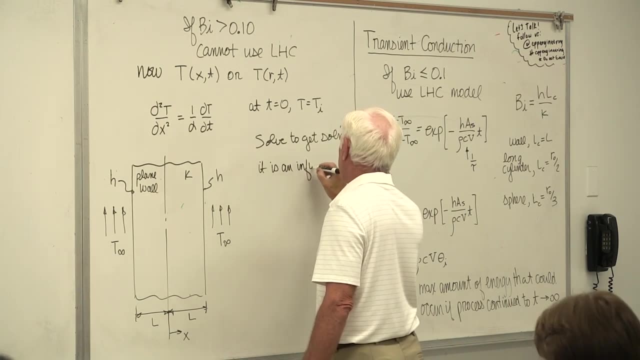 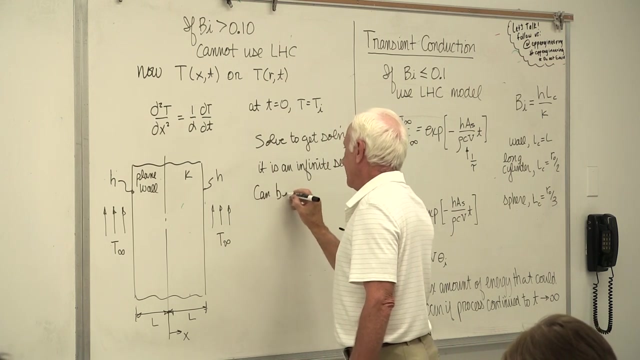 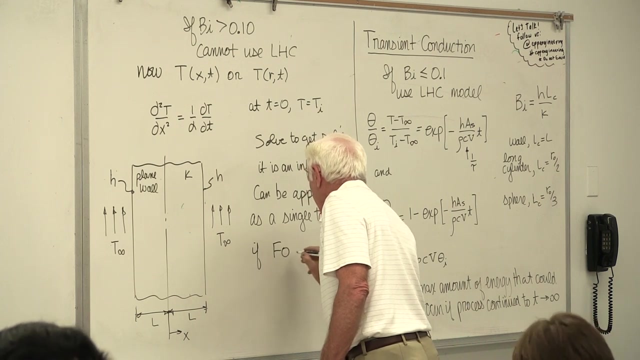 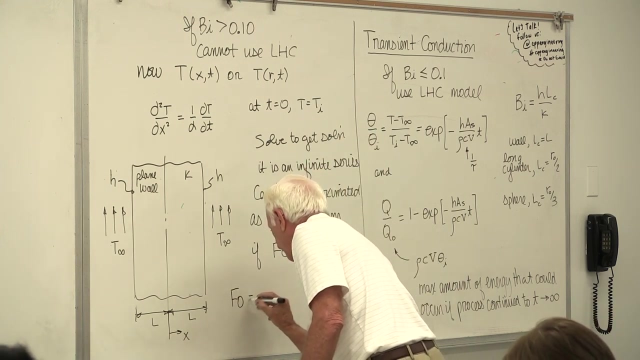 And you solve it and you get a pretty horrendous solution. now It's an infinite series. We can approximate that By the first term if something called a Fourier, Fourier number is greater than two-tenths. So a new dimensionless term. 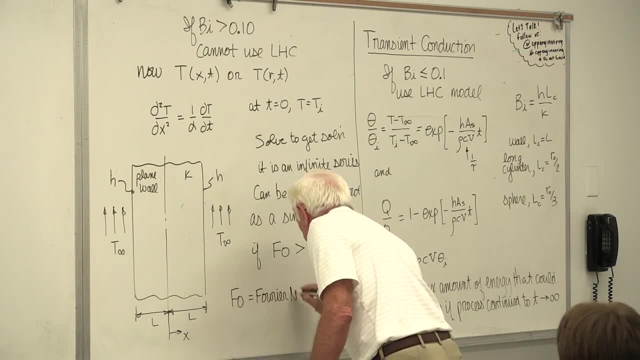 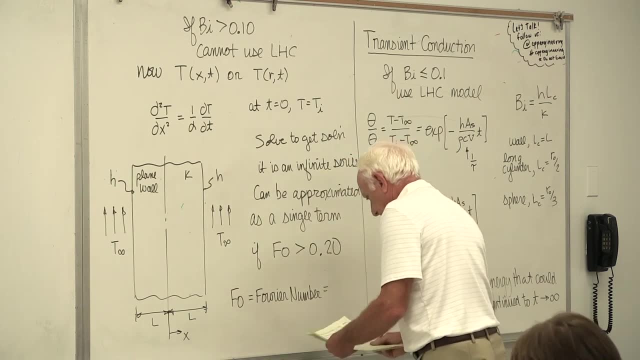 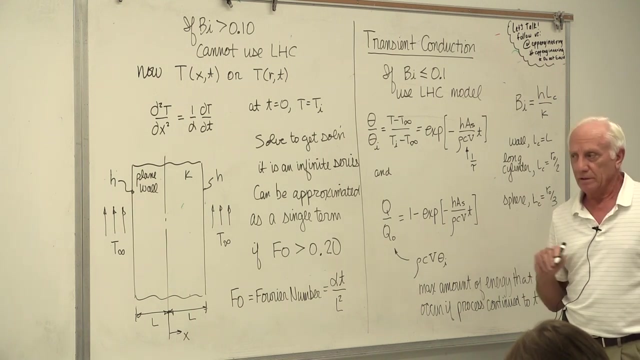 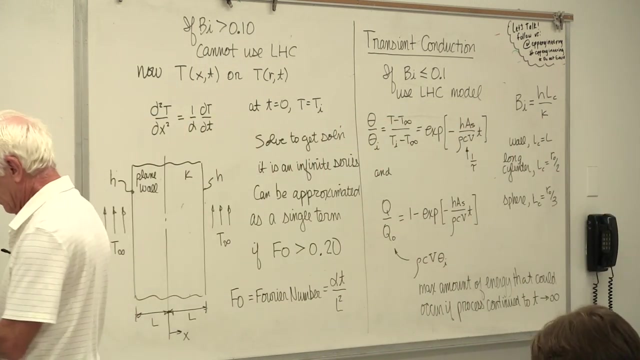 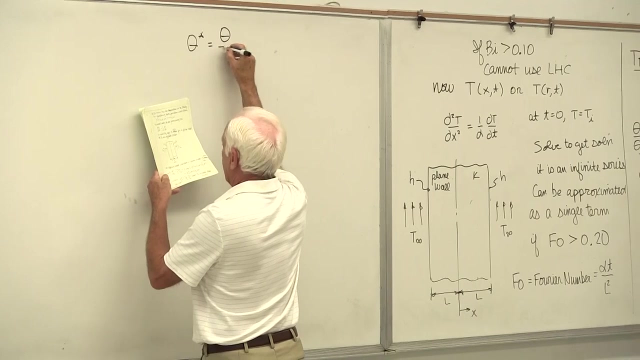 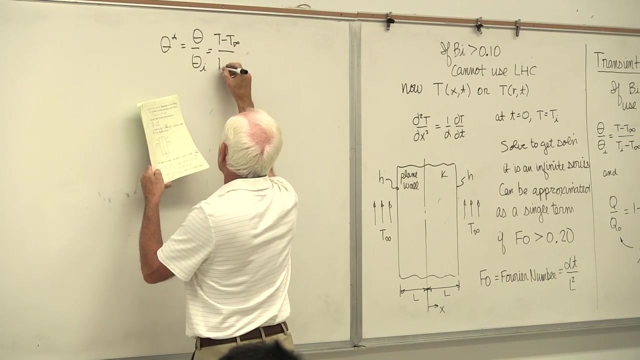 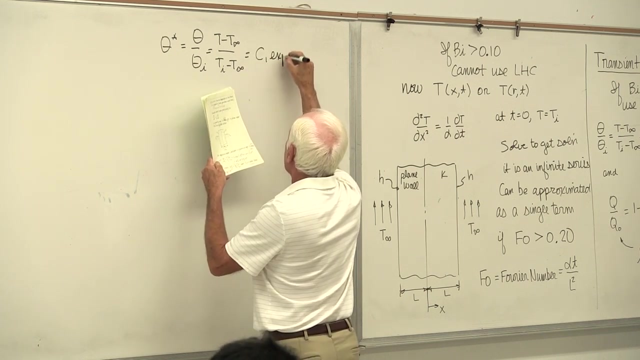 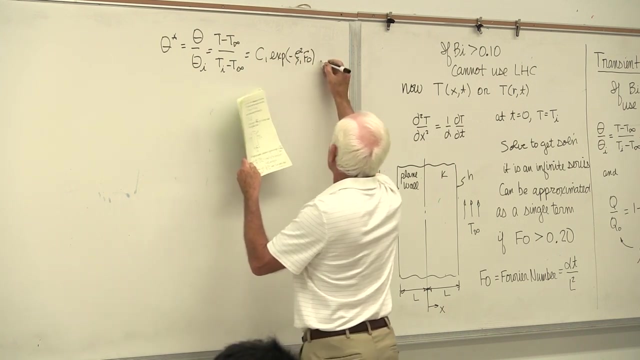 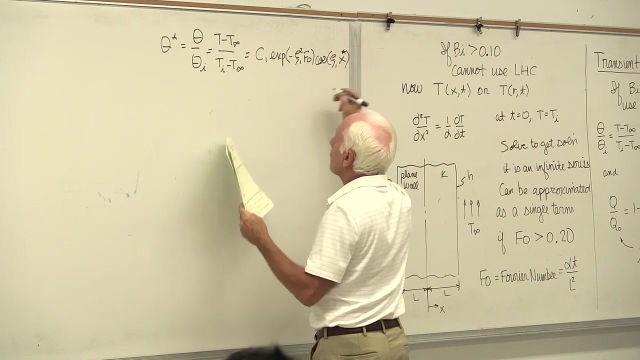 Fourier number And the Fourier alpha, T over L squared. Thermal diffusivity times the time in seconds divided by, for the wall, the half wall thickness squared. If you do that, the equation looks like this, And this is in the textbook: 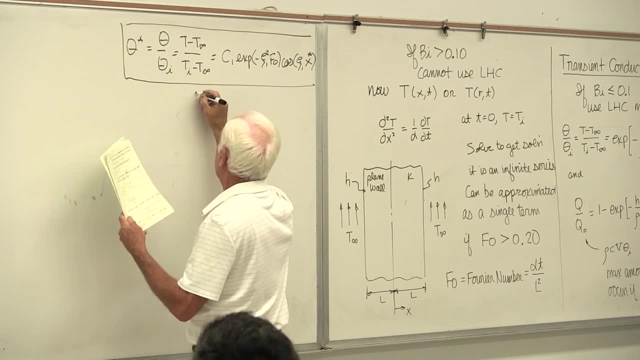 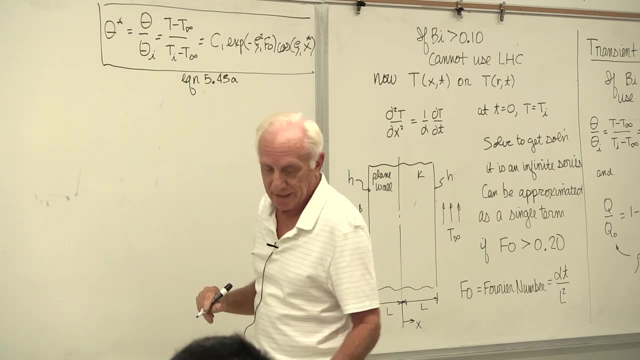 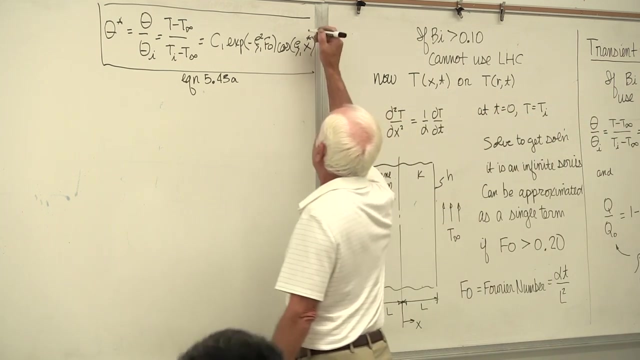 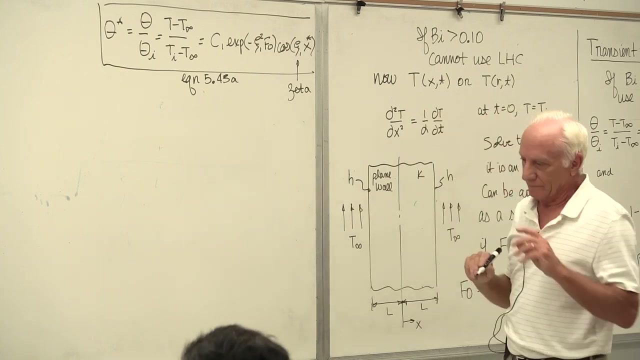 This is equation 543A. That's the first term of that infinite series That will give us a good temperature if the Fourier number is greater than 0.2.. Okay, This guy is zeta And okay, here it is. 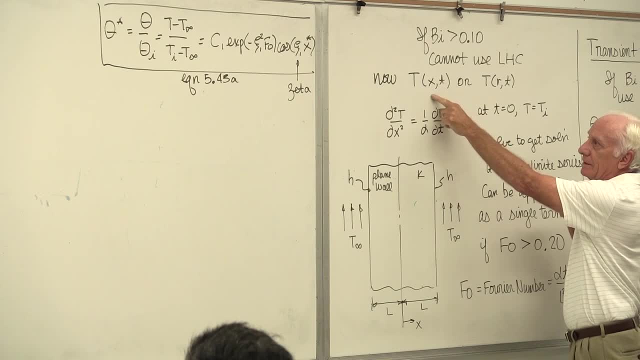 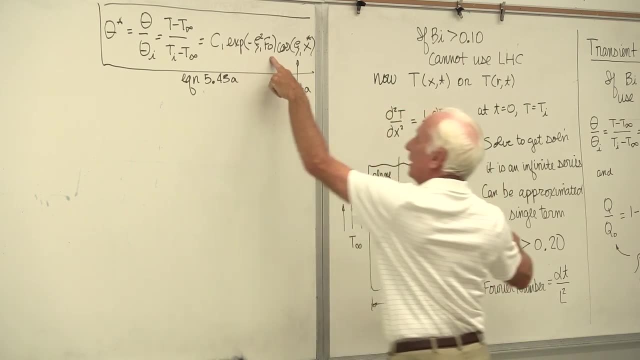 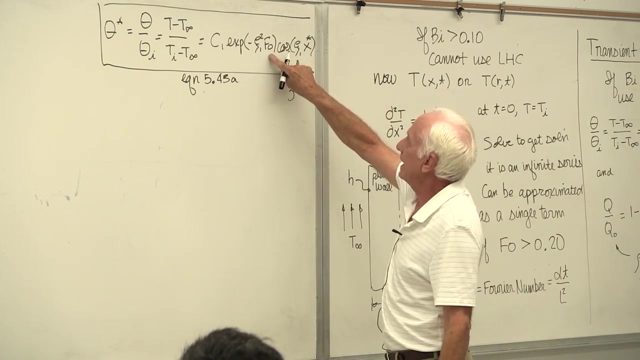 The temperature is a function of x and time. Where is time? Time is in the Fourier number. There's Fourier, There's Fourier. The time is in the Fourier number. Where is x In the cosine term x star? What is x star? 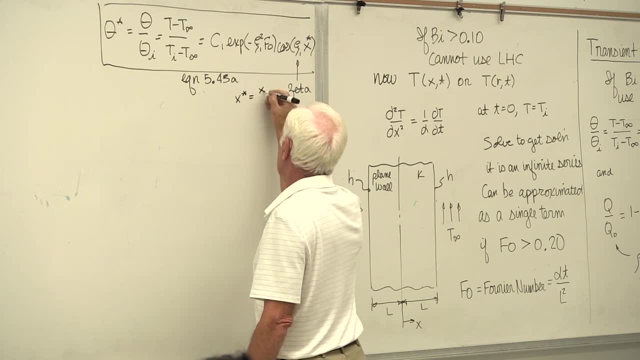 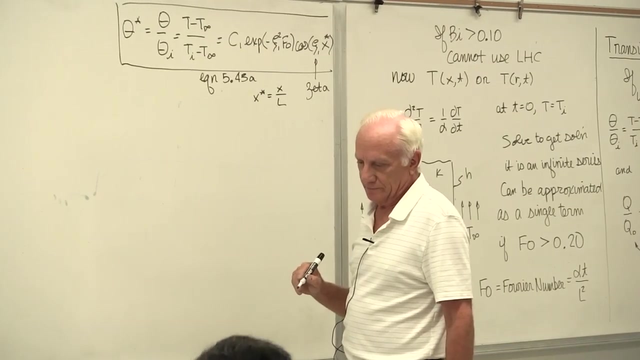 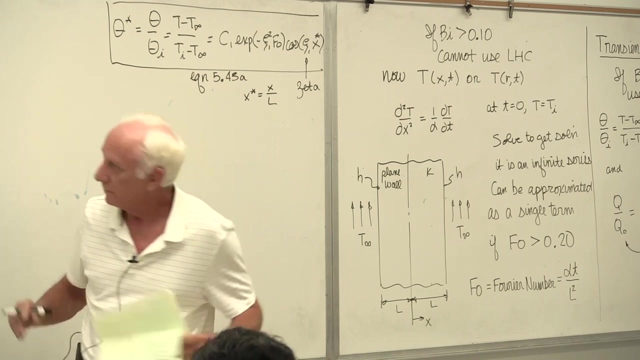 X star is x over L, the half wall thickness. It's a ratio. X star goes from 0 to 1.. What's c1 and zeta 1? They're constants. Where do they come from? Table 5-1.. 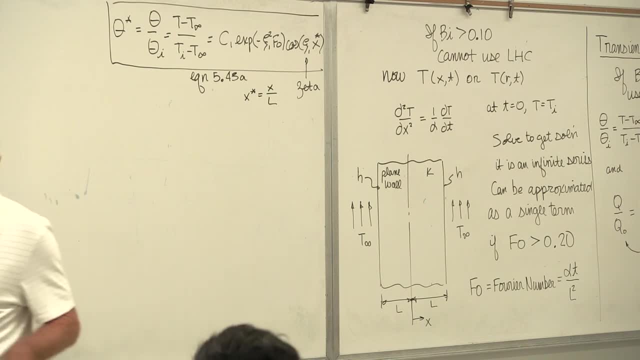 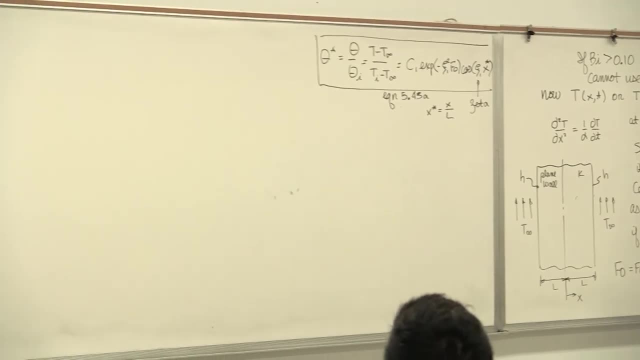 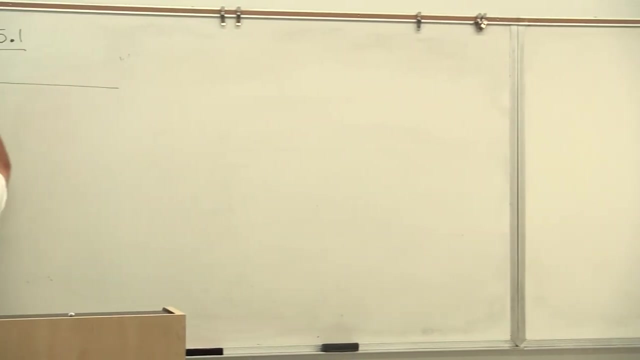 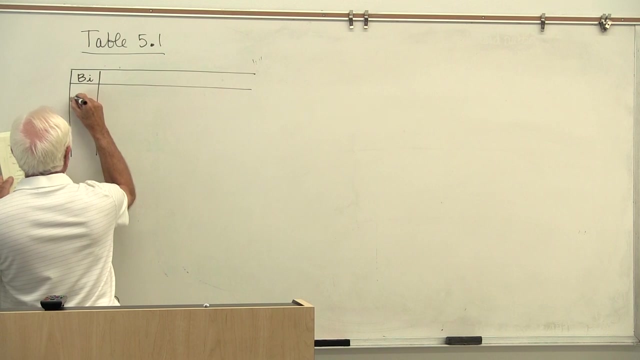 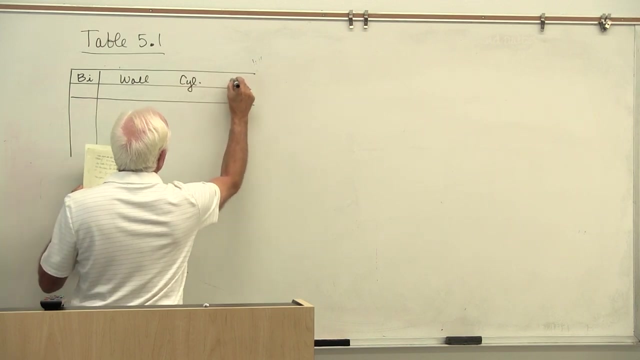 I'm going to put table 5-1 over there because I'm going to use it for an example problem later, So I'll put it over here. This is the format of the table: Plain wall, long cylinder and sphere. 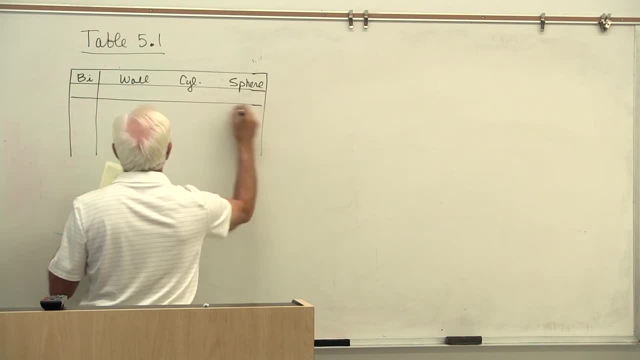 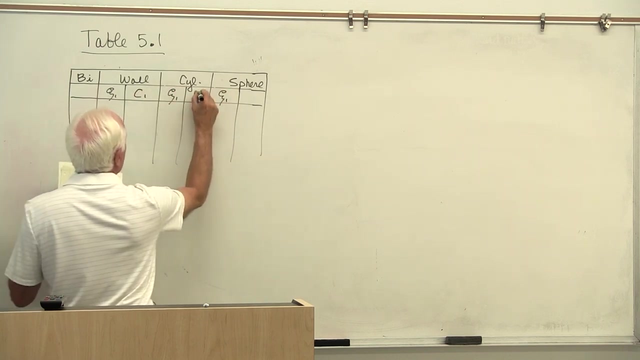 Each of them has a zeta 1 and a c1.. So c1 and the zeta 1 come from table 5-1.. And at the bottom of table 5-1, it tells you: 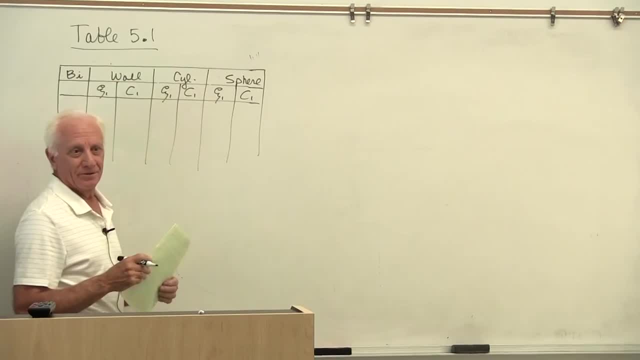 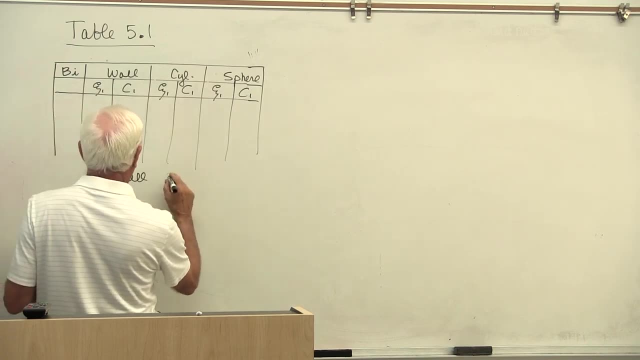 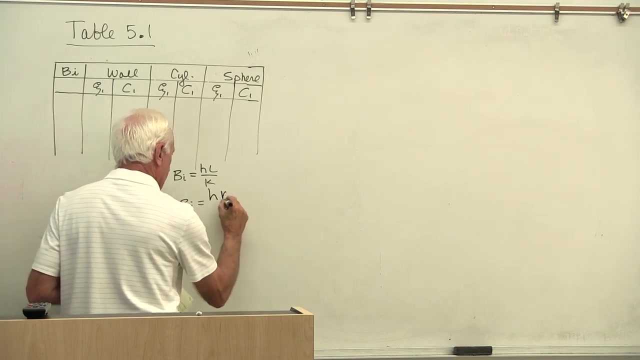 If it's a wall, we have VOHL over k. If it's a cylinder or a sphere, VO is equal to R naught A sphere VO is H R naught over k. 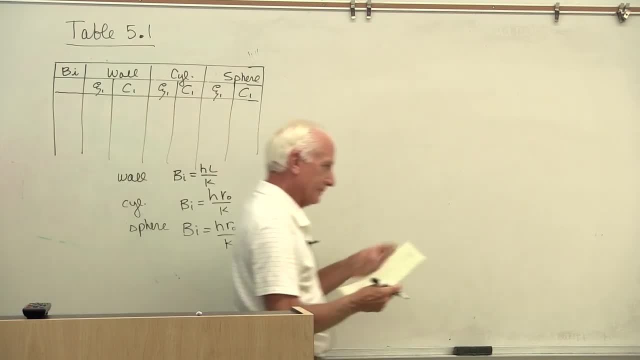 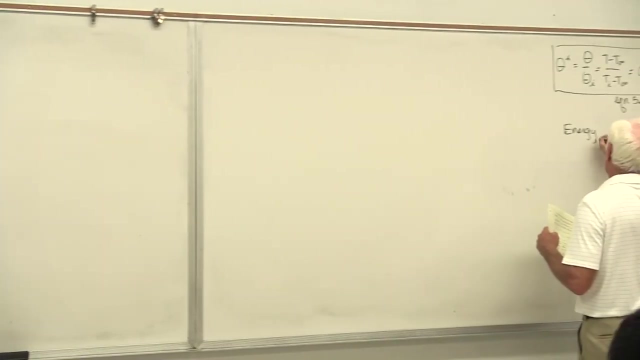 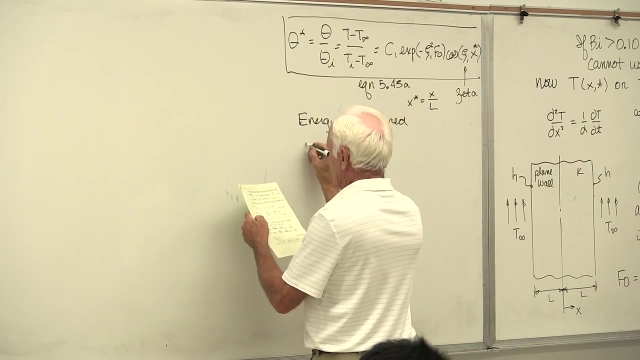 The total energy transferred q integral rho c t minus ti d volume. Integrate that over the volume with time. 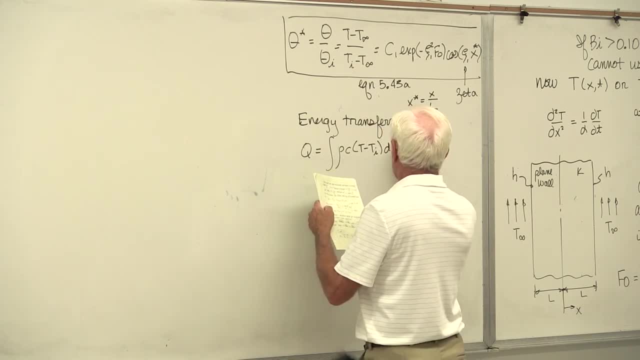 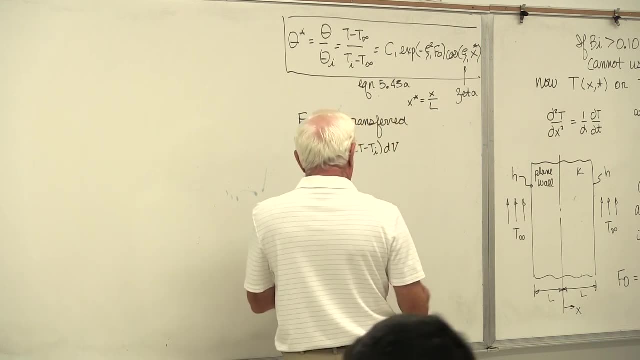 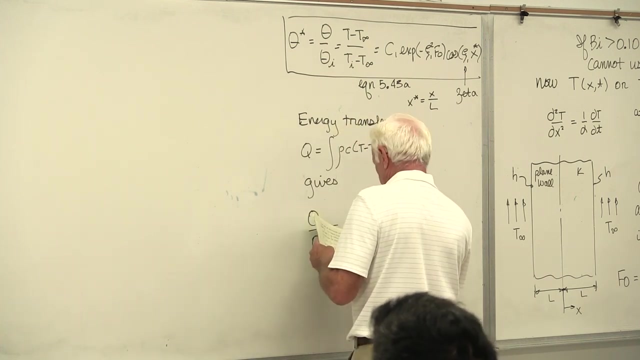 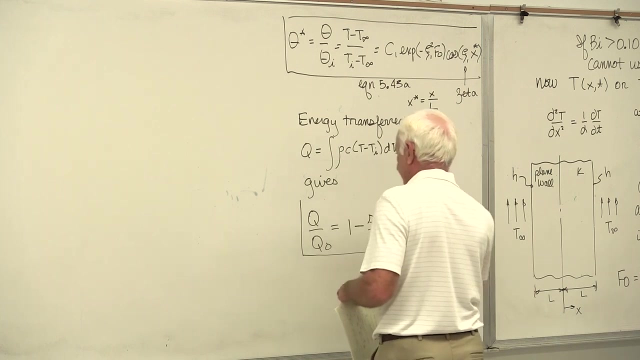 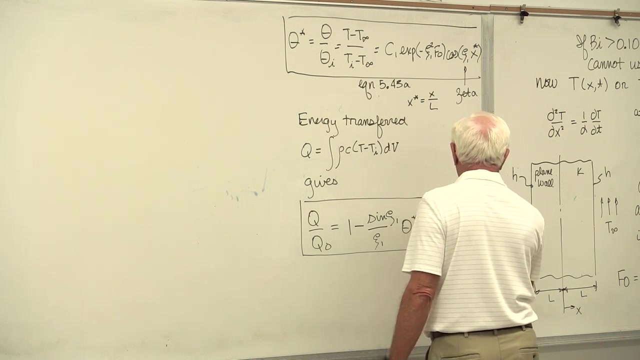 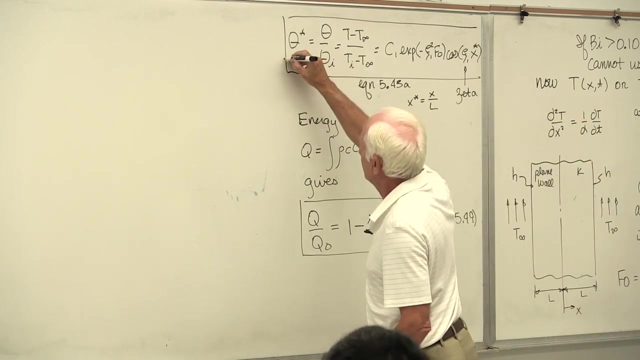 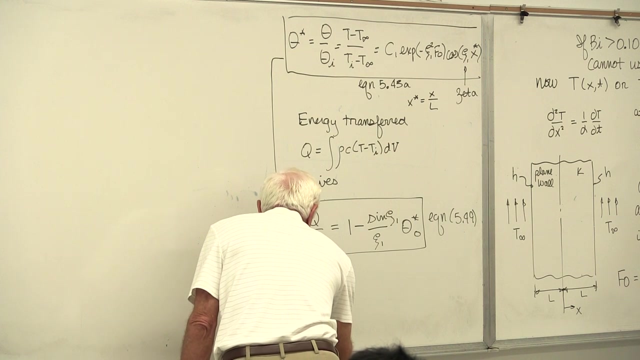 This gives. This gives Q over Q, naught 1 minus sine zeta, 1 over zeta 1, theta naught star Equation 549.. If you want, the center temperature of a wall that occurs at x equals zero. 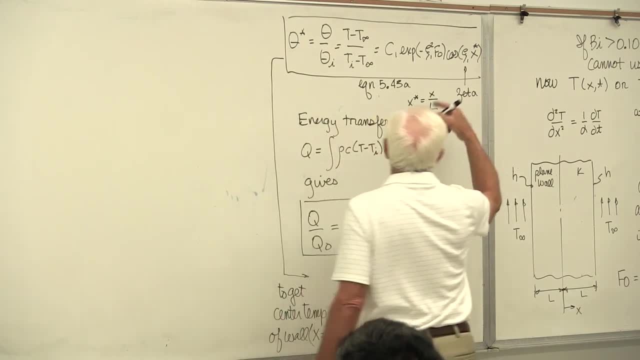 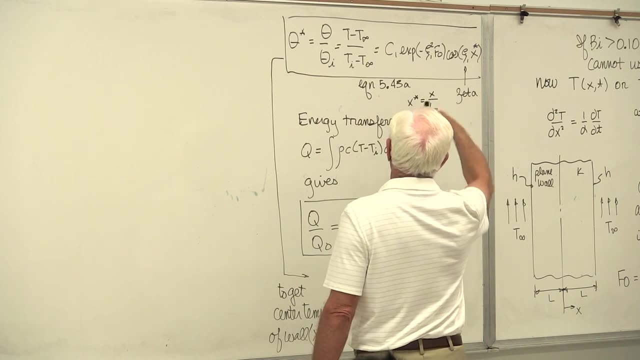 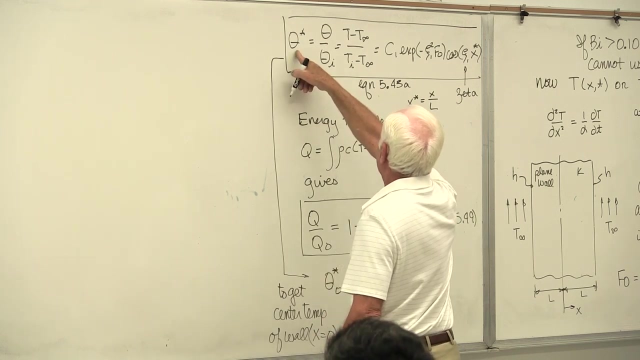 Just put the zero up here for x star, of course, And that is cosine of zero, which is 1.. So theta naught star The naught means that x equals zero is equal to C1, exp. zeta 1 squared Fourier. 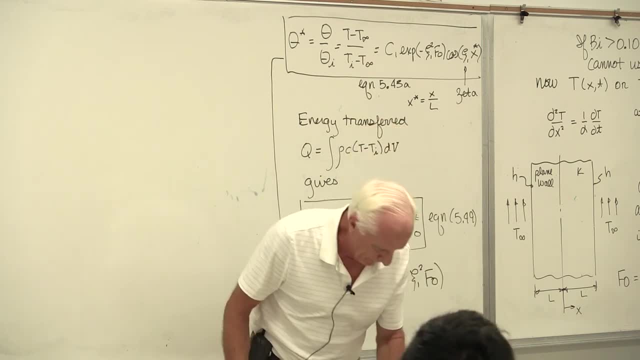 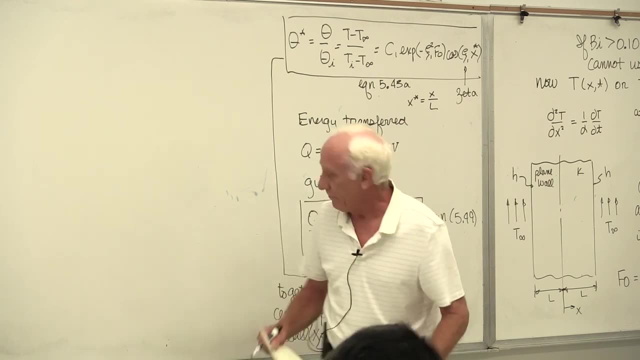 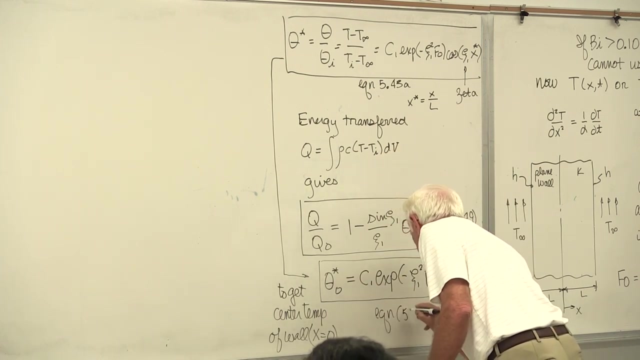 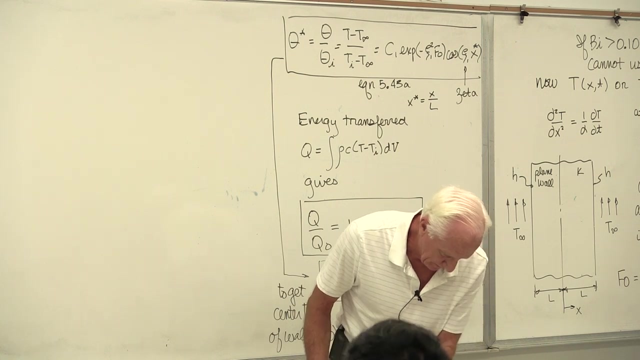 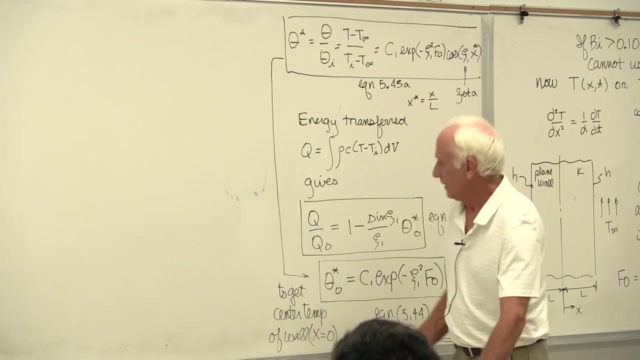 Okay, And that. let me check where that is in here. Okay, that is equation 544.. Okay, I think that's all we have there, Right? Okay, with a plane wall. there are three things you can get from this. 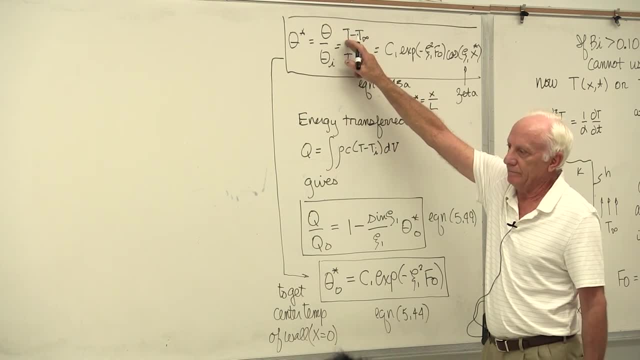 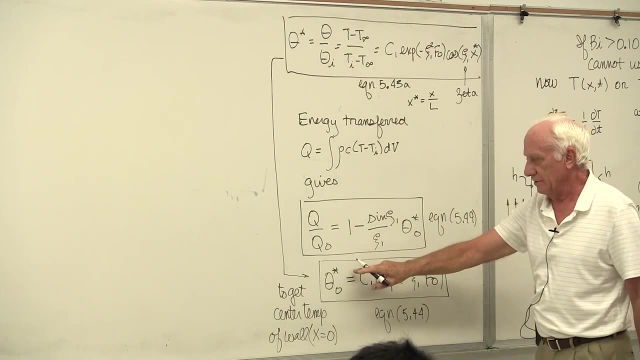 The temperature at any x and any time. You want the temperature at any x and any time, use this equation. If you want the center temperature of the wall, use this equation. As a matter of fact, you can just put: x equals zero here. 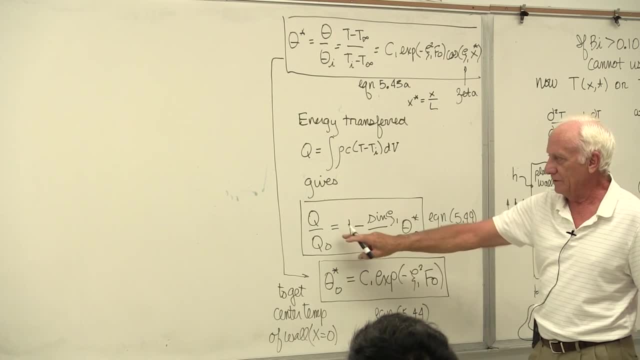 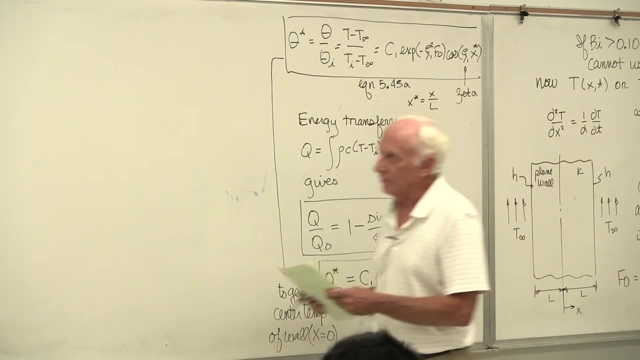 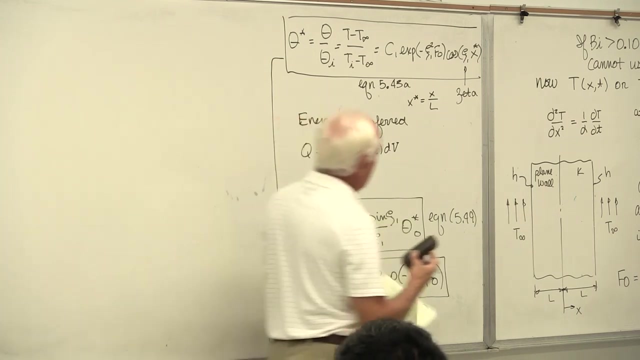 It doesn't make any difference, But this is a simpler version. Okay, If you want the Q, the energy transfer in joules, use that equation. So here is the summary for the three. I'll put it right by here. 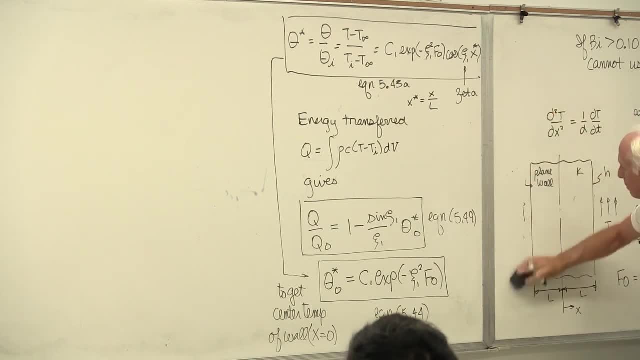 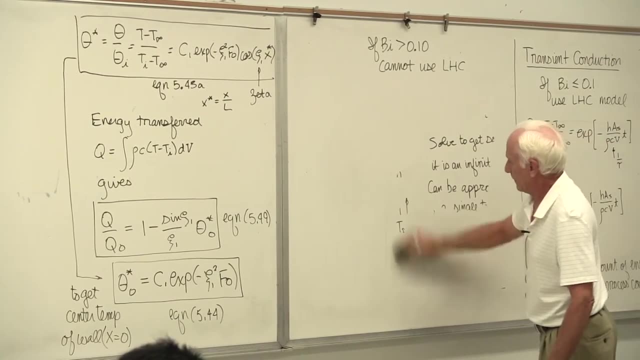 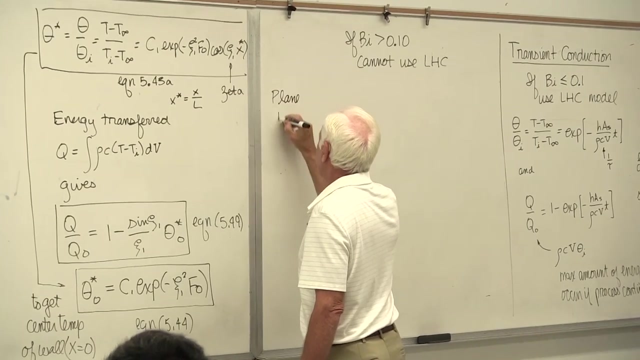 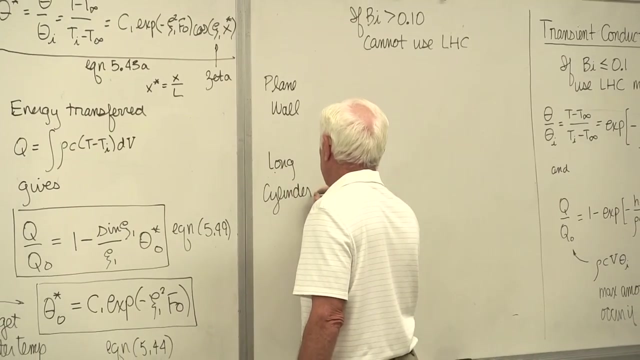 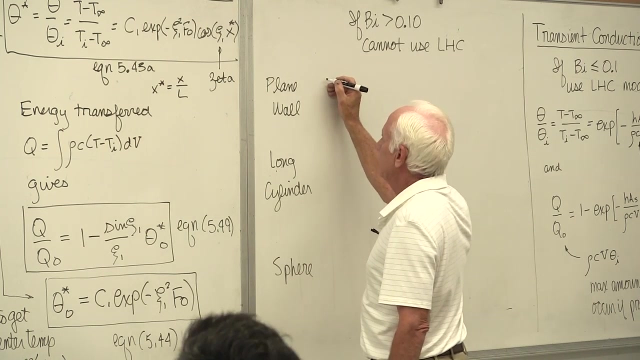 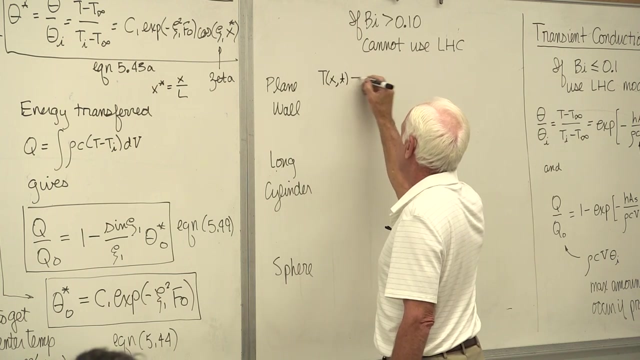 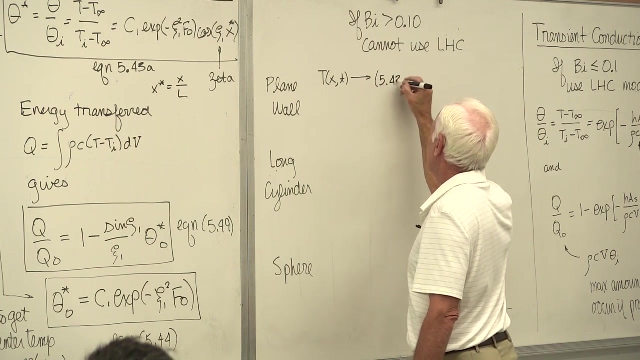 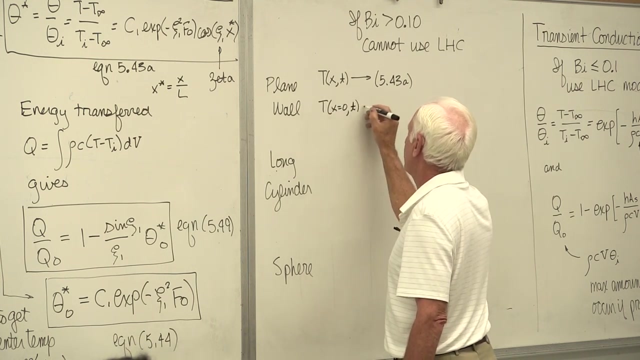 You cannot use this, I'll put it right here. So: plane wall, long cylinder and a sphere Plane wall for the center temperature, or the temperature at any x or any time. There it is Equation 543a: The temperature at the center for any time. 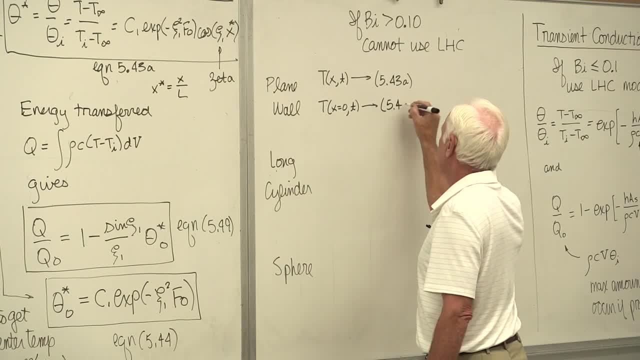 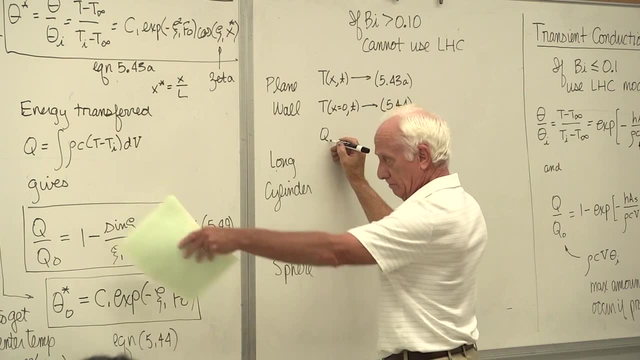 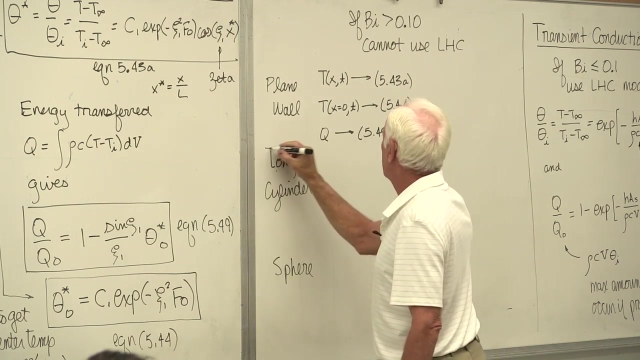 There it is 544.. Energy transfer: Q naught or Q, Equation 549.. Long cylinder: any radius, any time, Center line of the long cylinder for any time And finally, the energy transfer as a function of time. 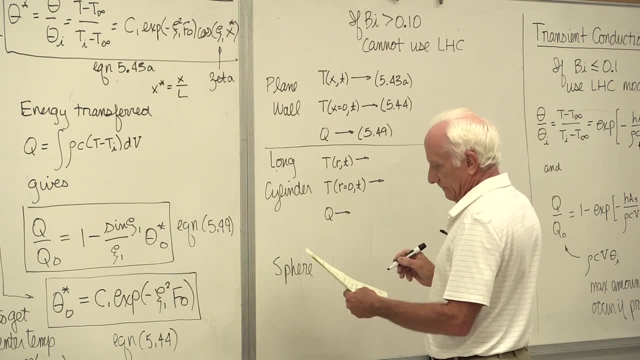 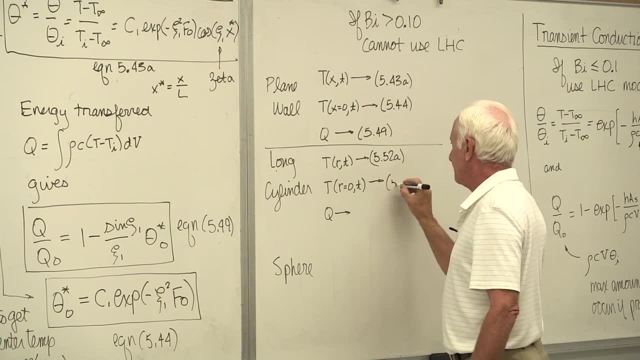 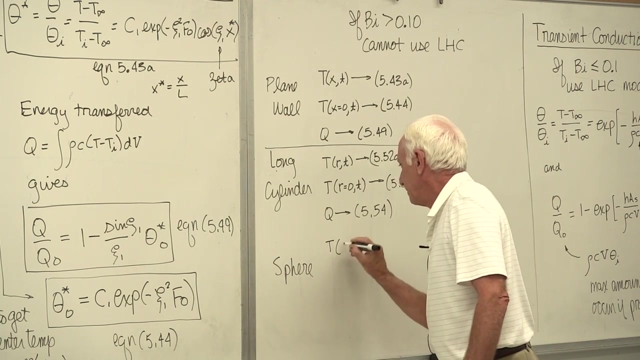 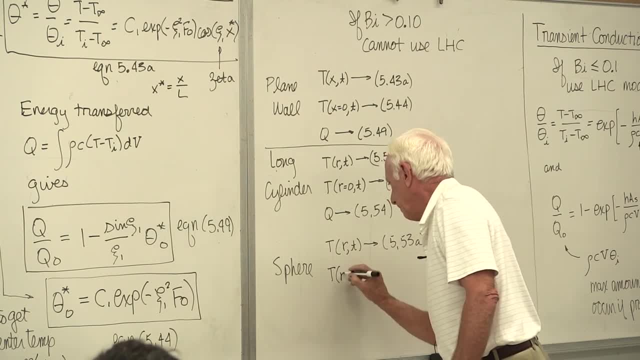 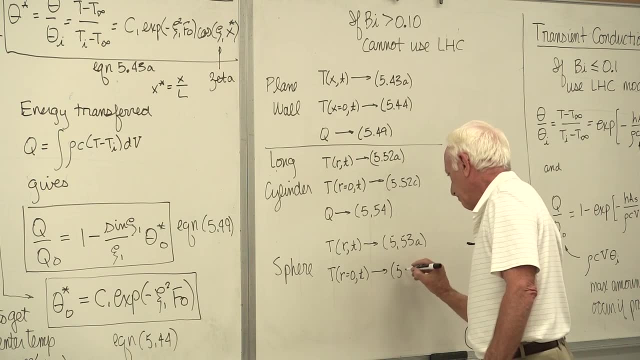 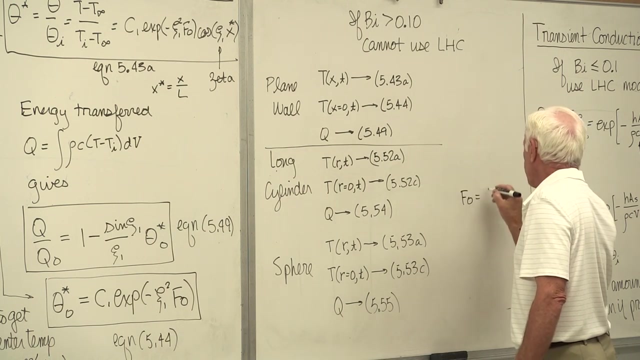 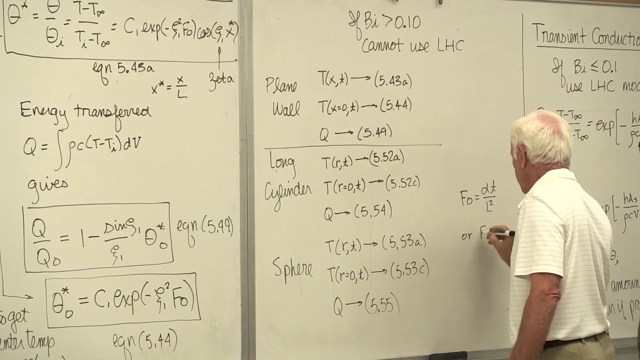 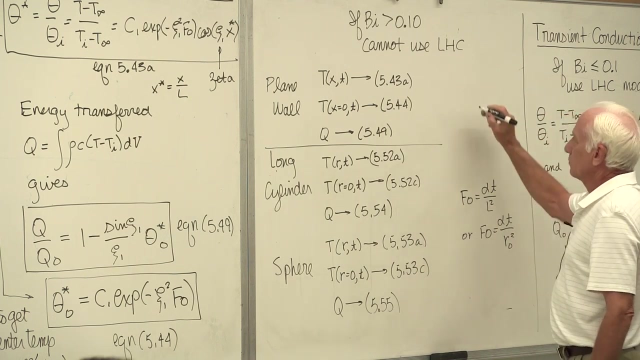 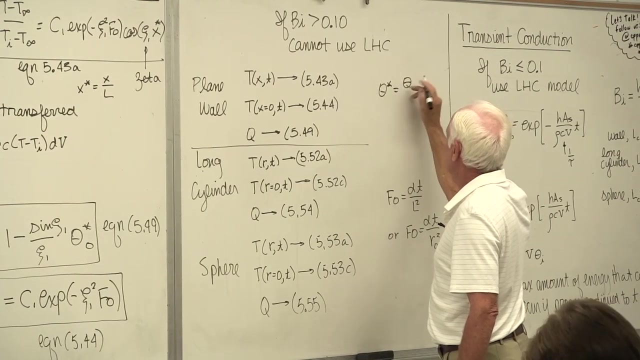 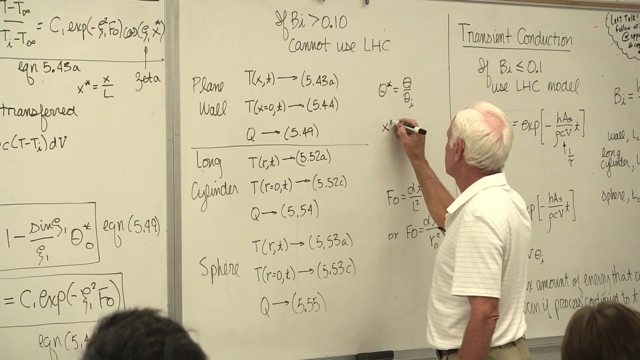 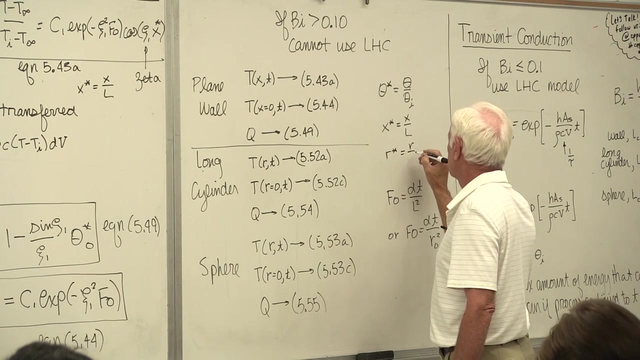 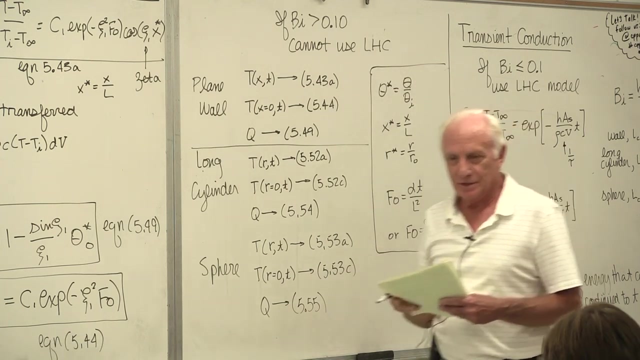 05.53a, 05.53a, 05.53a, at any time. 553C- Energy transfer to the sphere as a function of time. 555.. Thank you, So pretty much there's Chapter 5 on the right side of the board. 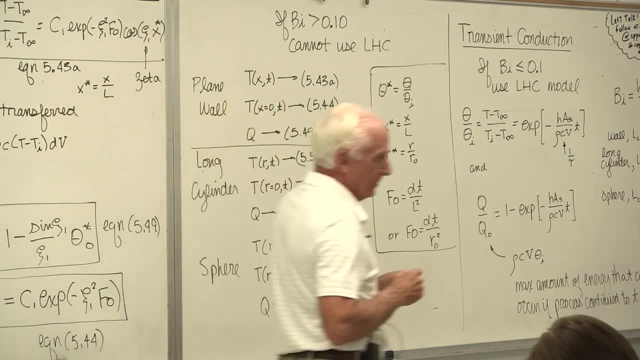 That's it. That's Chapter 5.. Nothing else to worry about. That's all we're going to do. We're not going to do the infinite series. no, That's too complicated. All our problems pretty much if they're not, if they don't satisfy the B on less than 1 tenth. 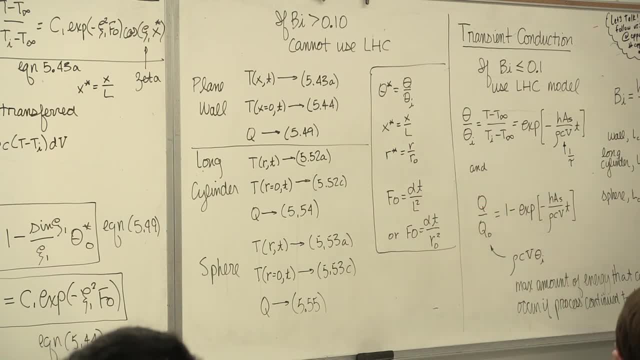 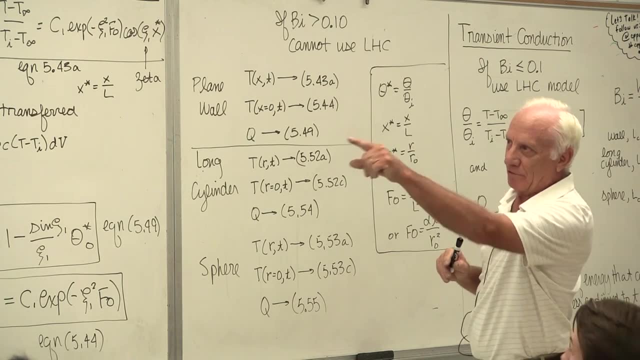 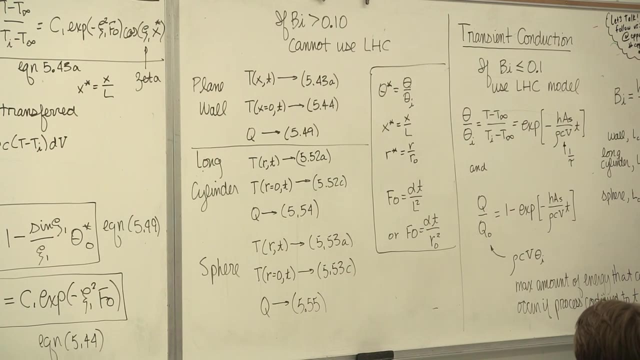 pretty much. they're going to have 4EA greater than 0.2.. Okay, You need that Table 5-1 with these nine equations. Nine equations: Everything's done with those nine equations Over here, only two equations. 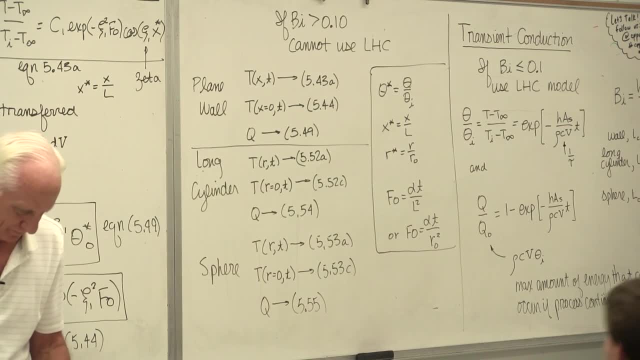 Okay, What's the difference in these two guys? I'll put that here and then I'm going to erase it. I'll put it over here first. I'm going to do two pictures for you. Show you the difference in those two on the panel over there. 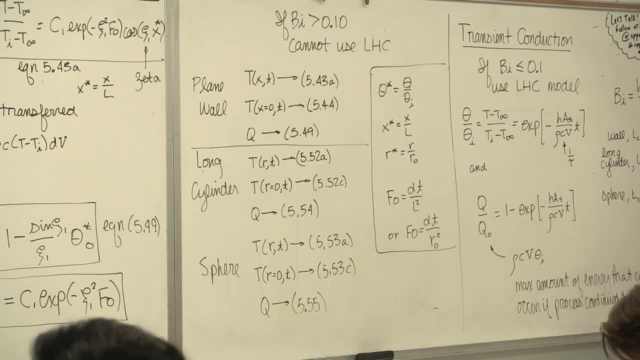 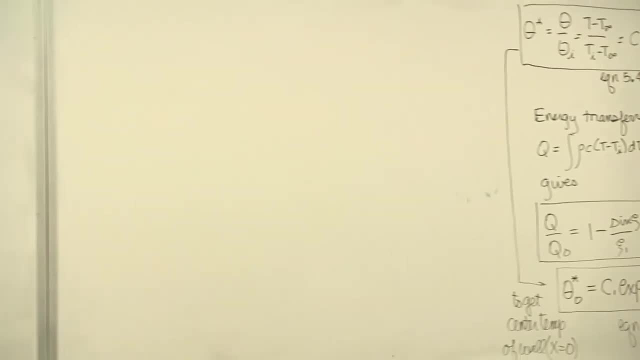 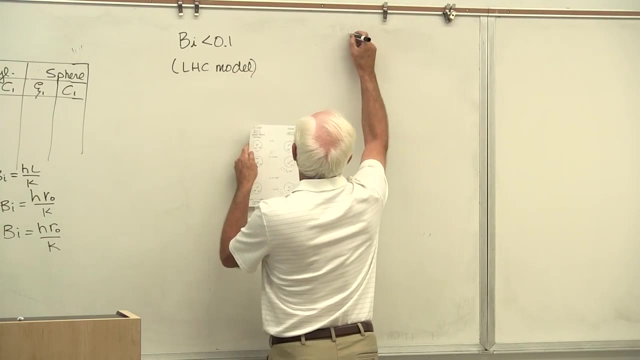 I'm going to look at a sphere being cooled. First of all, the B-O is going to be less than 1 tenth. This is lumped heat capacity model. And then I'm going to look at the actual one: what actually occurs? 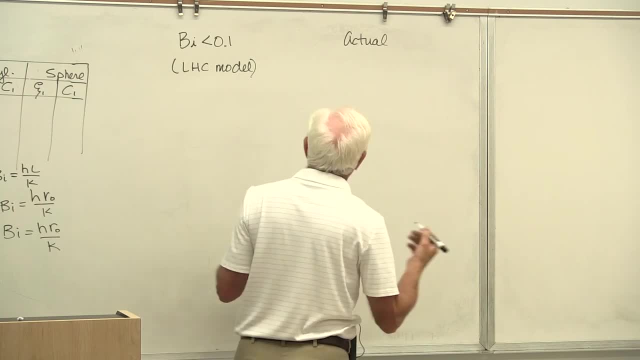 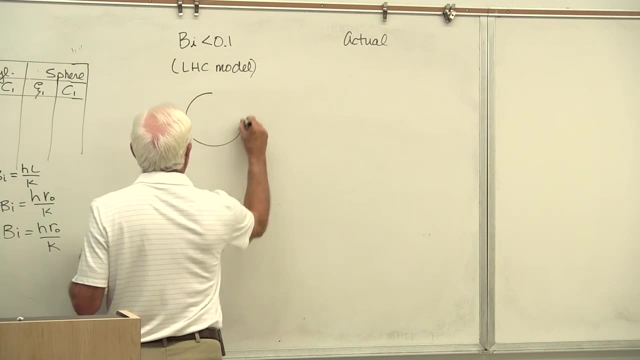 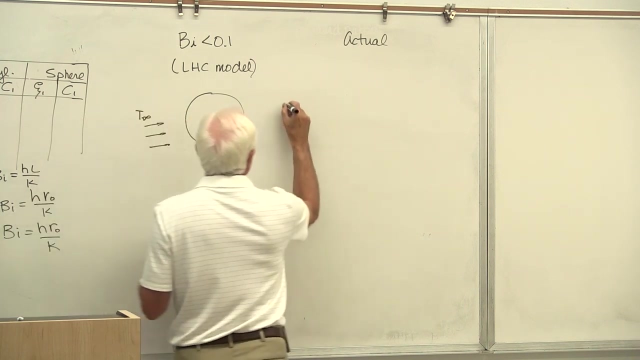 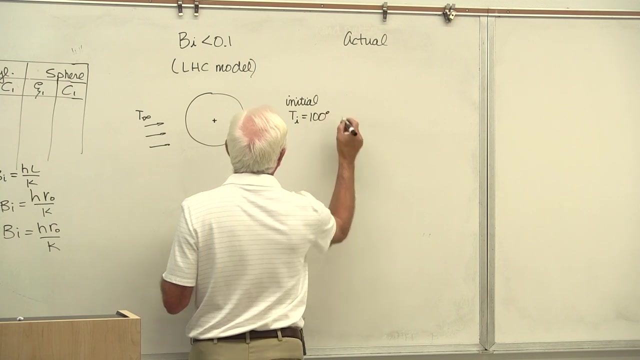 Okay, It's valid for B-O greater than 1 tenth. So here is a sphere. We have a fluid blowing over it at T infinity. This is initial. TI is 100 degrees. Here's the actual picture. We start off. 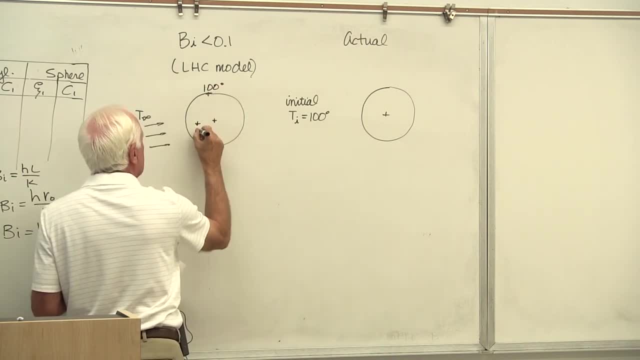 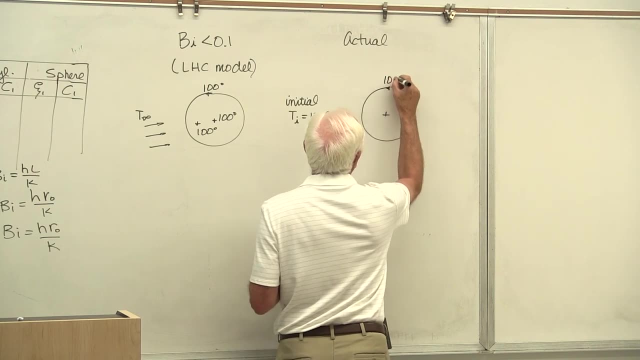 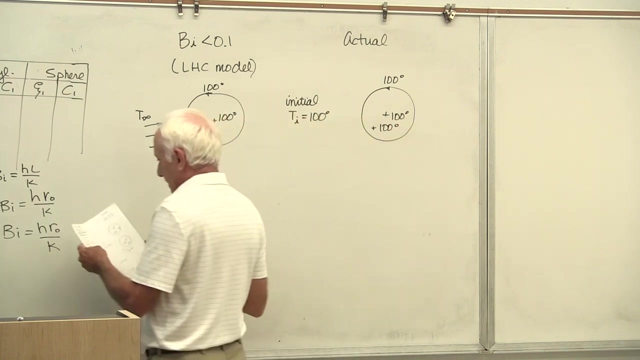 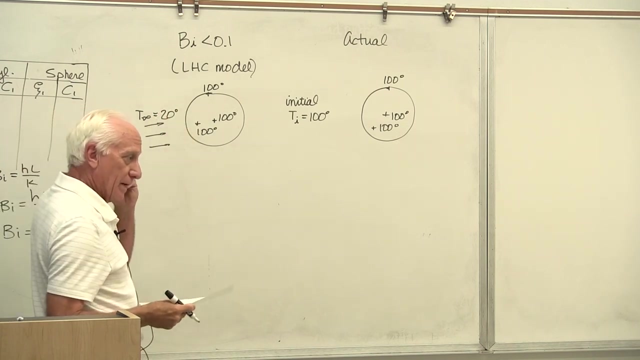 Everywhere the sphere is at 100 degrees. No matter where you look at the radius, it's 100 degrees Everywhere. The initial temperature: I'm going to just assume that the temperature T infinity is 20 degrees C. 20 degrees, just to put a number in there. 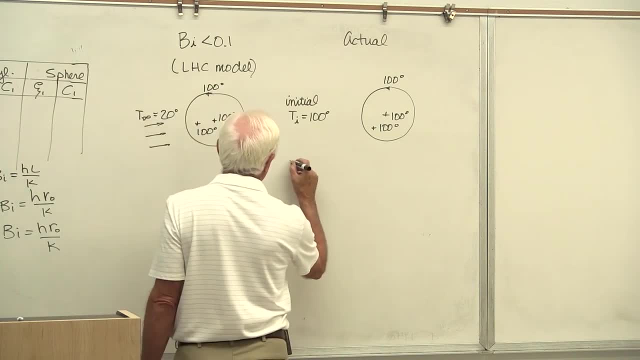 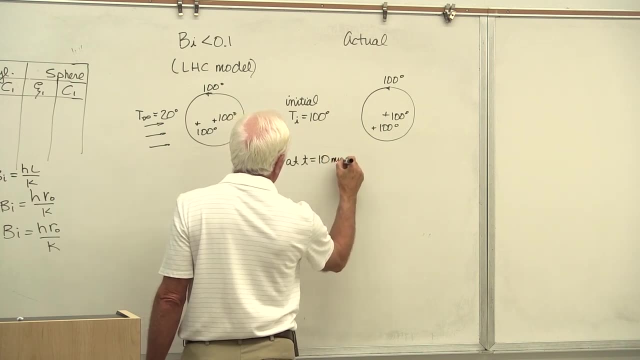 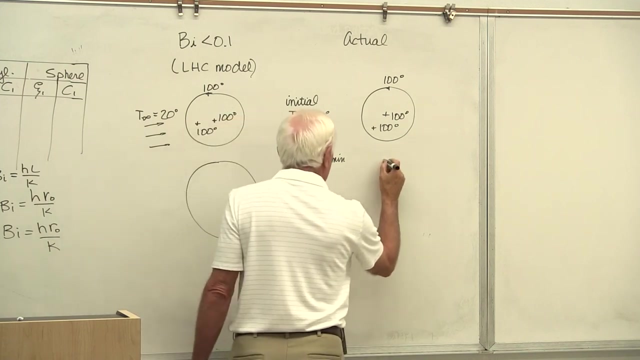 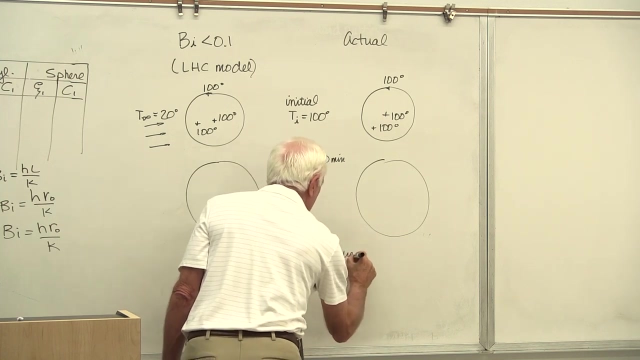 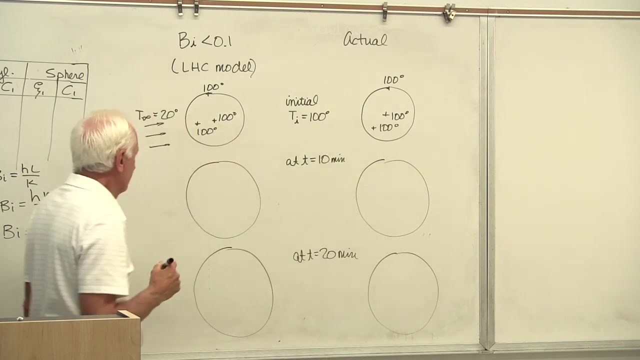 Okay, Uh, At time equal 10 minutes. I'm just making that up, Whatever, Okay, Here's the picture. Here's the picture At time equal 20 minutes. Here's the picture. There's the picture. Lump T capacity. 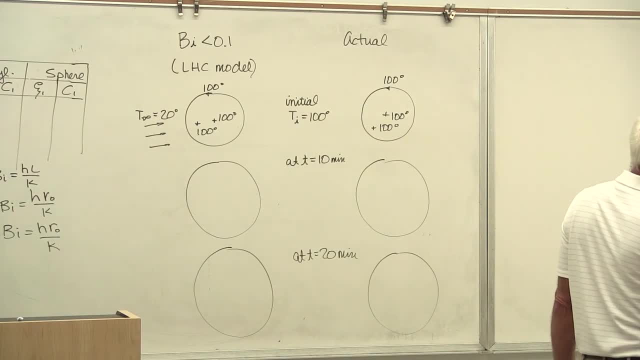 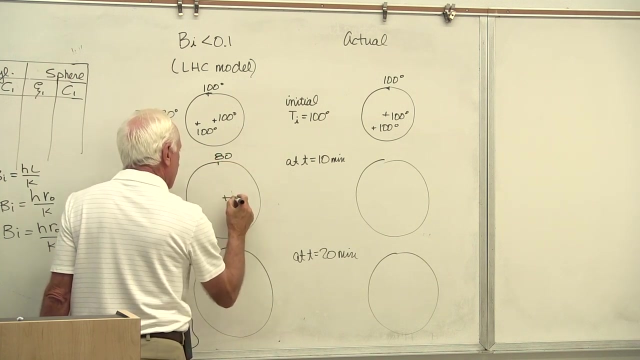 Temperature is not a function of X or radius. It's only a function of time. far right hand equation: It's not a function of that. The sphere starts to cool down. The outside surface now is 80 degrees. The middle of the, the middle of the sphere, is also at 80 degrees. 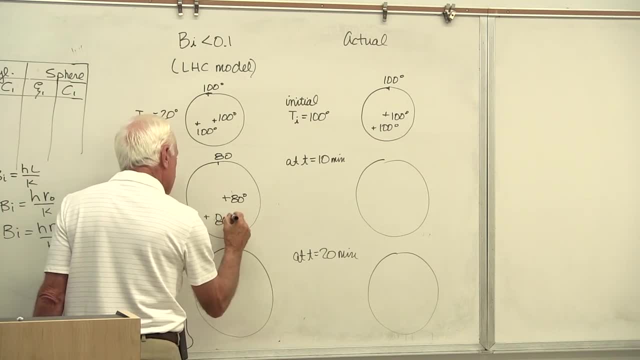 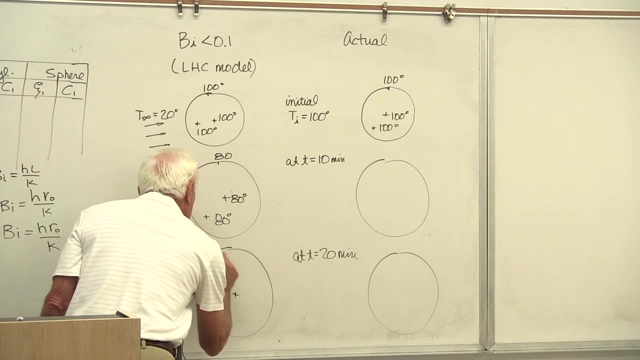 Anywhere inside the sphere at any radius is 80 degrees. I wait longer. It cools down so fast. I'm going to go back to that. I'm going to go down some more. Now the outside of the sphere is 55 degrees. 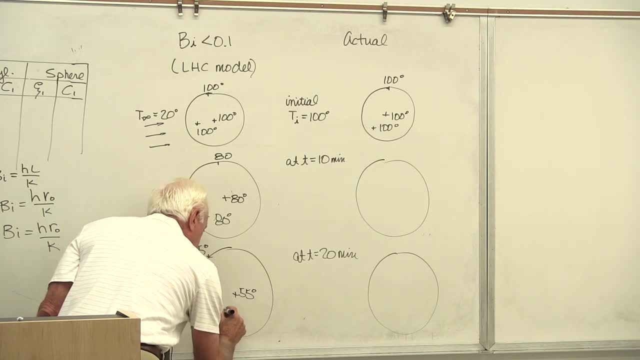 The center of the sphere is 55 degrees. Any radius in the sphere at that time is 55 degrees. That's the Biot model, Now the real one. If the Biot, let's say, is greater than 110, this isn't going to work. 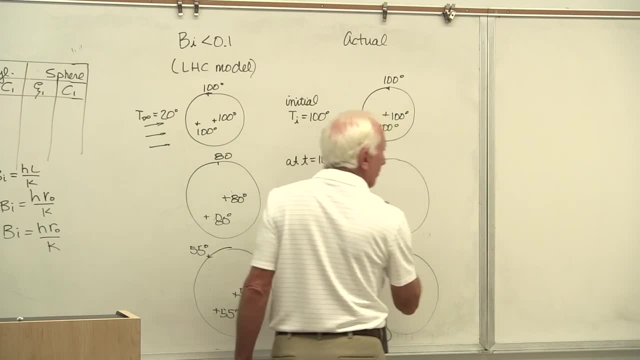 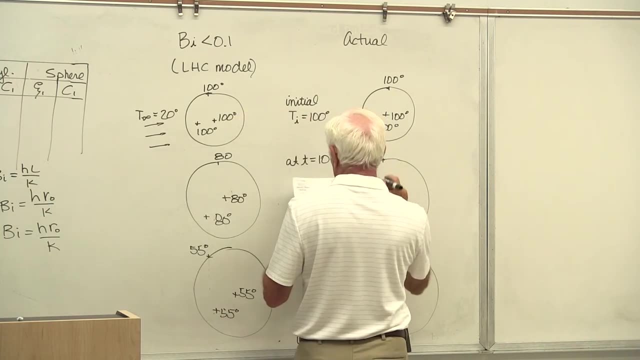 Okay, Uh, Which part starts to get colder faster? Oh, the surface. The surface is exposed to that fluid at 20 degrees. So up here now I'll assume that's cooled down to 75 degrees. Of course the center might still be at, uh, like this, right here, uh, let's just say the. 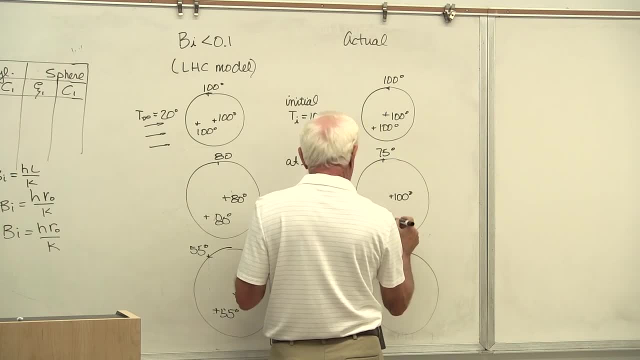 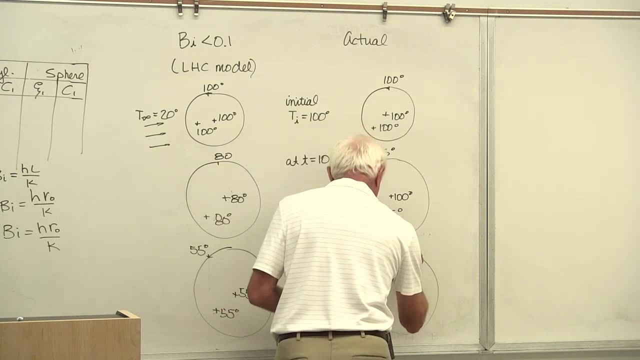 center in this case is at 100 degrees. Somewhere else this temperature might be 85 degrees. Wait a while longer. The surface cools down some more. Now the surface is at 50 degrees. The center now is at 90 degrees. 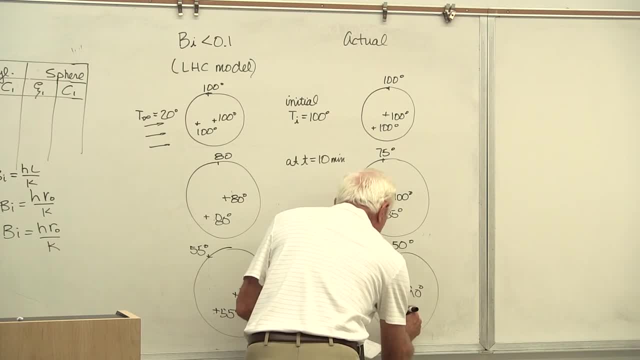 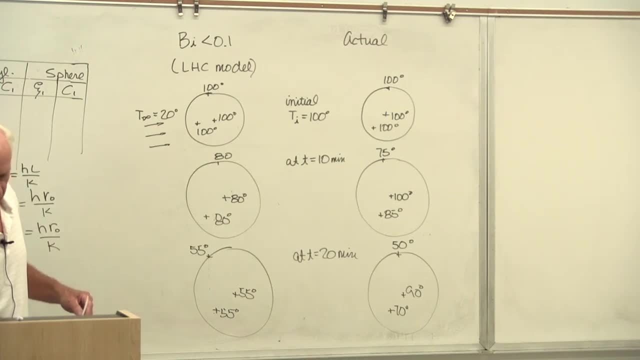 And at 50 degrees, At some particular radius, the temperature is uh 70 degrees. So, although that's the difference in the lump heat capacity model, which are these three pictures, temperature is only a function of time, not a radius, versus the non-lump. 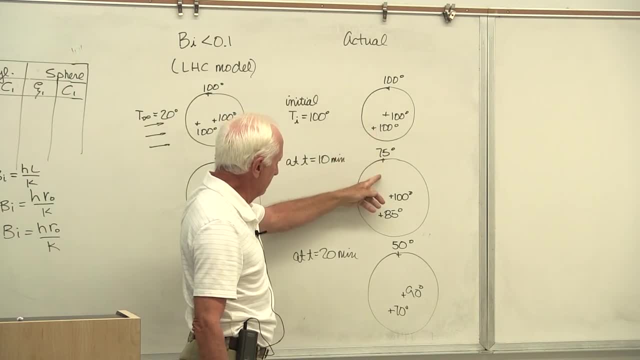 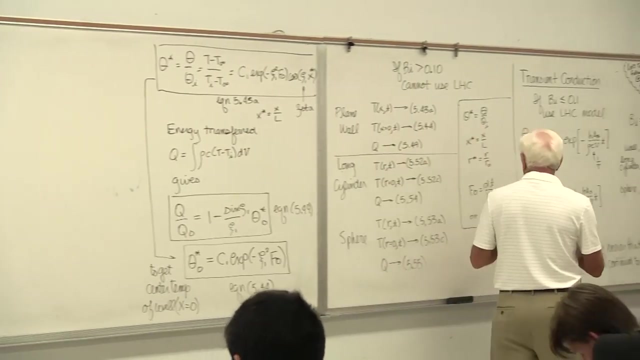 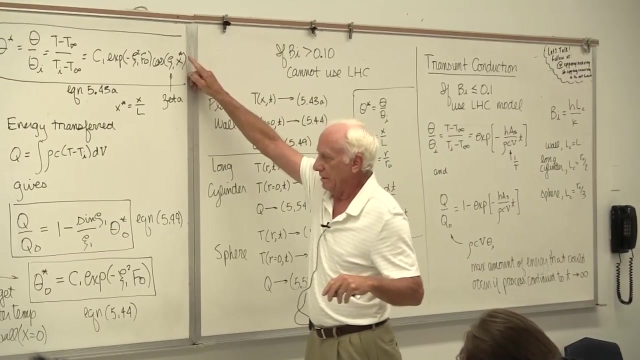 heat capacity model. Now, the temperature depends on the time and on the radius Time, and radius Time is in the Fourier. X, or radius is over here, By the way. um, any time you see an asterisk or star, let's just say star X, star theta. 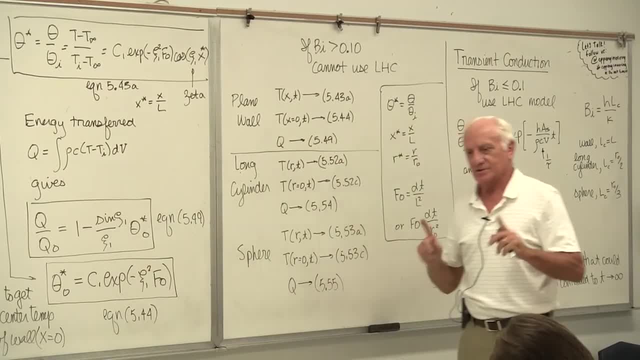 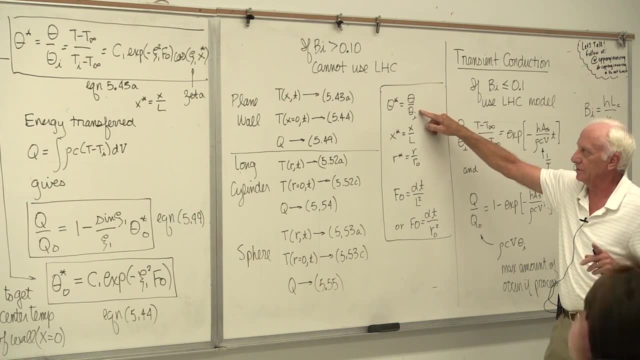 not star. that star tells you it's a ratio. If it's theta, it's star, it's a ratio. Theta over theta I is dimensionless. If it's X star, X over L, it's dimensionless. R star. 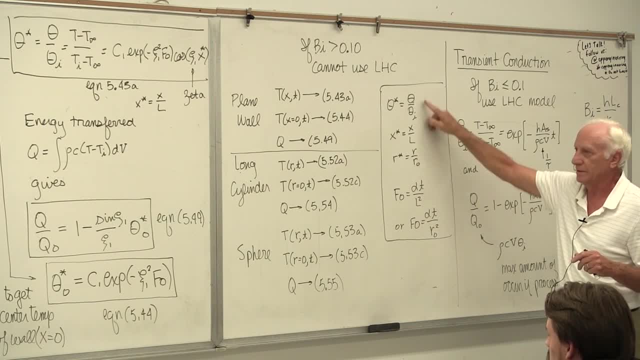 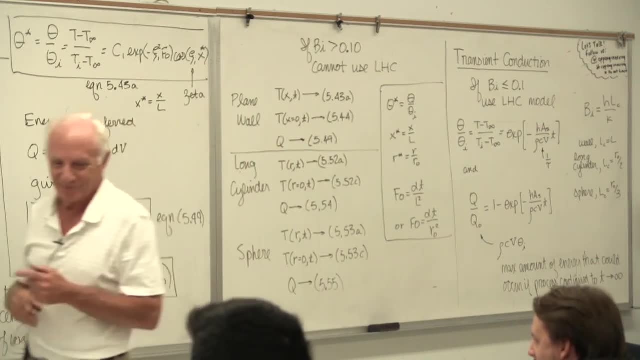 R star R over R naught. It's dimensionless. This is dimensionless, The Fourier is dimensionless. The Biot is dimensionless. As I said before, you know, we engineers love dimensionless numbers. Yeah, it makes life simple. 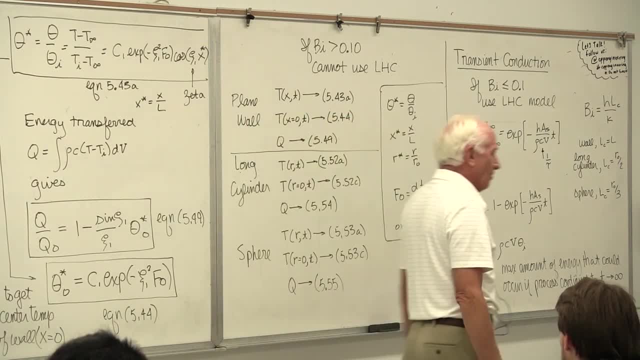 What does X star go from Zero to one? What does R star go from Zero to one? That's why we like it. Okay, Now let's work an example problem. Okay, Now, let's work an example problem. 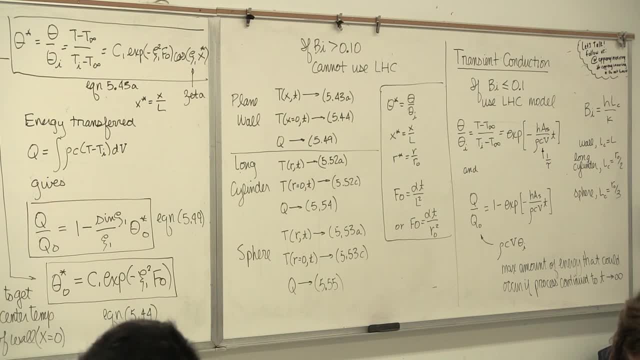 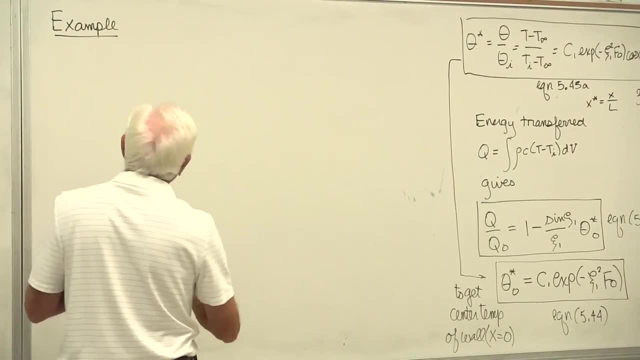 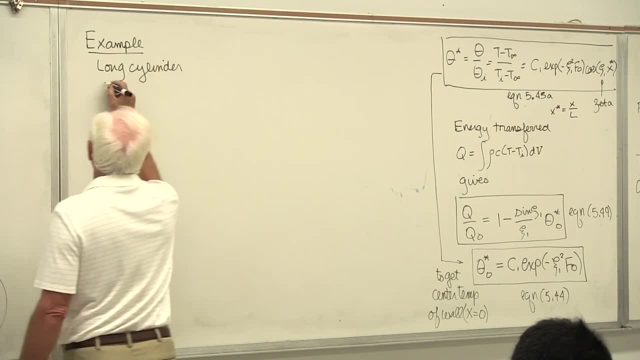 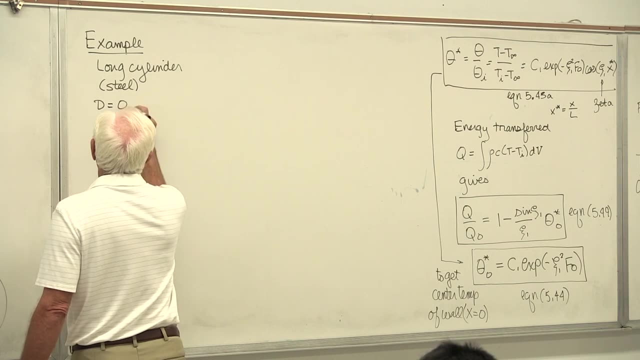 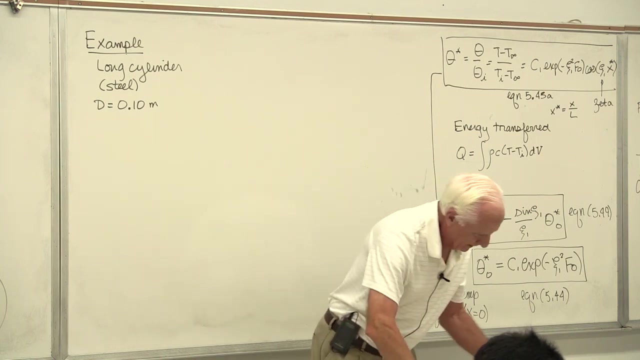 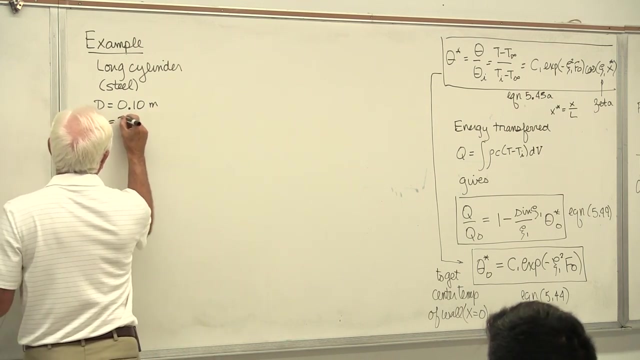 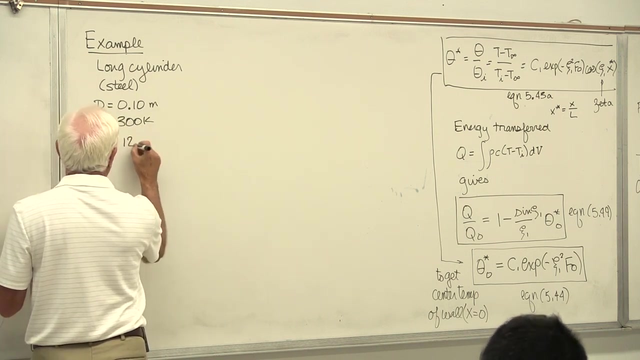 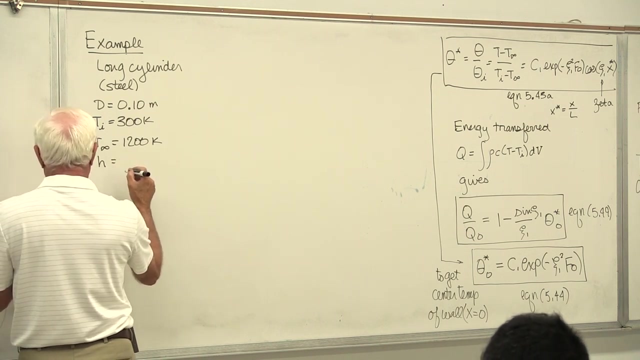 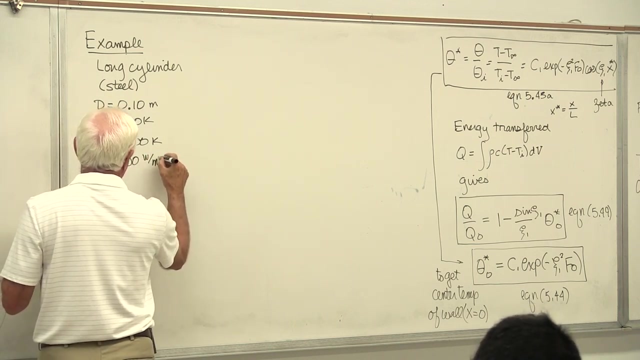 It's steel Diameter: 10 centimeters. Let's see what else we know about. it starts out at 300 K T, initial 300 K. It's exposed to an air stream at a temperature of 1200 K. The convection coefficient on the outside surface of the steel cylinder is 100.. 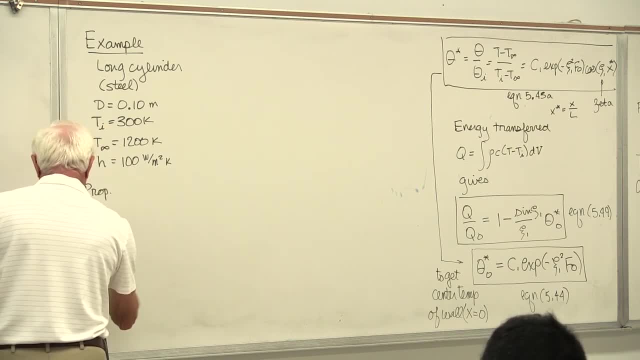 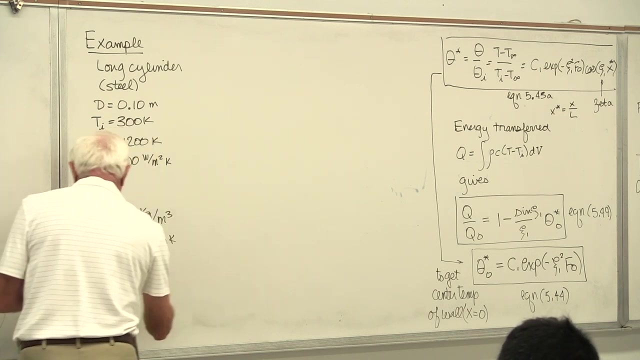 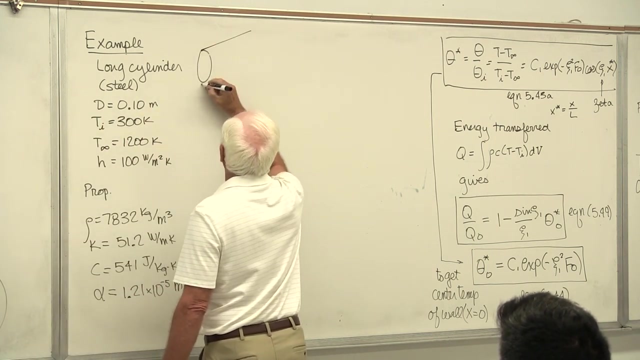 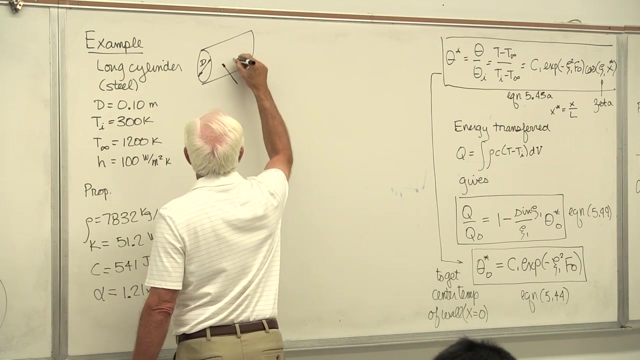 Rho, K, C and alpha thermal diffusivity And we're supposed to. I'll draw a picture of the cylinder. here's the diameter and we have a T and K going over it, H on the surface. 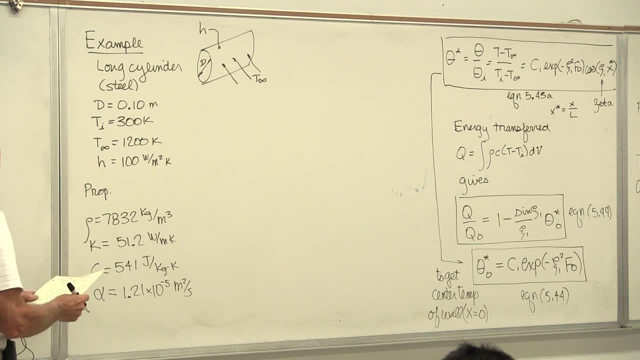 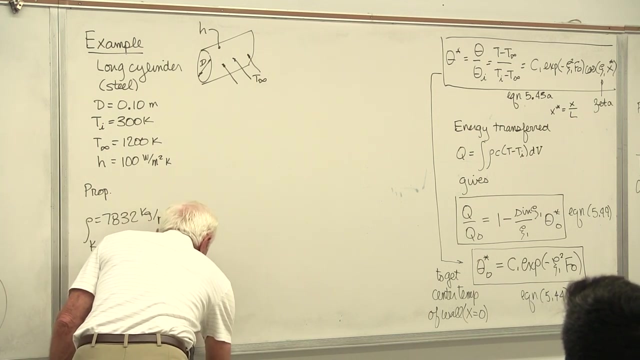 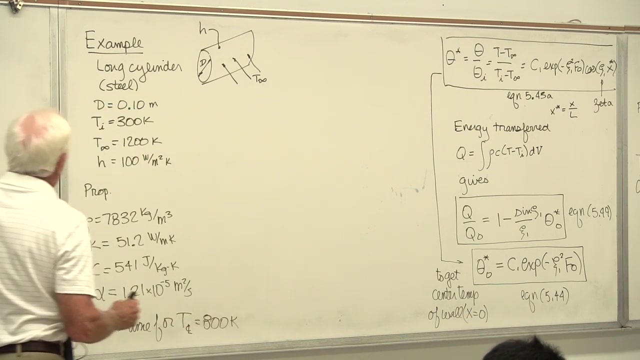 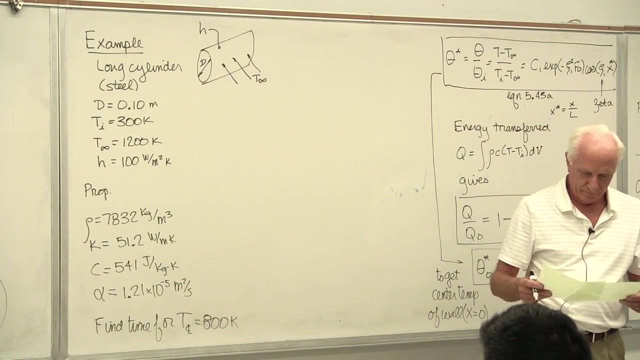 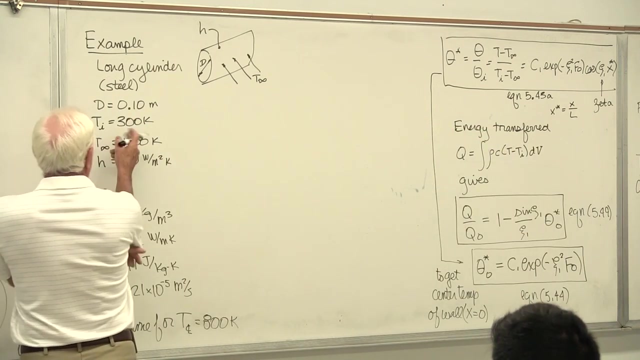 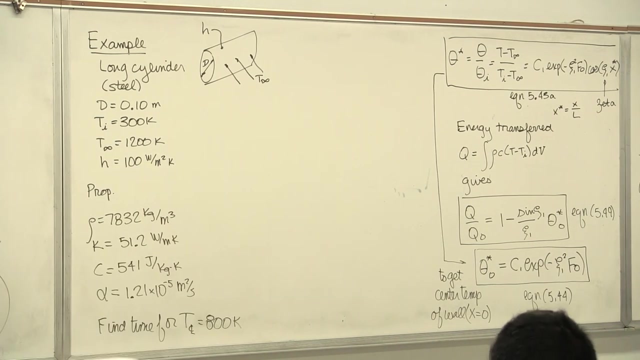 And we're supposed to find how long it takes until the center line temperature gets to 800.. Temperatures are all in specified degree Kelvin. Okay, it starts out at 300.. I don't want my properties at 300. I don't want them at 300 because if it doesn't stay at 300 long, it starts getting hot. 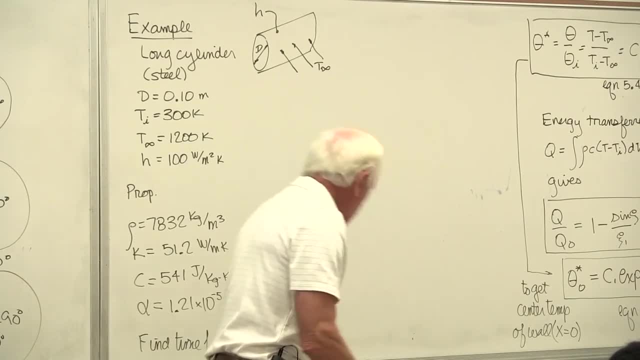 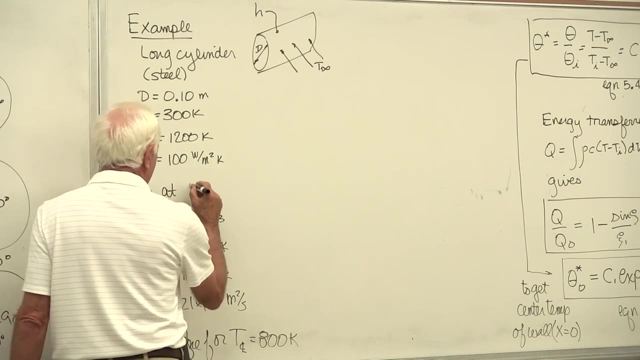 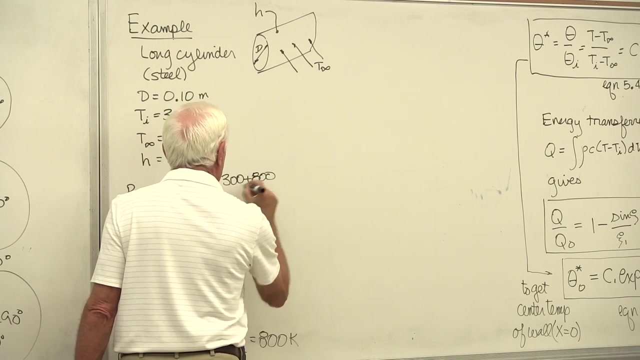 Matter of fact, it ends up getting up to a temperature of 800.. So when I find my properties in the appendix, I want to use something like a T average: 300 plus 800 divided by 2, which comes out to be 550. 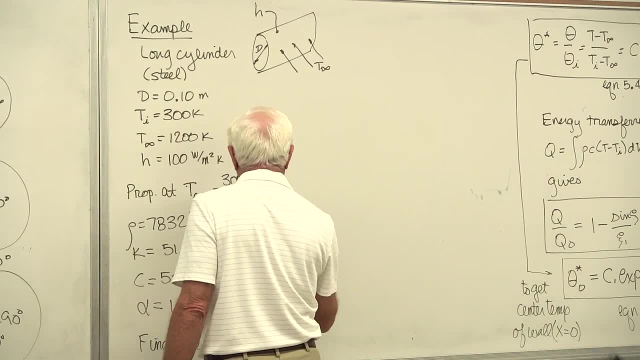 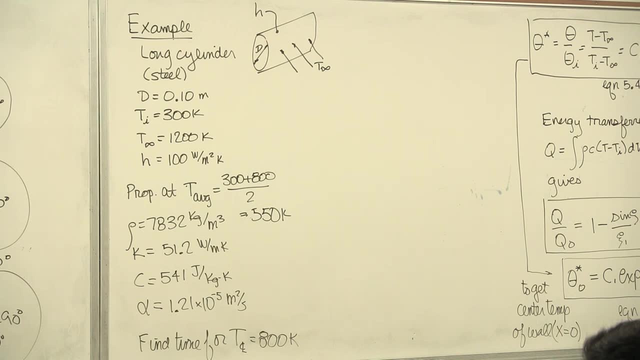 So when you go to the back of the book and find the properties, find them, interpolate them at 550.. All the density's not going to change them, There's only one density. But these three guys will. K will change, C will change. 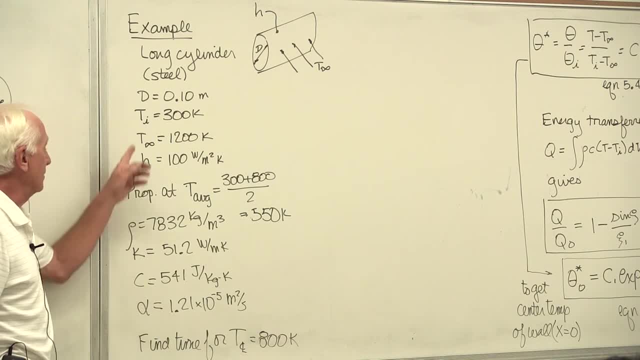 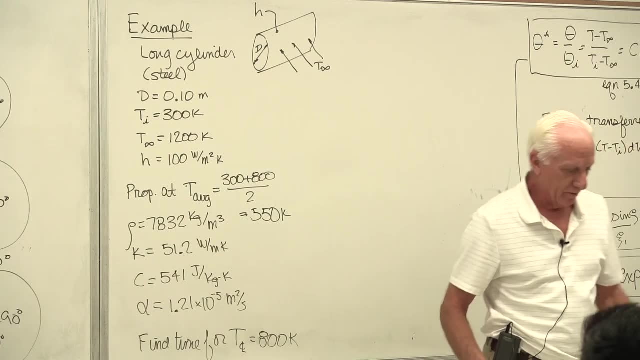 Alpha will change. So back of the book with the kind of steel you've got, find out what those values are. This is carbon steel, by the way. Okay, Now, next step. of course BO, that's always the next step. 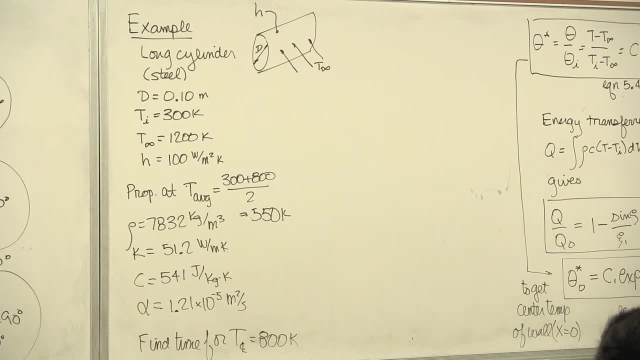 Fluid mechanics. you've got to flow in a pipeline. First step: always calculate Reynolds number. Always calculate is it turbulent, is it laminar? This is heat transfer. Always first step in transient Check it BO number. can I use lump heat capacity or no? 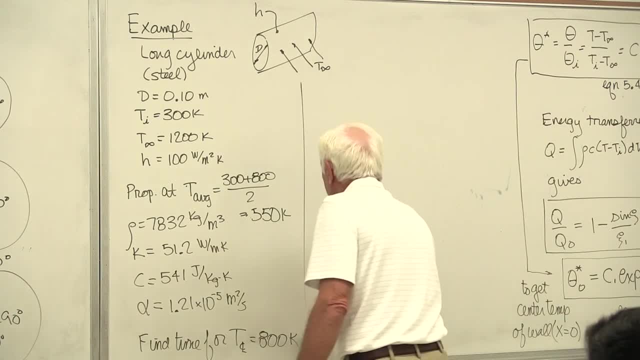 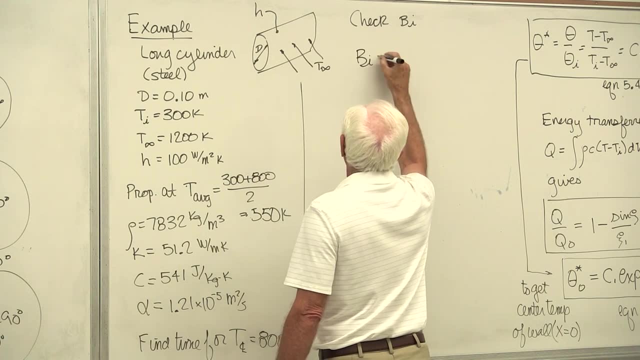 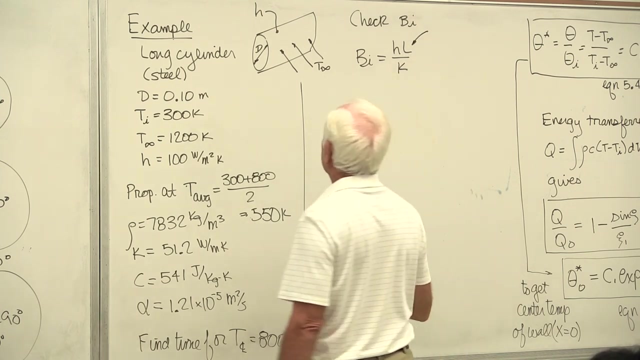 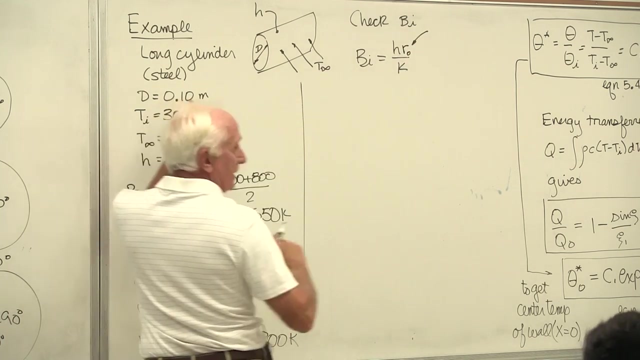 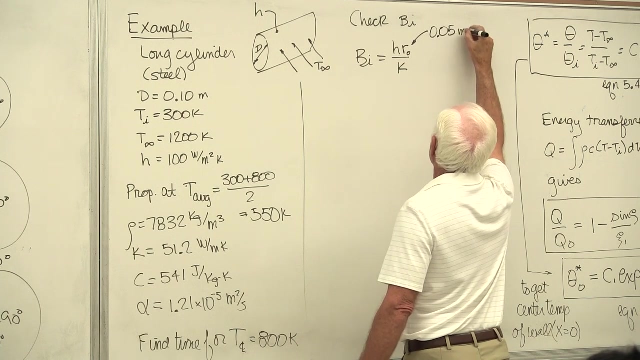 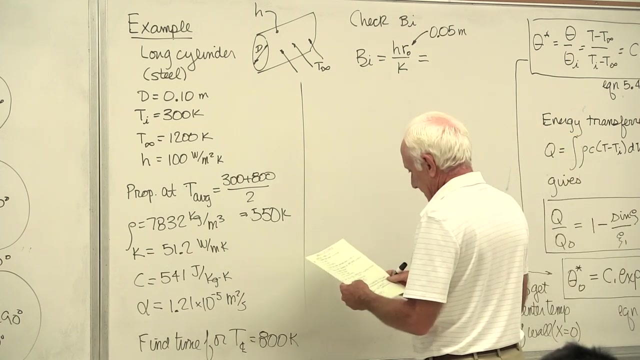 Okay, So BO number HL over K, Not HL, Pardon me. R Okay, R0.. Diameter 10 centimeters, Radius, half of that 5 centimeters, And if I do that, there it is. 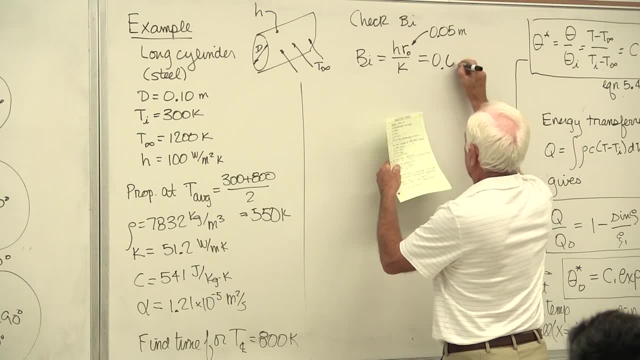 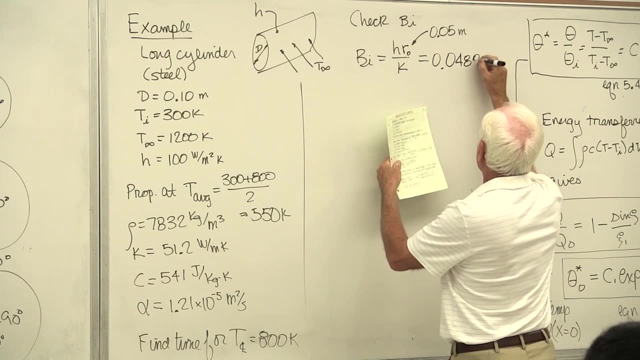 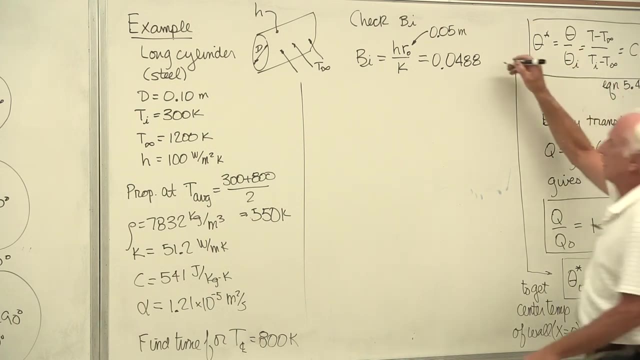 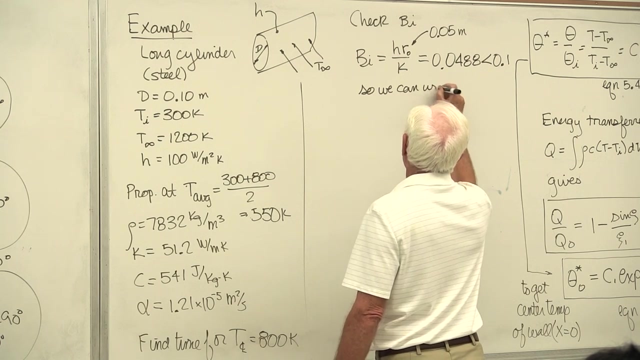 0.0488.. That number is less than one-tenth, So we can use lump heat capacity. Is that with the new properties or the initial properties? There's only one property We don't have. they don't change. 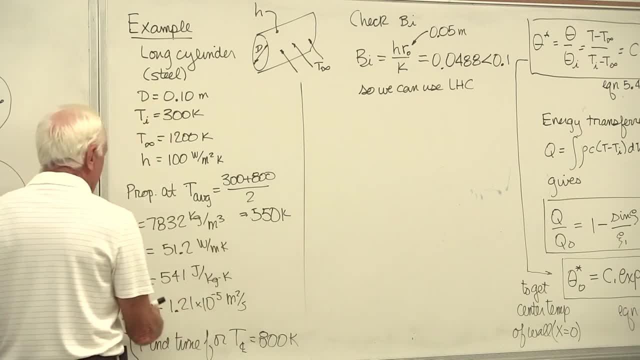 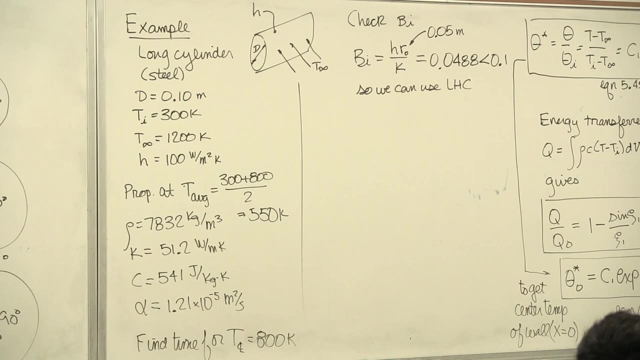 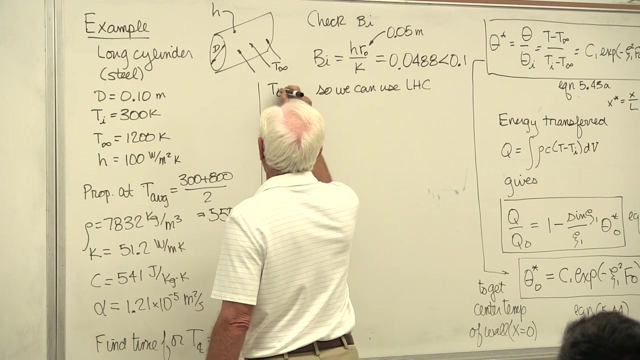 Everywhere, in every equation, you put these properties which are at the average temperature. Okay, let's see. So we're supposed to find time center temperature. okay, There's the equation right there: T center temperature. This is T center line. 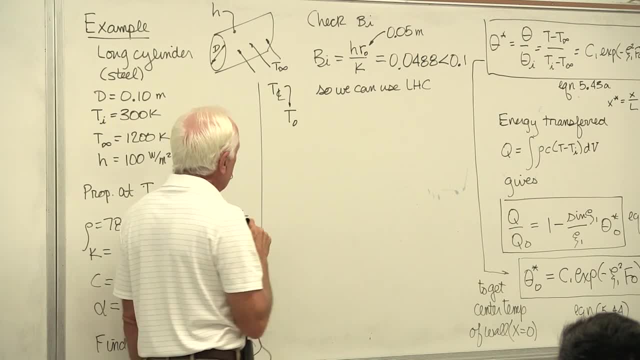 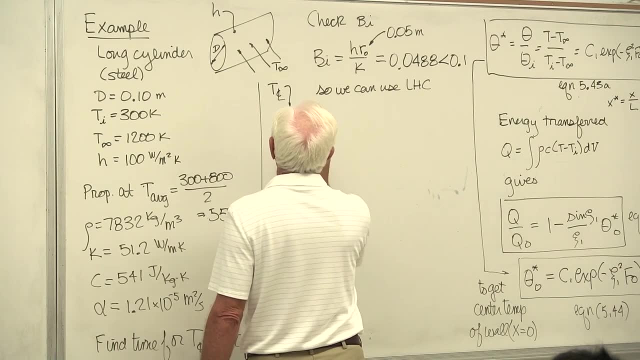 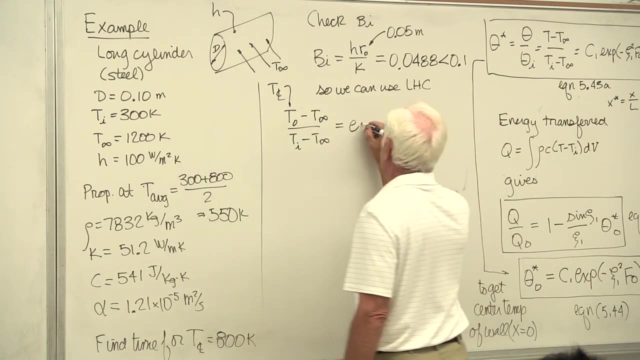 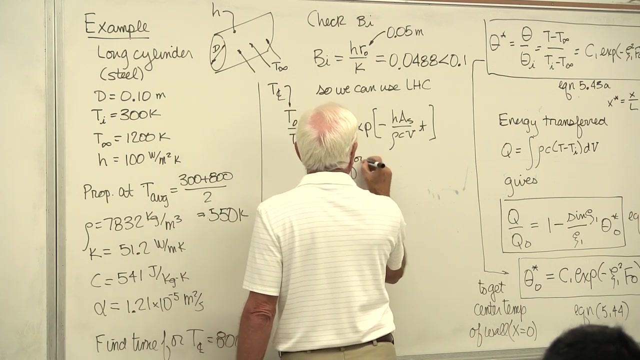 The subscript. zero means at radius equals zero T. where the radius equals zero minus T, infinity divided by T- initial minus T infinity is equal to exp minus our HAS, rho, CVT. solve for T. Okay, We know everything. 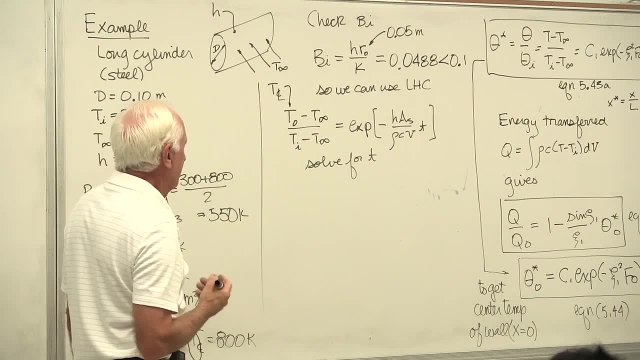 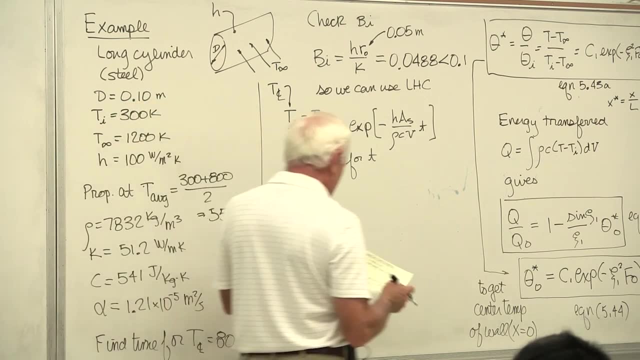 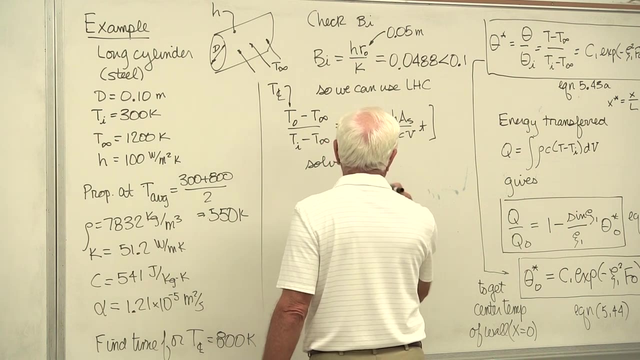 H surface area. pi R squared, pi T squared. pardon me, Rho, CVT, T, infinity, TI, T, center line. Put them all in there Straightforward, Solve for T and we get 560 seconds, Okay. 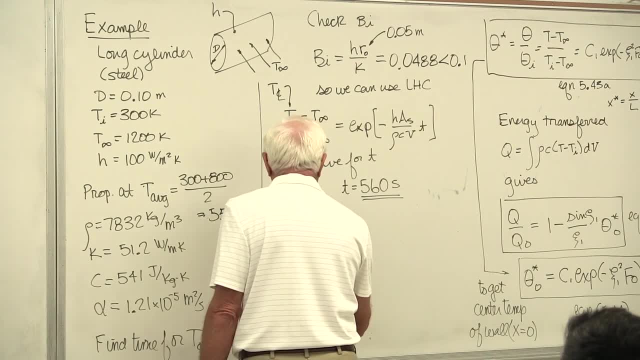 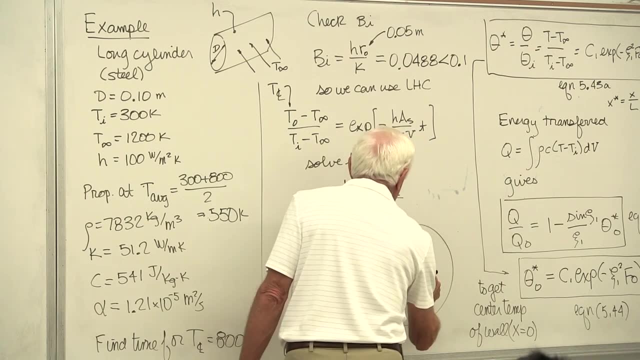 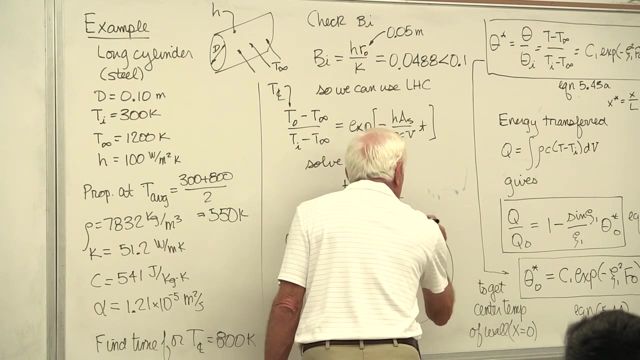 So if I look at that model at 560 seconds, the center temperature has reached 800.. The temperature on the outside surface is 800.. The temperature at any radius in the cylinder is 800.. That's what the lump heat capacity model predicts and says. 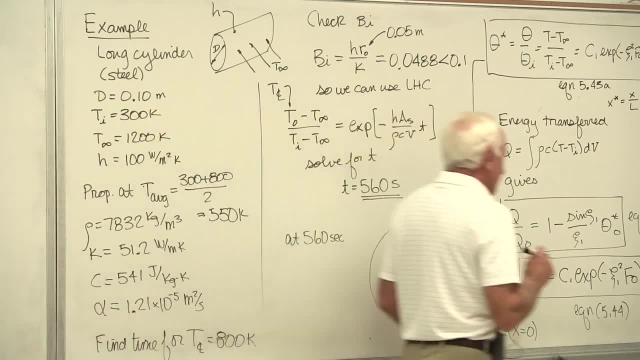 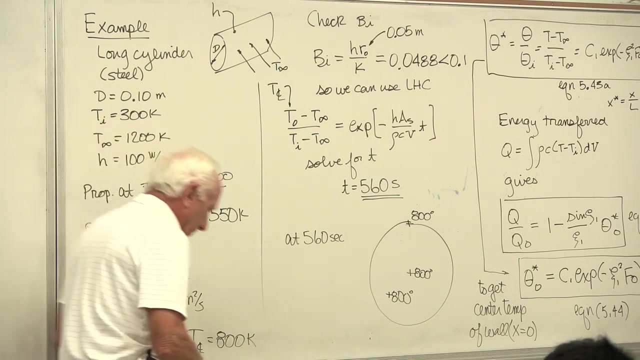 There's the picture All right. Now we're going to check that against the approximate solution. Okay, Remember, the approximate solution is an approximate solution to an infinite series, which is a solution of the governing partial differential equation. Is it valid for this BO number? 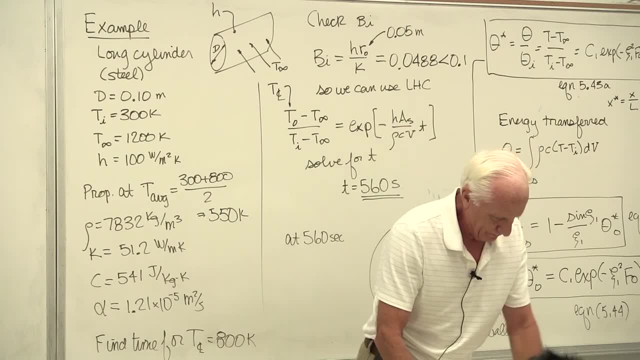 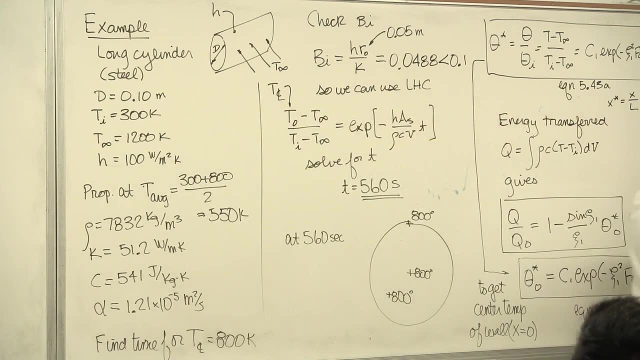 Well, of course it is. Of course it is. Why don't we just always use it then? Is this valid all the time? Because that thing is so simple. If you can use it, use it. It would be crazy not to. 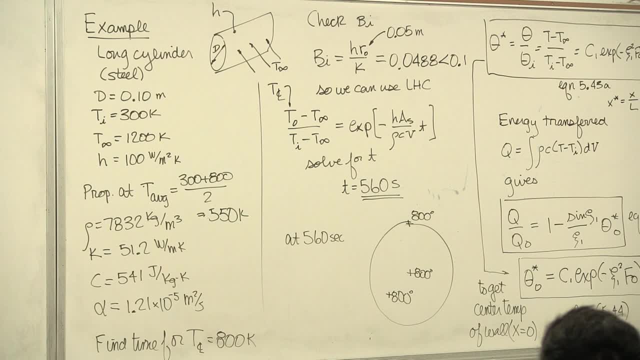 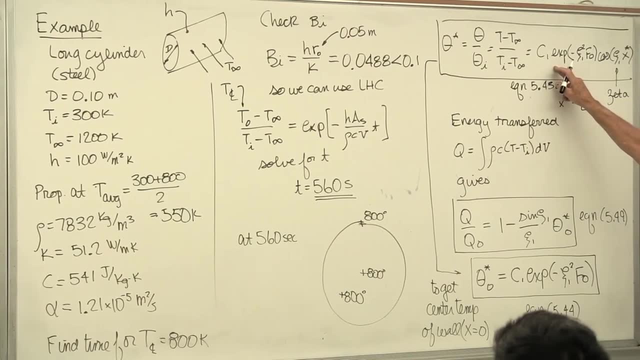 If you can use it, use it. There's a very small error using it. But if you want to get more complicated with the Fourier's and the Zay's and the C1's, yeah, this is valid any time. as long as what? again? 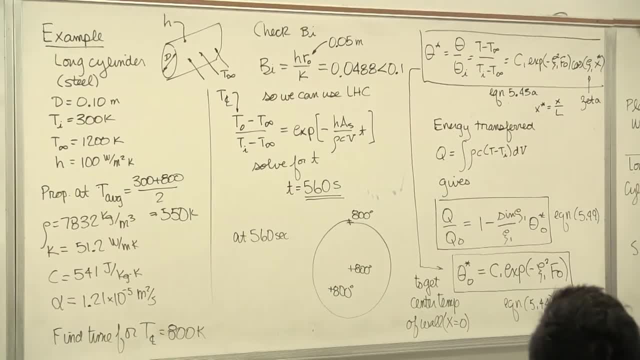 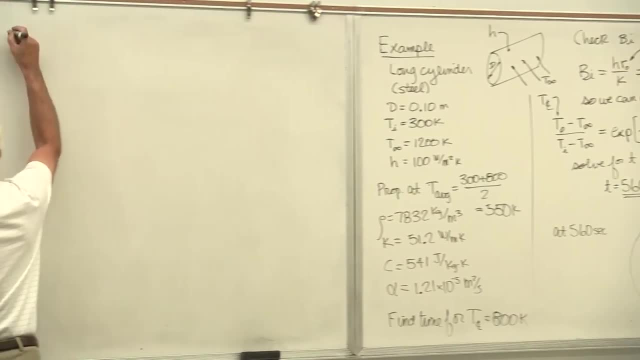 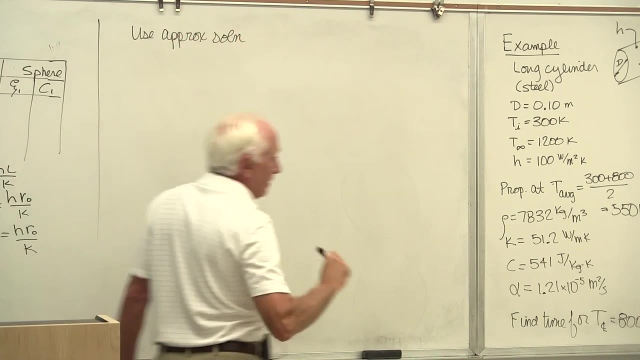 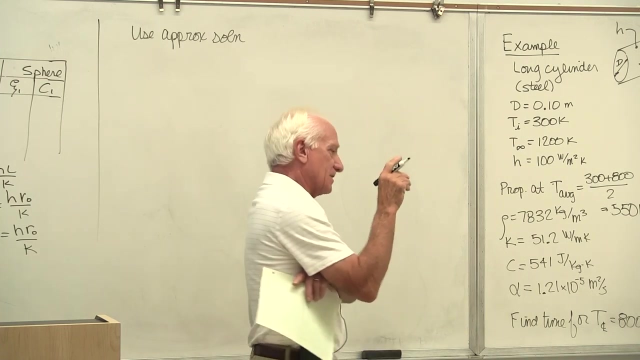 The Fourier is greater than 0.2.. Okay, So now we're going to use the approximate solution. Okay, The approximate solution. we start out. and To use the approximate solution, the Fourier has to be greater than 0.2. 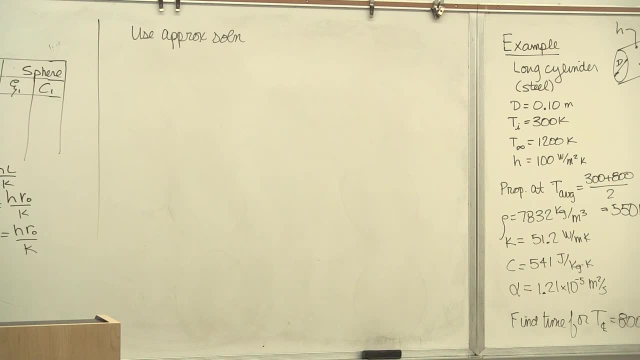 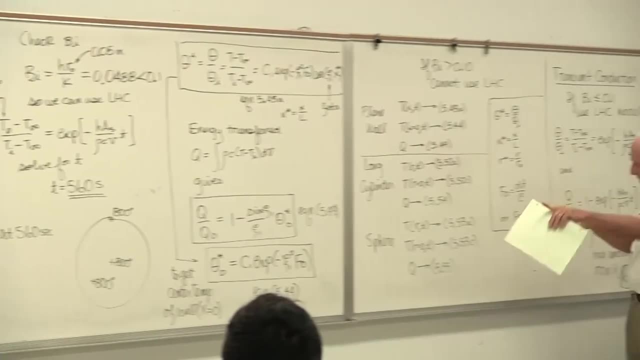 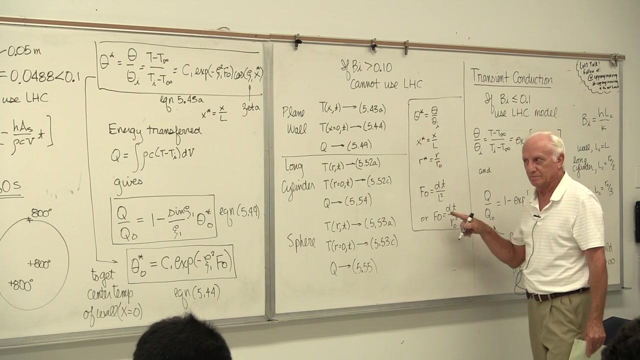 Here it is. So the first thing I do is calculate the Fourier number. Take alpha: There it is: Divide by the outside radius squared, We know, 5 centimeters Times the time. Uh-oh, I got a problem. 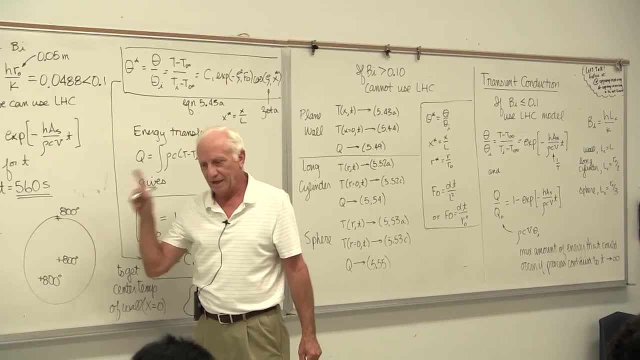 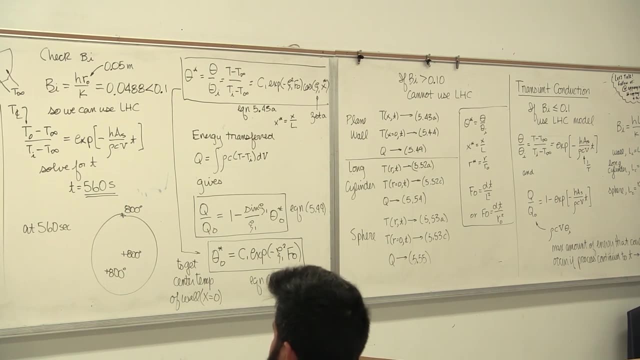 I don't know the time, So I can't find the Fourier number first. So what do I do? I assume it's going to be greater than 0.2. And when I'm done I can make sure it's greater than 0.2.. 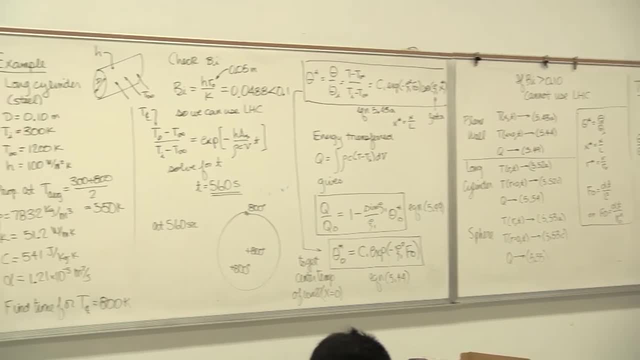 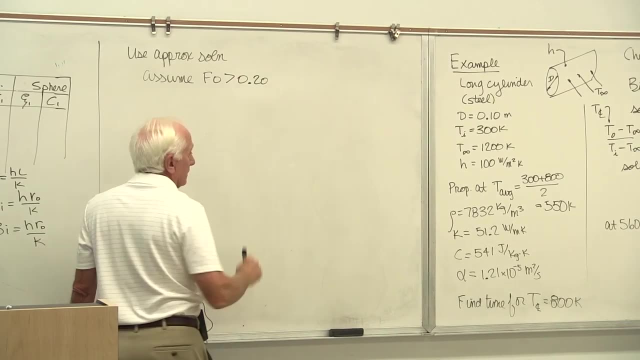 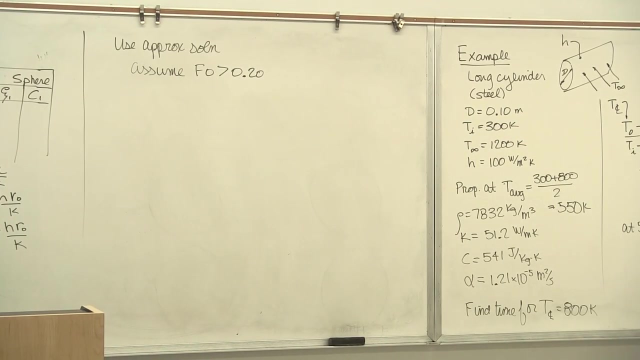 Okay, I assume it's greater than 0.2.. I can't calculate it right now. Okay, If I do assume that, here we are. This is chapter 5.. Everything you can use is on this side of the board. 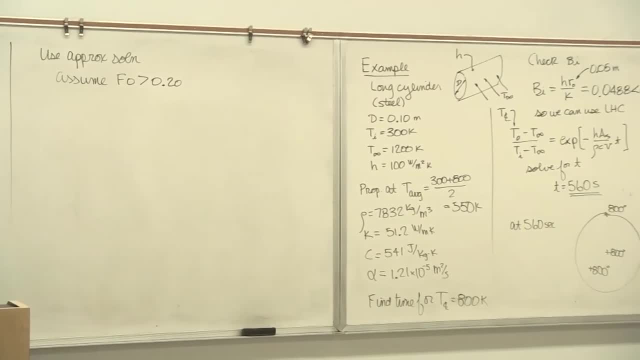 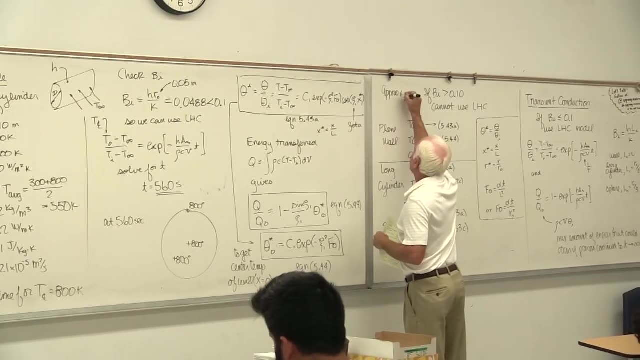 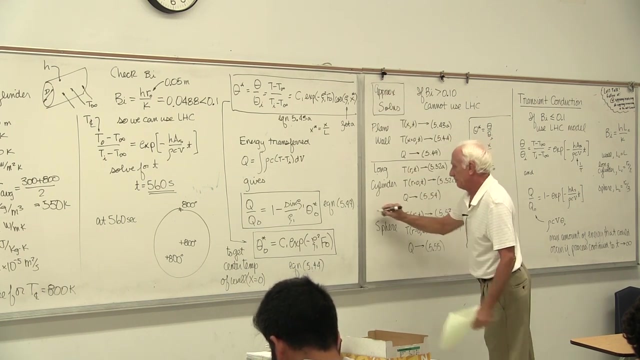 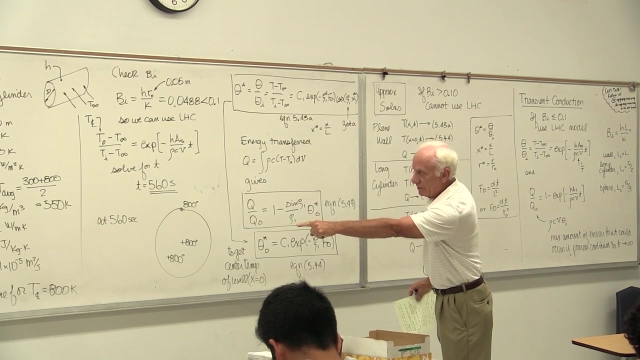 right here, Find it. I can't use that. I can't. This is the approximate solution. These are the approximate solutions. There it is. It's a long cylinder. It's a long cylinder. What do I want? I want the time for the center temperature: 800.. 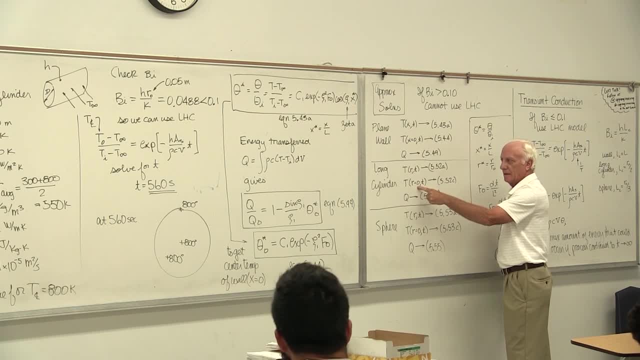 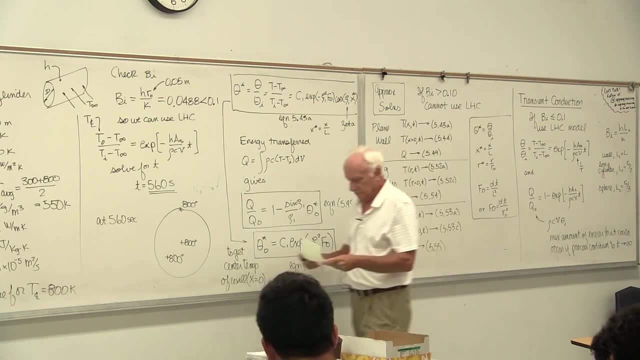 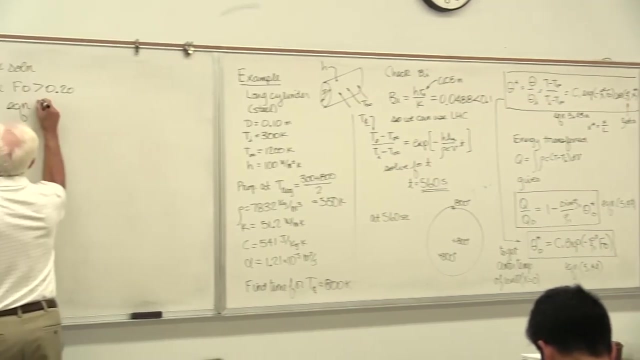 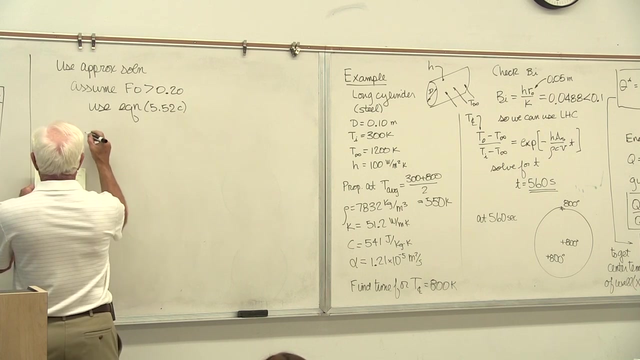 Center temperature, radius 0.. Oh, there, it is right there. That's the equation. I want Equation 552C Center temperature. There's time, Use 552C. Okay, So we use that And this is what we get. 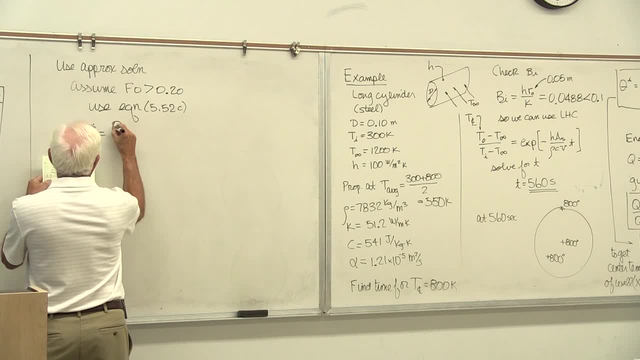 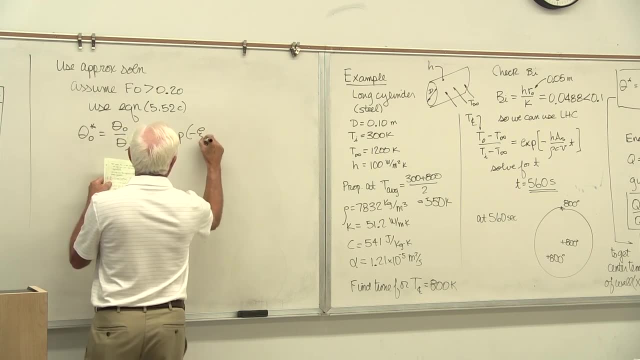 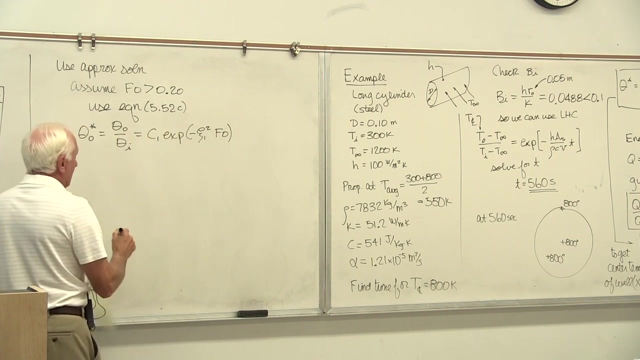 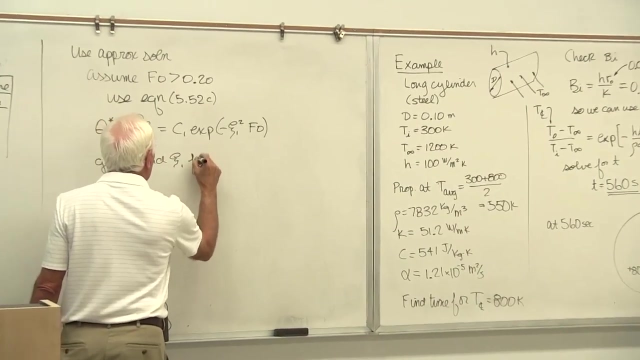 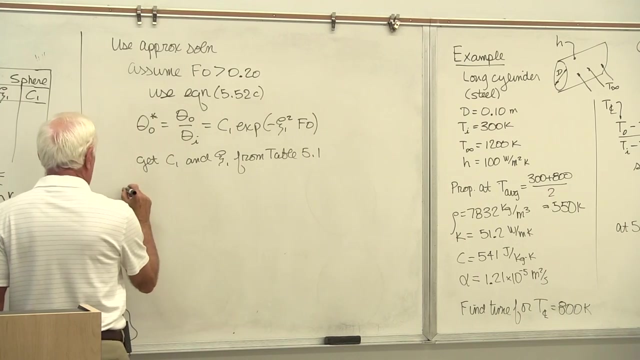 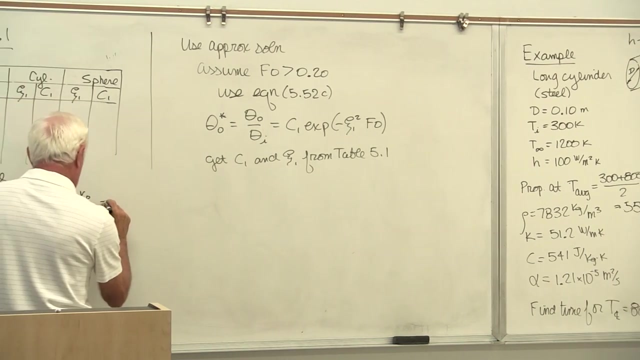 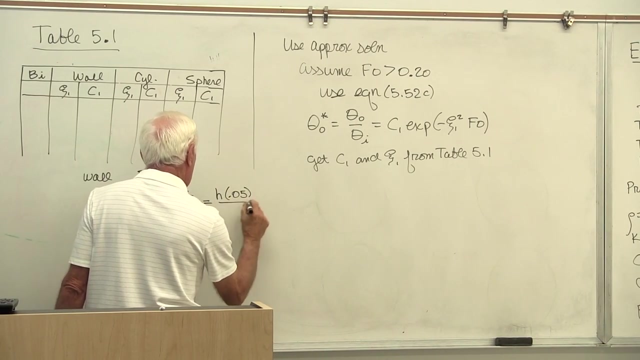 Beta naught star. Okay, Get C1 and Zeta 1 from Table 5-1.. Okay, BO, What is it A cylinder? Okay, Here, Cylinder Cylinder BO HR, not 5 centimeters over K, So the BO number .0976.. 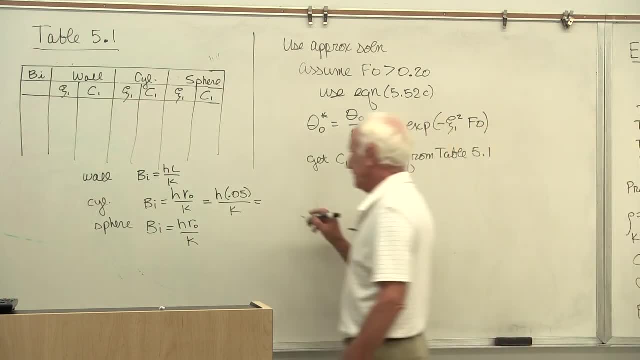 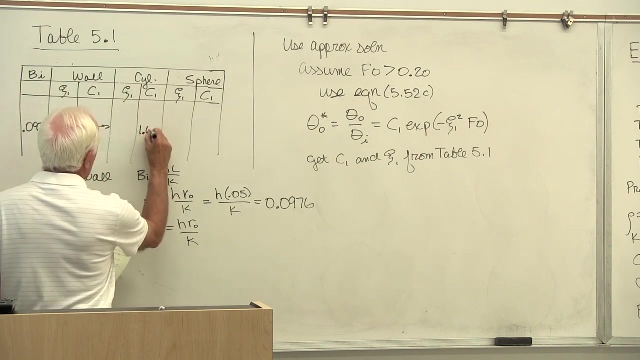 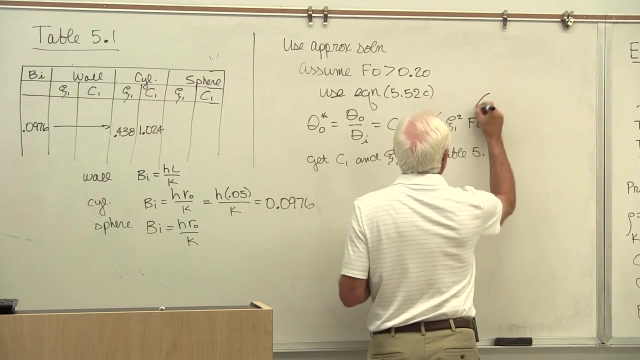 Okay, Go to Table 5-1.. Find the BO number No, Interpolate .0976.. Go to the cylinder right there, Get the value of C1, 1.024.. Interpolate: Get the value of Zeta 1, .438.. There it is right there. Put them in here. Remember the. 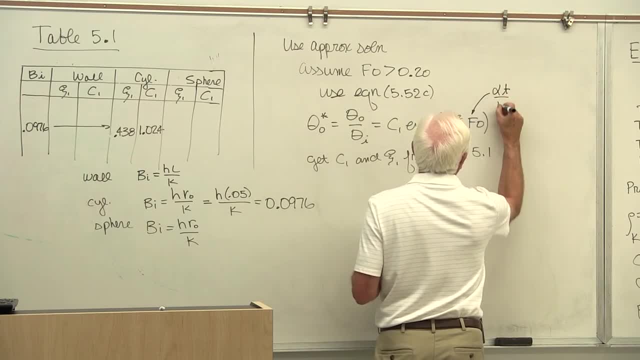 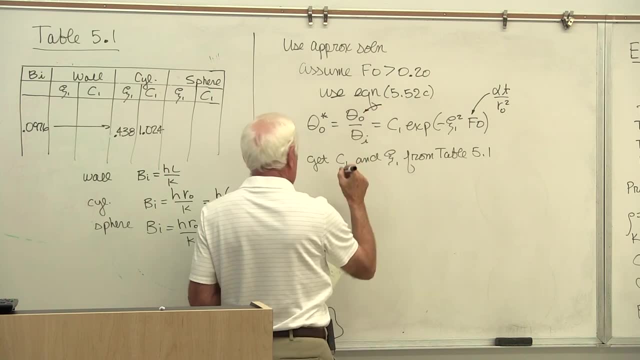 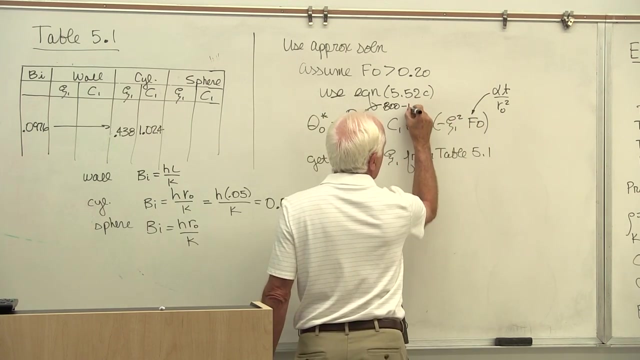 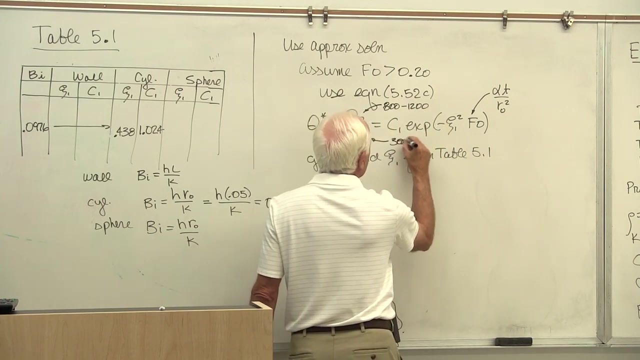 Fourier Alpha T over R0 squared. Remember what Theta T0 is: Center temperature: 800.. Free stream temperature: 1200.. Theta I: initial temperature: well, that was 300.. Minus 1200.. Put C1 in there. Put Zeta 1 in there. 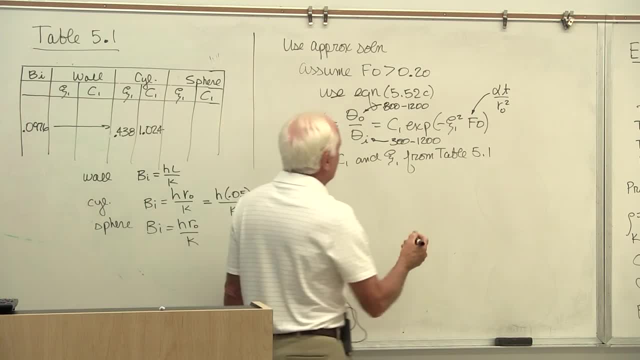 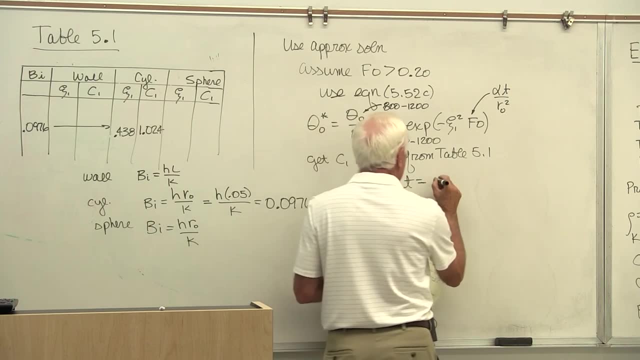 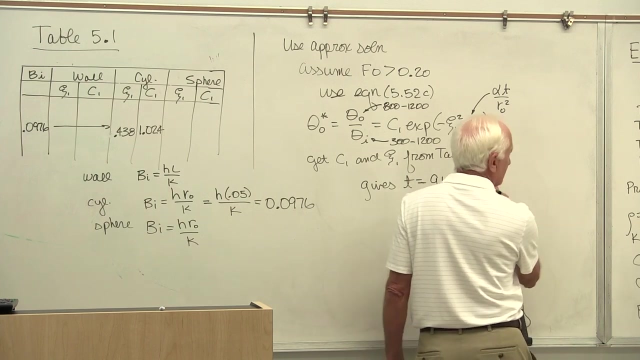 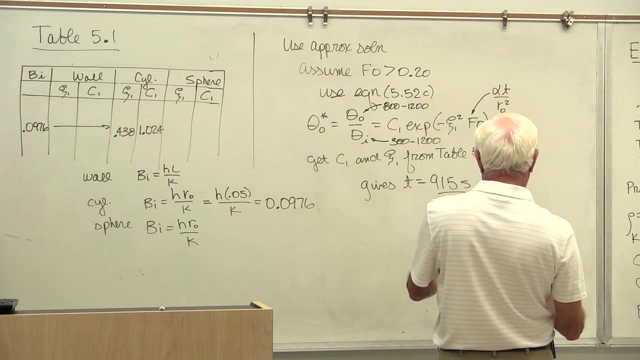 Take the natural log of both sides: Da da, da dah Solve for time Time: 915 seconds. Okay, They are going to be a little different. That guy was 560 over there. Oh, not 560.. 560.. Let's see here, 560.. We didn't get that guy, I wonder. 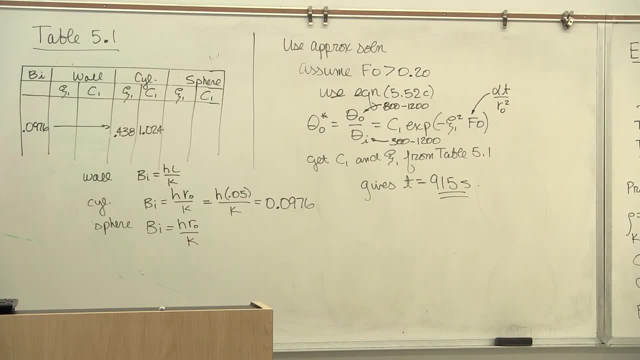 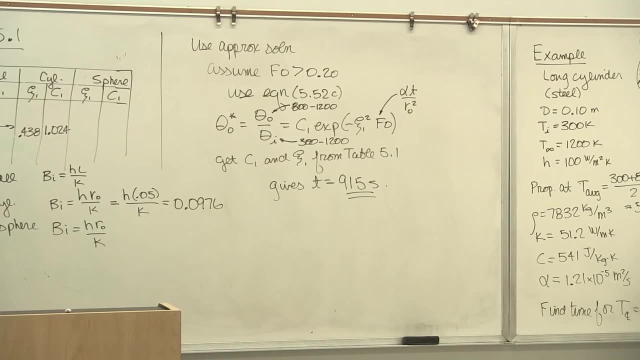 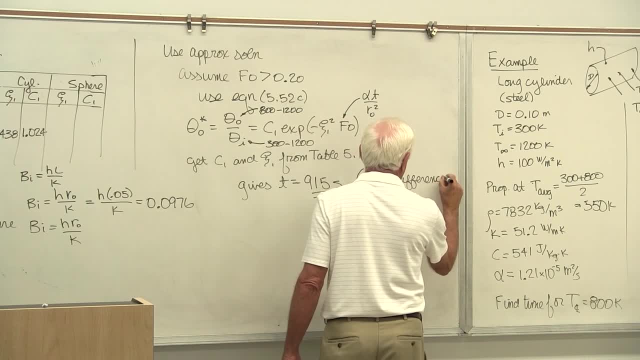 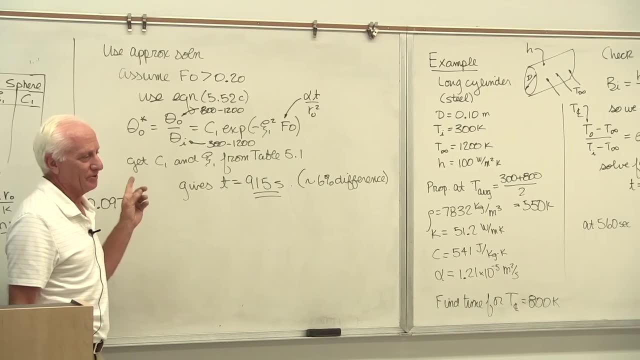 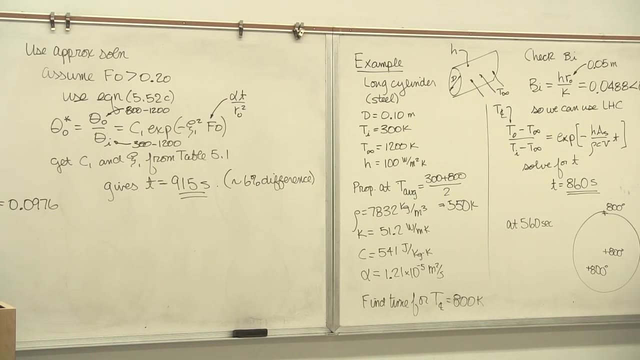 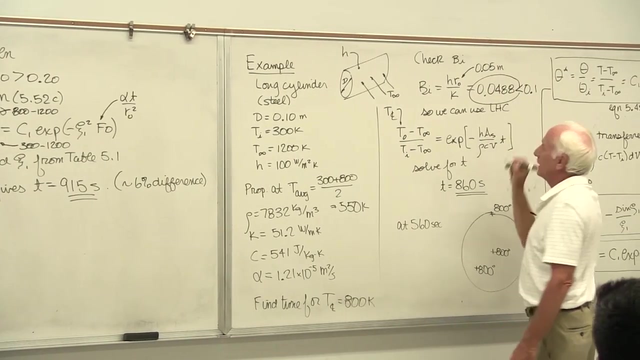 difference. which one's a better estimate? oh, probably this guy. he comes from the solution, the governing partial difference equation. this guy's an approximate one, which gets you a pretty good number. if you assume that model, you better be really, really careful, because there's what I used. 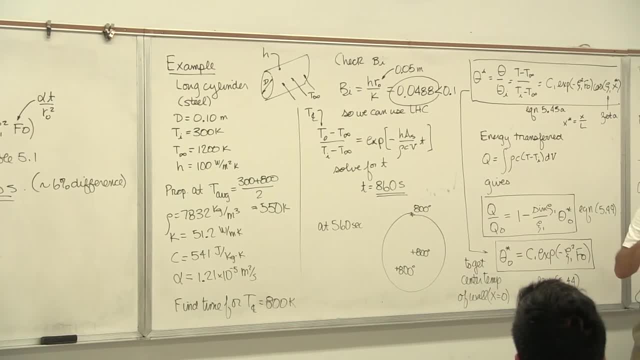 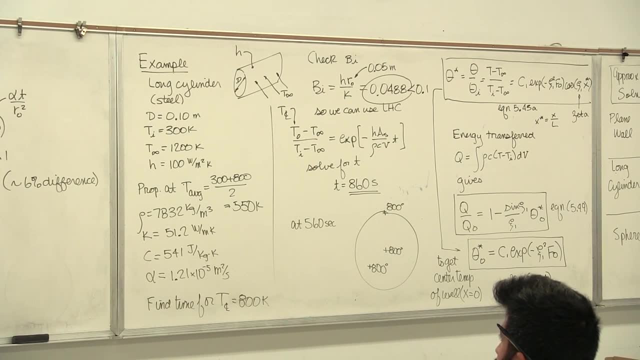 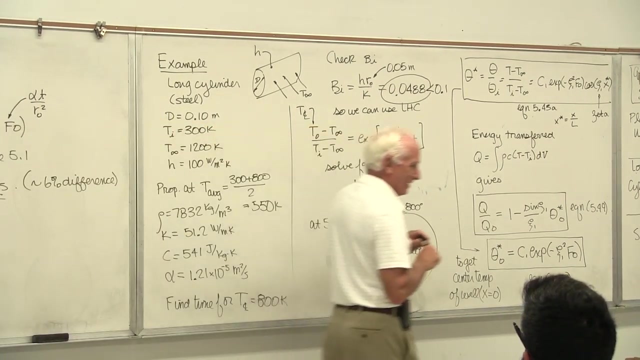 to find out if I could use lumped heat capacity Bionumber. here's what I used. if I go to table 5-1, they both say Bionumber. why are there two Bionumbers? because the guy that wrote table 5-1. 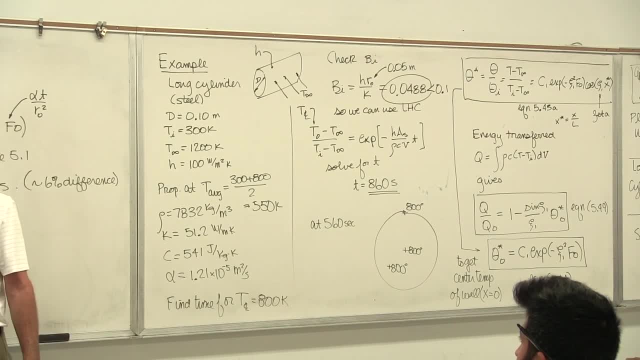 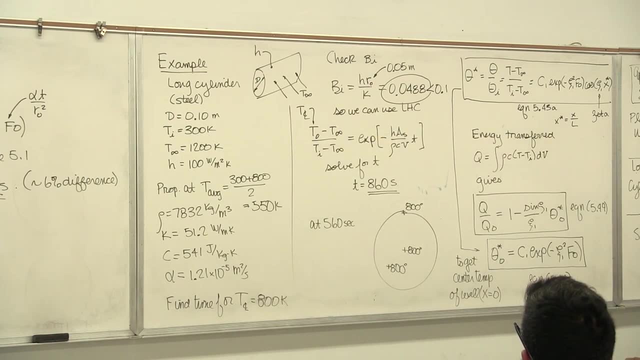 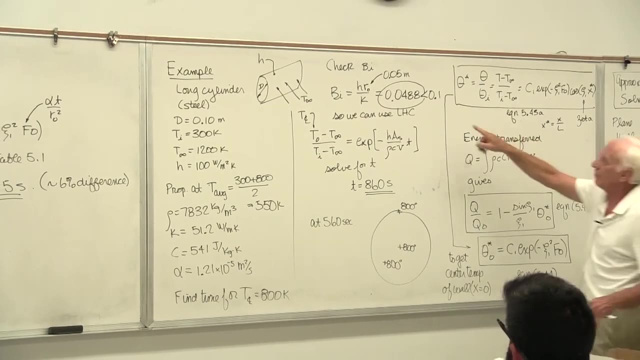 said: if you want to use my table, this is how you define the Bionumber. I play cards. I'm the boss of the table I'm dealing. that table came from him. he can call Bionumber whatever he wants. why, why wouldn't he call this? 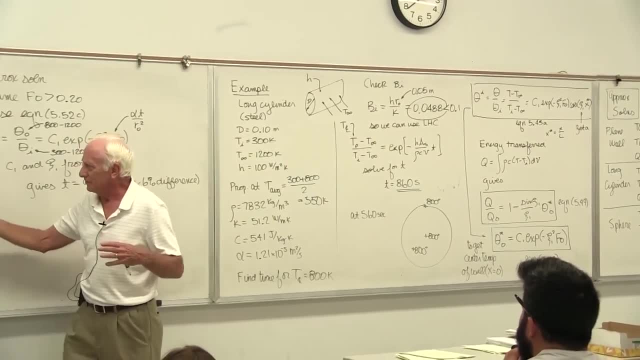 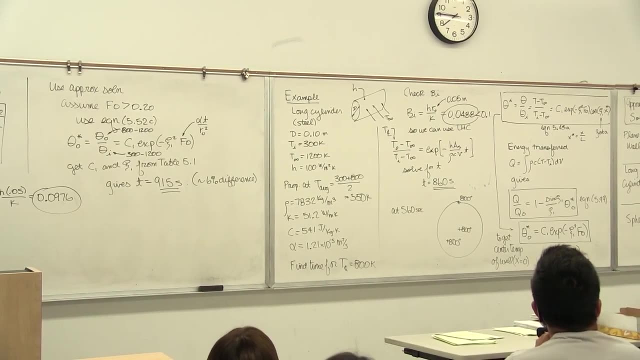 well, this way you don't forget things. it's a cylinder or sphere, it's just a radius over here. you got to remember. let's see: if it's a cylinder, it's the radius squared- I have to pardon me, it's half the radius. if it's a sphere, 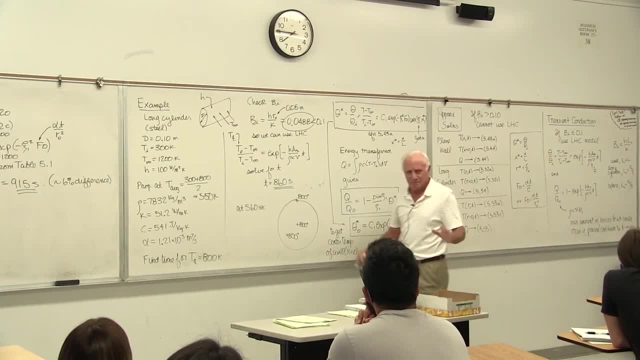 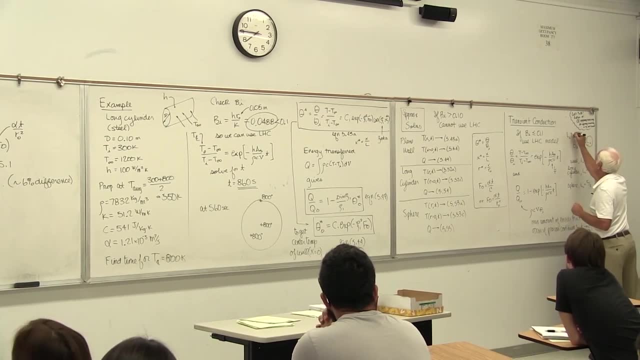 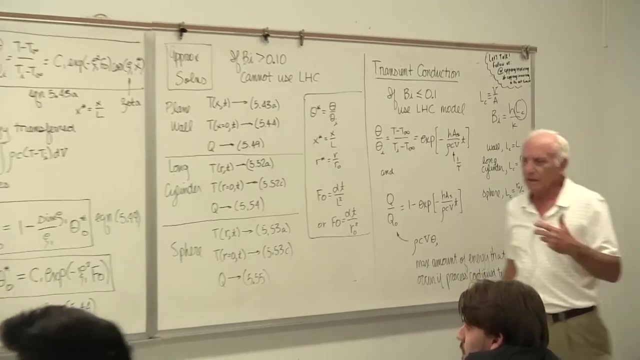 it's a third the radius. why make life difficult? well, that's because this is how the Bionumber is really defined, defined, And that LC is defined as a volume over the area. This is the right, correct way to do it. But to make life easy, this guy said, I'm just going to put an R naught. 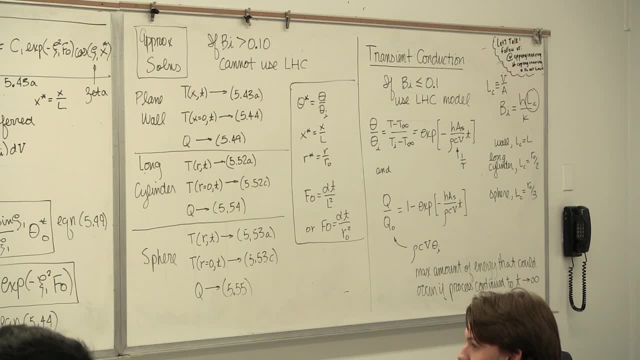 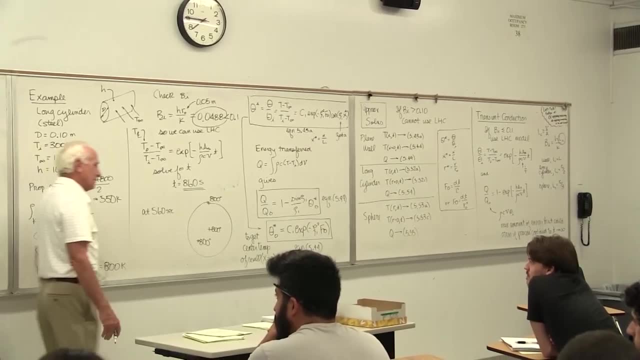 for both these guys, so you don't have to worry about is it divided by two or divided by three, and use my table And you get the right one. It's his call. He's in charge. He wrote the table. He can do what he wants. If I want to use it, I have to do what he told me to. 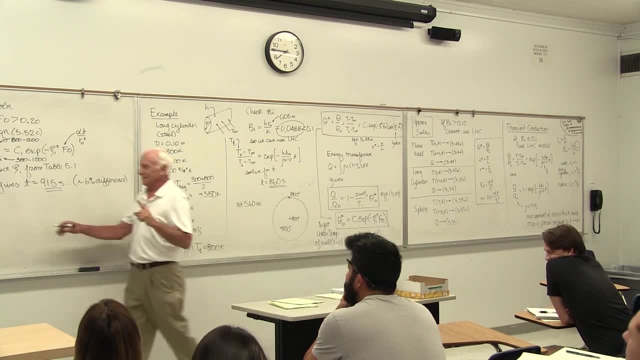 do? He says: if you want to use my table, there's a new VO number, which is this one. Isn't it like the old one? But does that bother you? I say well, kind of. Well, it's okay. 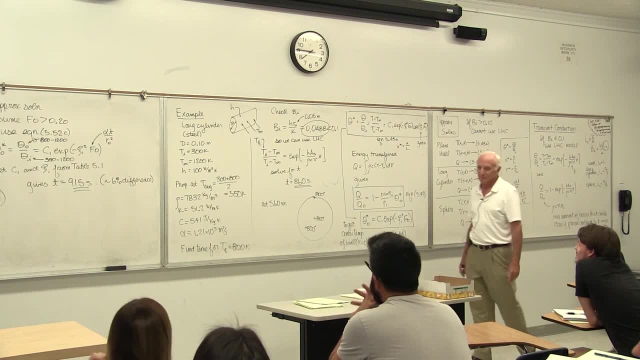 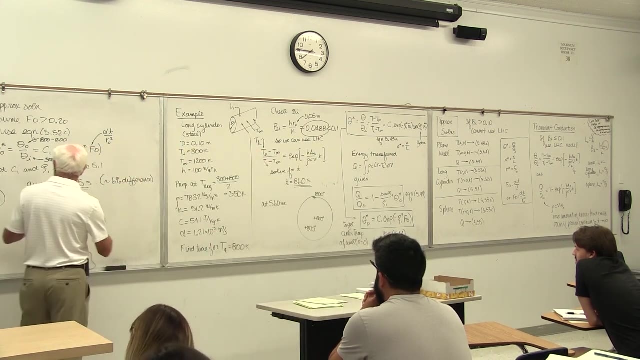 You'll get used to it. And so the R naught for the first VO number should be .025.. That's right, That's right, That's right. Yeah, Uh-huh, Uh-huh, All right. Yeah, that's right. Now let's say part B of the problem says: at this time next: 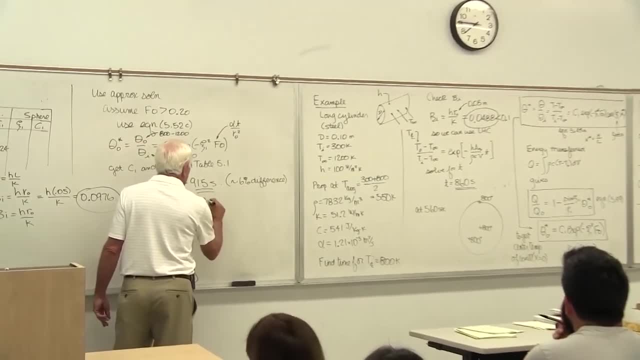 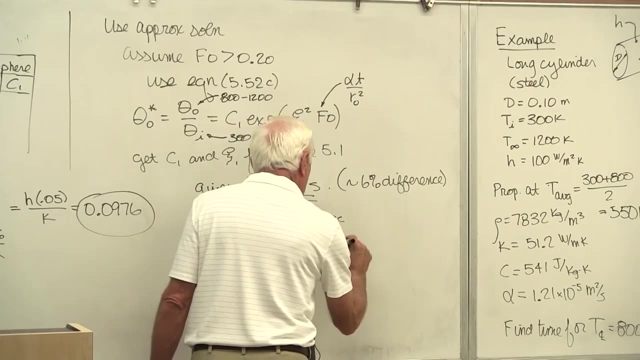 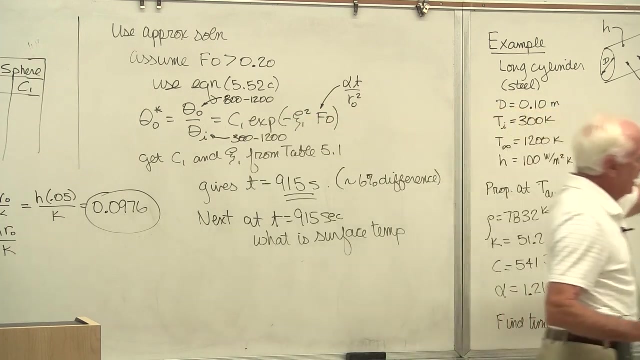 At t equal to 915 seconds. what is the surface temperature? Okay, There's chapter five. Go back there again. What do I have? I have a long cylinder. The VO is not less than one-tenth. Where do I go? 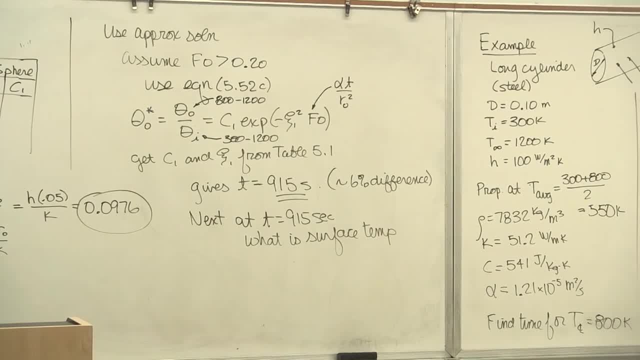 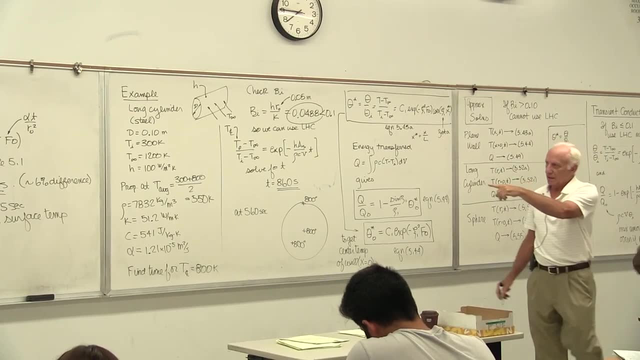 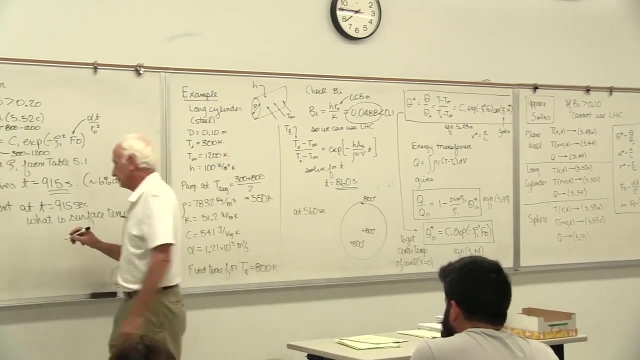 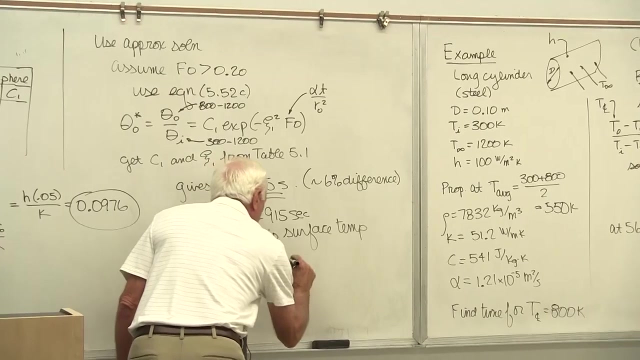 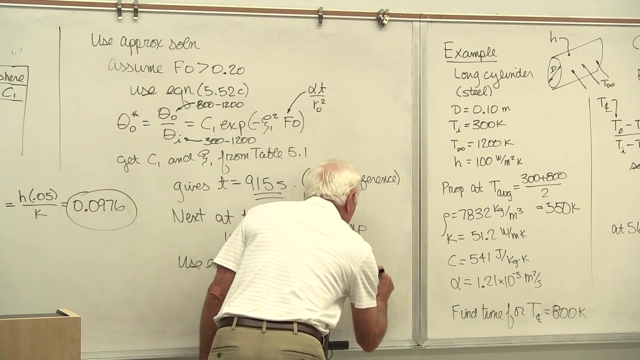 A long cylinder. What do I want to find Here? it is The temperature when the radius is outside and the time is 915 seconds. What equation? 552a With R star? there'll be an R star in there. R over R naught, that is one. 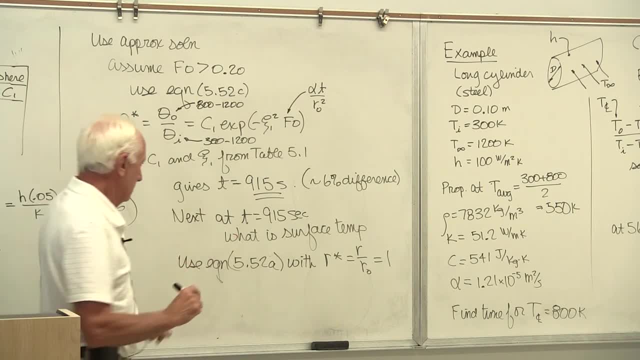 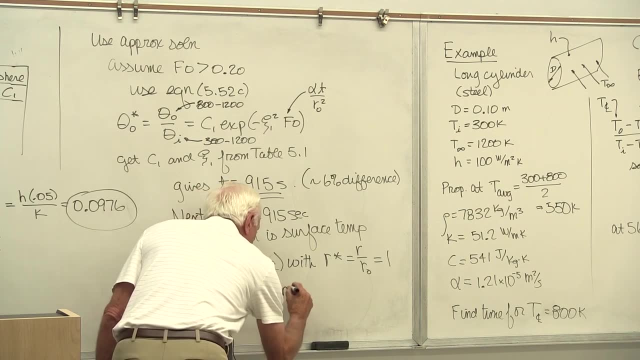 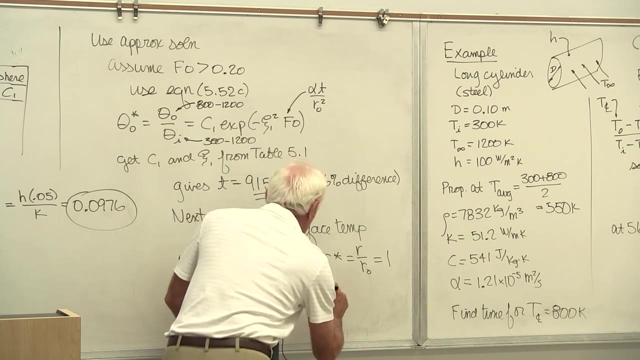 Wherever you see an R star in that equation, put one. Solve for temperature at R equal R, star at R equal R outside. Pardon me, And time equal 915 seconds, And if you do that you will get the surface temperature of 819 degrees K. 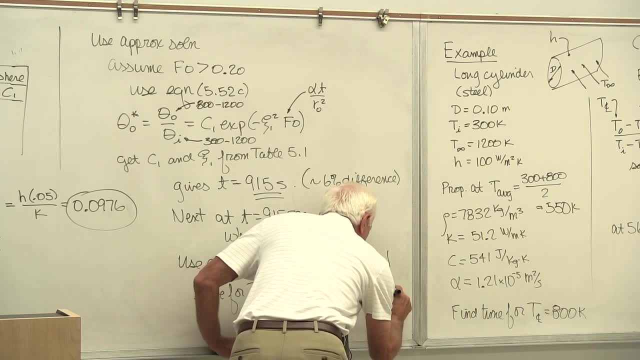 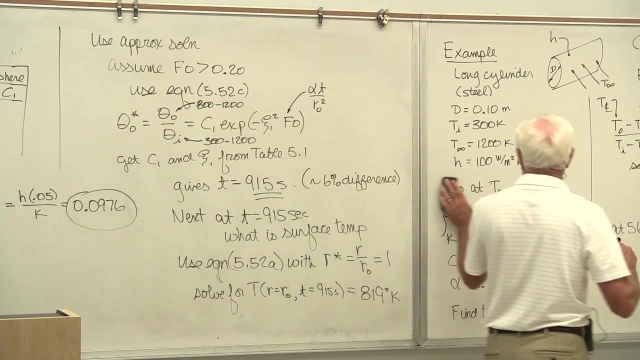 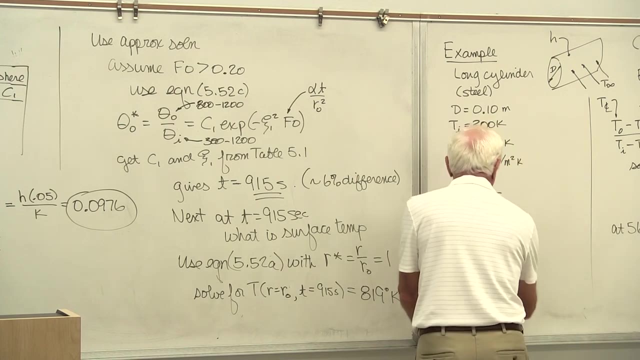 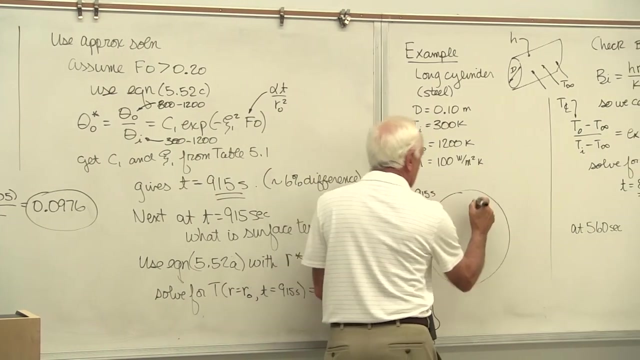 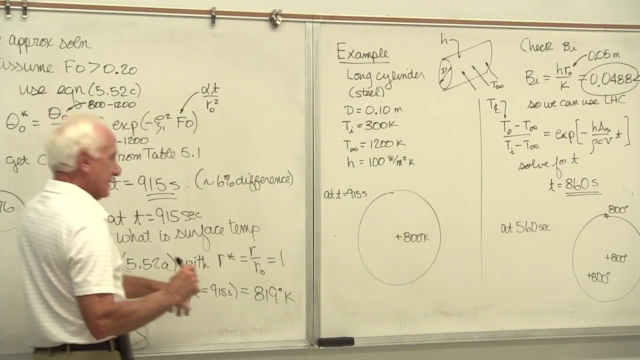 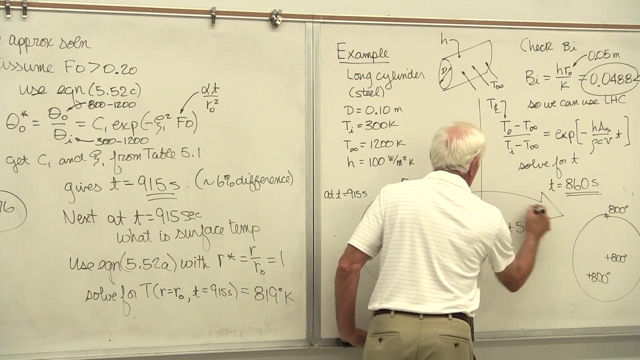 Okay, So here's the picture, for that, At time equal 915 seconds, the center of the sphere has reached 800 degree K, But the surface now is at 819.. And you can compare the two to see the difference. When we use these approximate equations, the temperature depends. 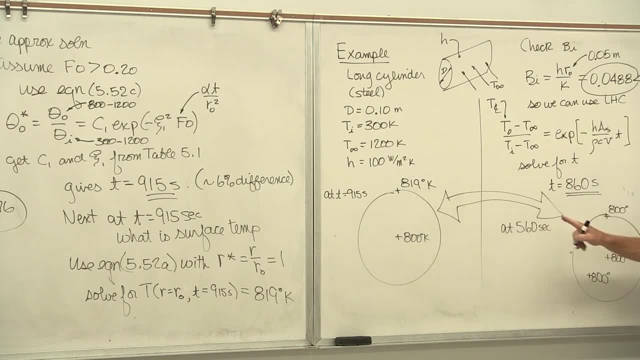 on not just the time but the radius. When you use lump heat capacity, the temperature does not depend on radius, only on time. Okay, so we've worked them both ways now. Oh, by the way, some people and some textbooks also use a. 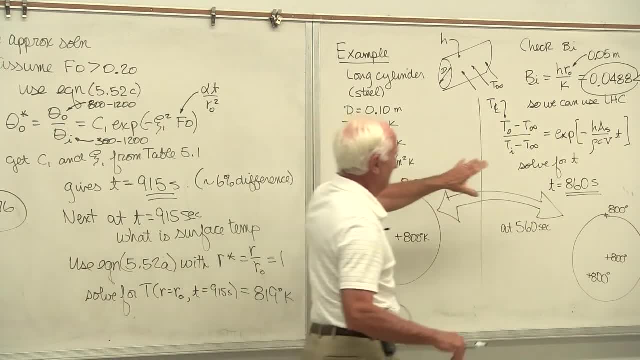 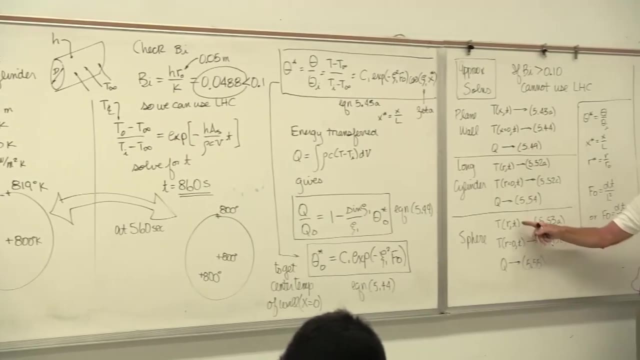 graphical approach, Rather than use these equations, these nine equations. here. they give you a series of six graphs: Two graphs for this, one for temperature, one for Q. Two graphs for this, one for temperature, one for Q. Two graphs for this, one for temperature, one for Q. 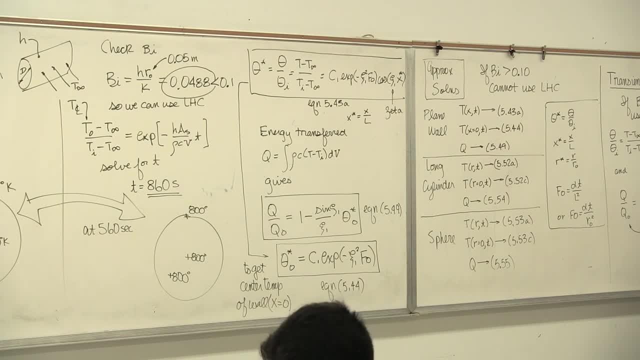 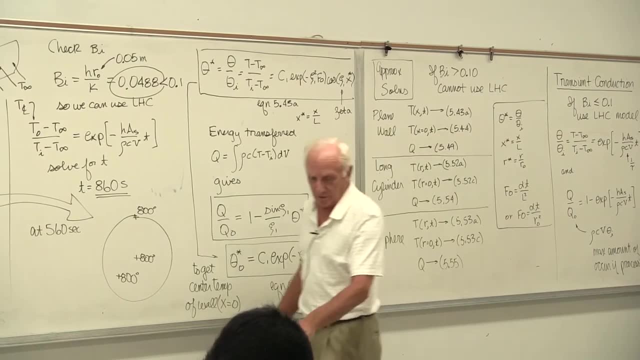 And you can read the graphs not too accurately. There's so many lines on this it's very, very hard to read accurately, But they are available. They used to be in our textbook. The author pulled them out and put them online now. 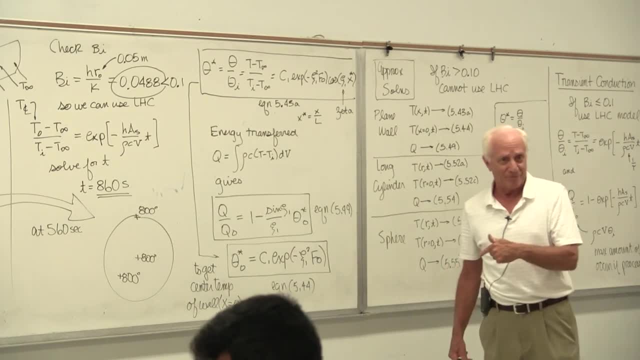 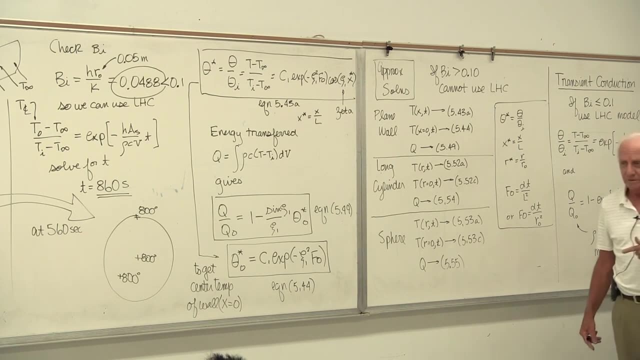 because he doesn't use them anymore in the textbook. It's hard to program graphs. You can't do it. Try and program the weight chart. You don't do that. You get curve for the equations, for all the friction factors. So it's probably better to look at the equations. 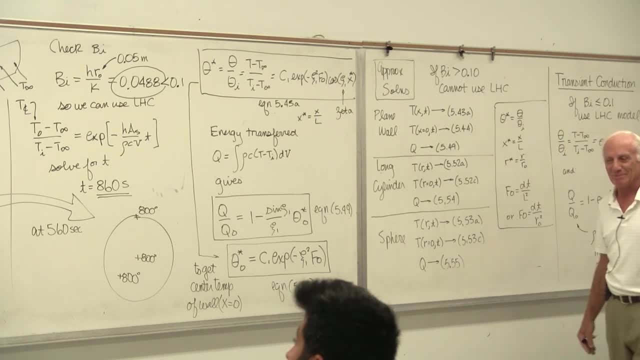 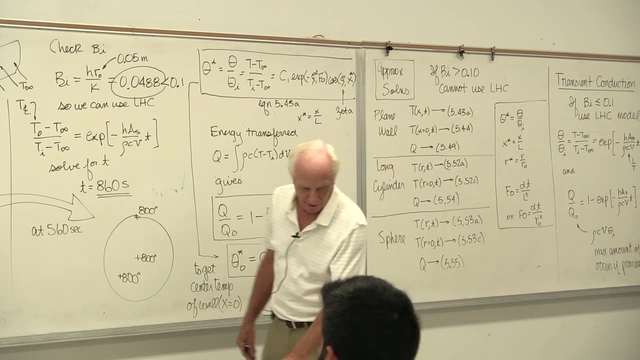 They're fairly straightforward, you know. They can be programmed where the they're called the Heisler charts. Heisler charts transient conduction problems, And you can do all these things. Okay, I think that's got it. 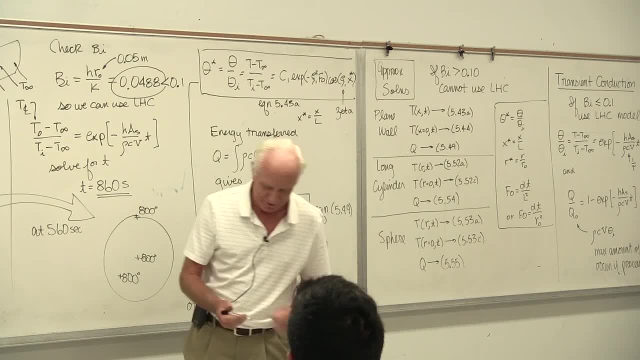 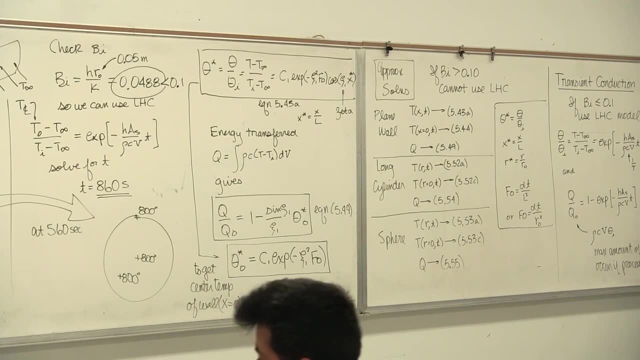 So that ends Chapter 5.. We're going to start Chapter 6,, ah, Chapter 12, Radiation, on Monday. Okay, So next week we start. 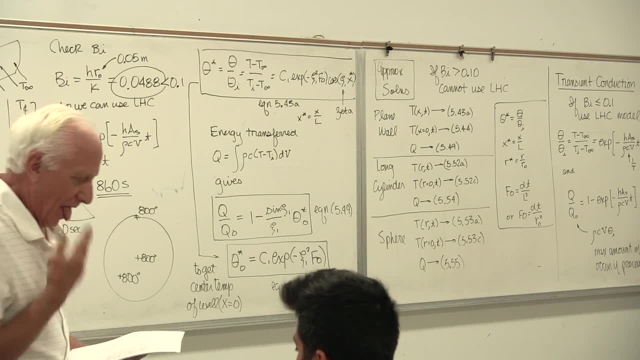 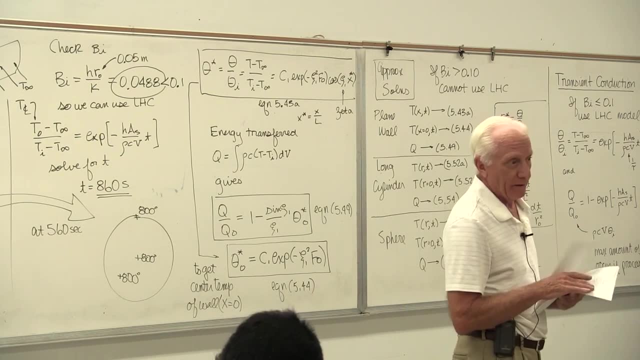 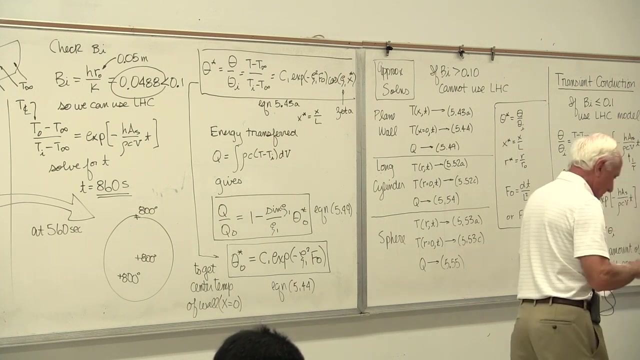 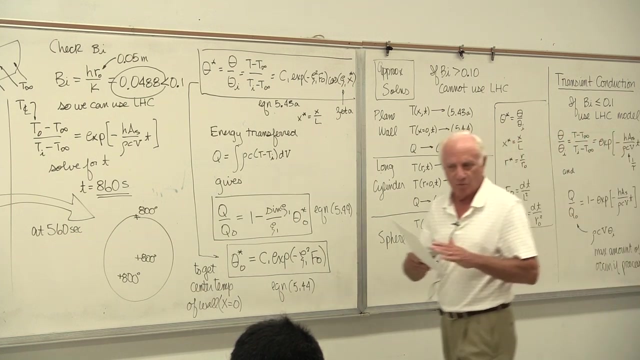 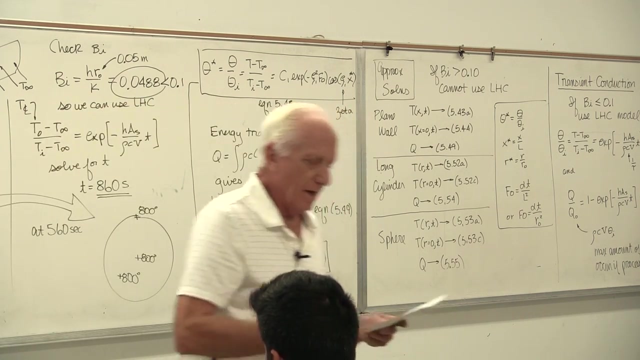 You can work clubbing forward two ways. One way- I worked it here using table 3-4- or you can use table 3-5, which is the fin efficiency. 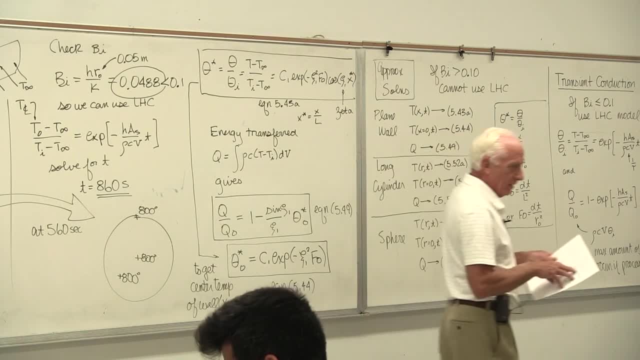 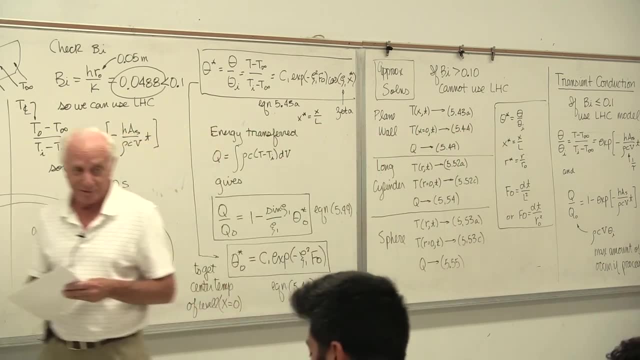 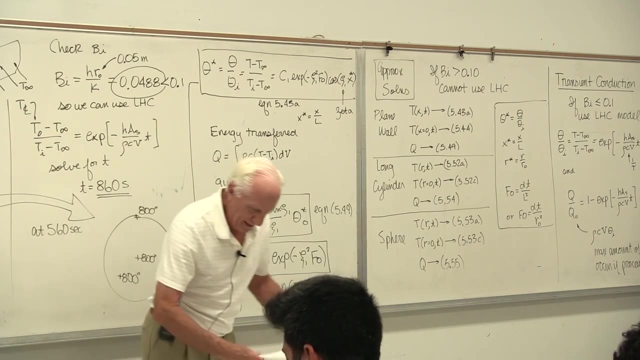 So either way, use table 3-4, like I did here for part A, or use table 3-5 for part A. For part B, you've got to use table 3-4 for part B, the temperature, Okay. so if you can look over that and see how you did compared to that, 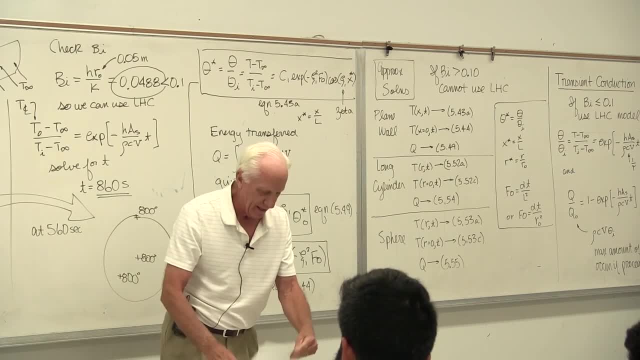 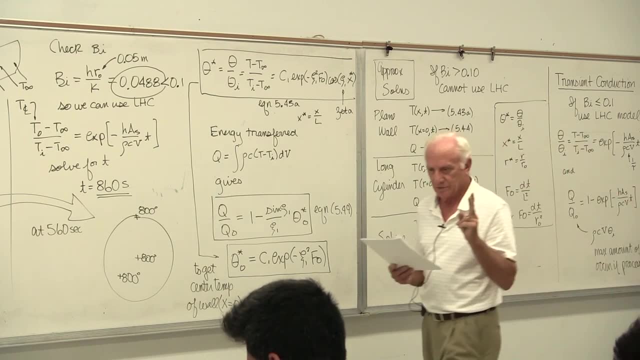 The average is pretty decent: 78 and a half, 78 and a half. the high was 1-100,, 2 at 90,, 8 and a half. So the three highs: 1-100,, 2 at 90,, 8 and a half. 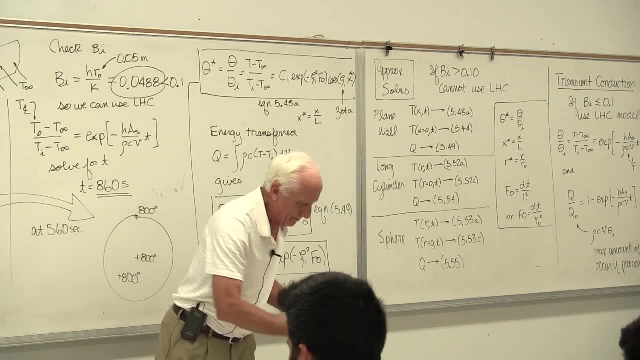 When we get these back to you. we're done for today. We'll see you on Monday. let's see about section one. 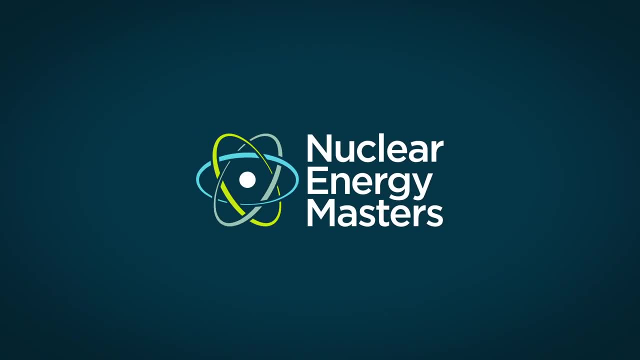 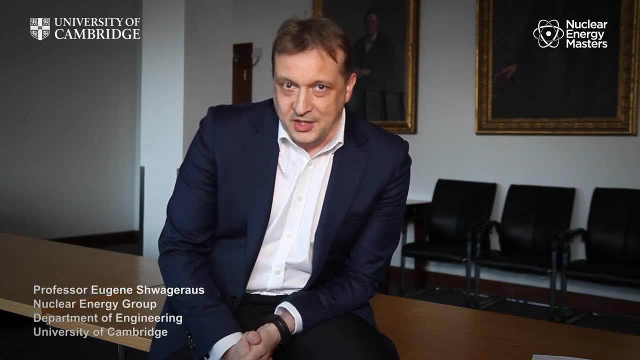 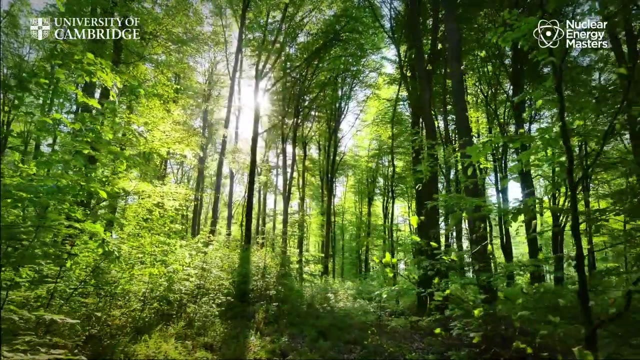 Nuclear science and technology improves many aspects of our everyday life. Nuclear energy is one of the least polluting energy sources we know. It's available whenever we want it on demand, regardless of season, weather or geopolitics. It can propel ships or even spacecrafts. 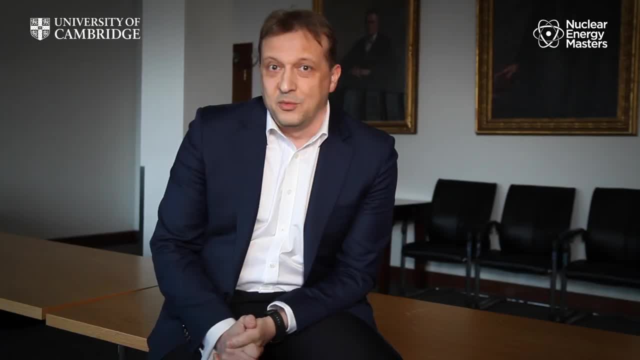 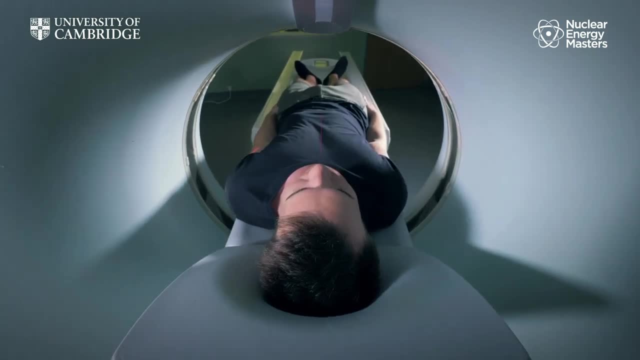 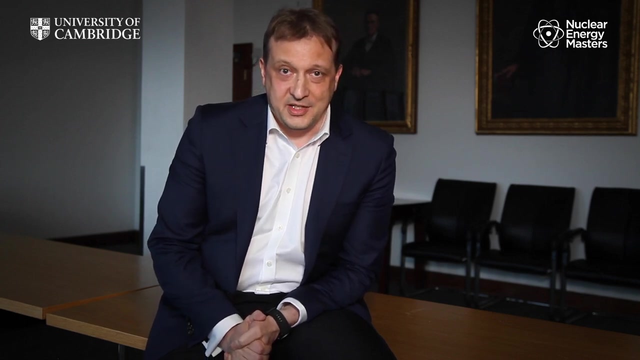 It can heat our houses and power many industrial processes. We will need all of those things to decarbonise the world economy. Nuclear technology is also saving lives by allowing early diagnostic of diseases and their treatment. A long-anticipated renaissance of nuclear energy is happening as we speak in the UK and around the globe. It will require a massive